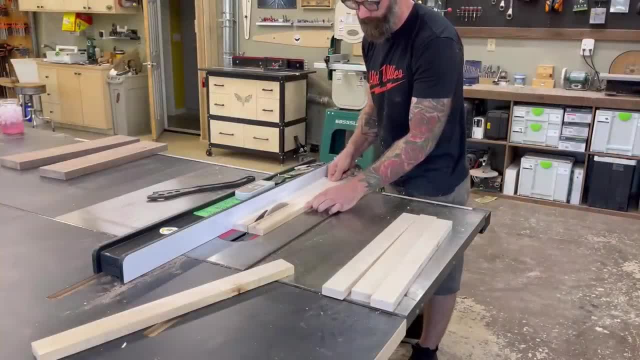 I'm going to need two contrasting woods For my chessboard. I'm going to need two contrasting woods For my chessboard. I'm going to need two contrasting woods For my chessboard. I'm using black walnut and this hard maple. Next, you're going to cut down strips of wood Now, whatever. 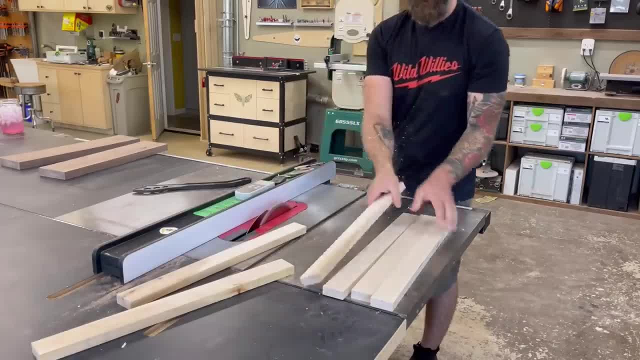 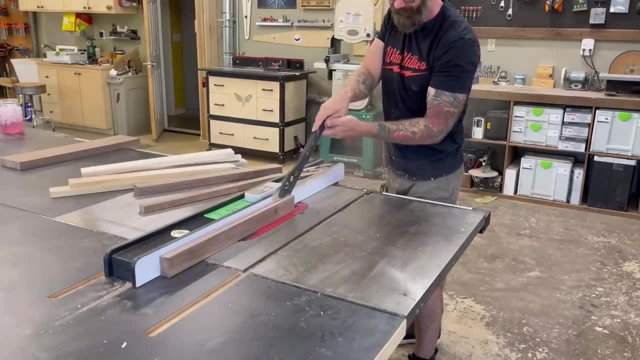 width you cut these strips to. that's going to be the width of your individual squares. You're going to need four of each color, because there's eight rows in total on a chessboard. So I cut down four of the maple And then, because I was using thicker walnut, I cut that down and then 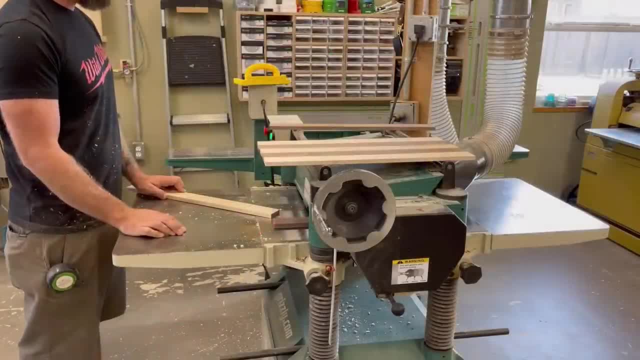 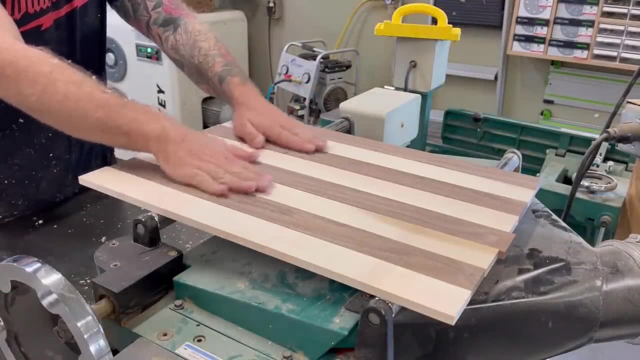 I cut each one of those pieces in half so I could get more out of it. Then I took all my walnut strips and my maple strips and I planed them all down until they were a uniform thickness- Eight strips in total. Then I glued all of my strips together, making a nice 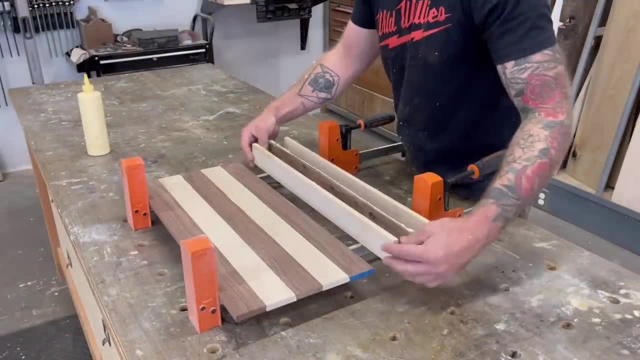 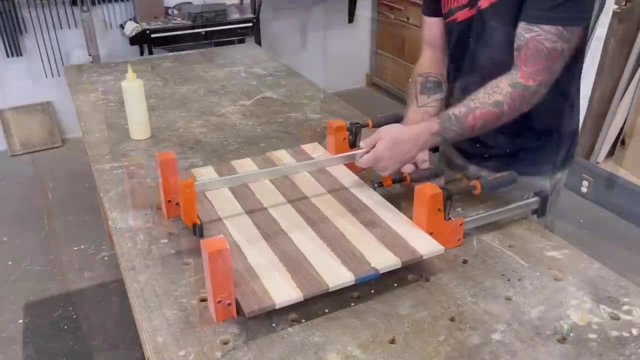 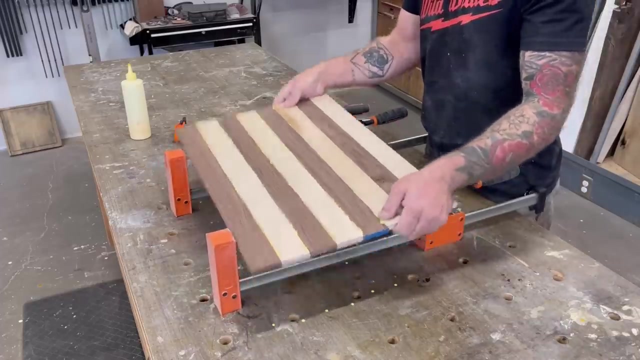 pinstripe motif, Just making sure there was enough glue in between each seam so that everything sandwiched together and had proper squeeze out and would glue up in one solid chunk. Once my glue was dry, I took my beautiful maple and walnut pinstripes out of clamps and next I 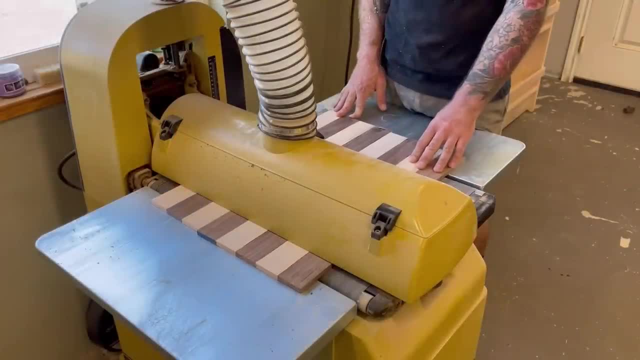 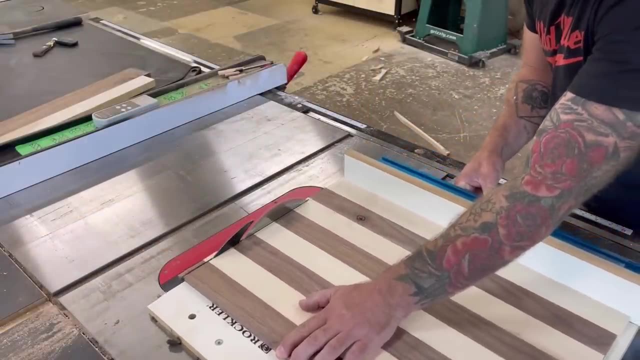 ran the entire thing through my drum sander on both sides just to make it nice and smooth. Then I took it over to my table saw and using my Rockler crosscut sled. This is such an easy sled to use. I'm really happy with this Rockler sled. 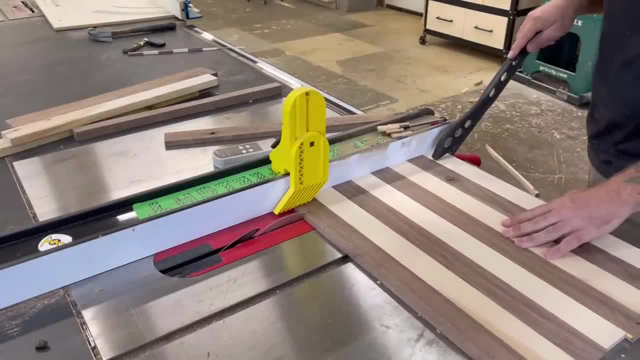 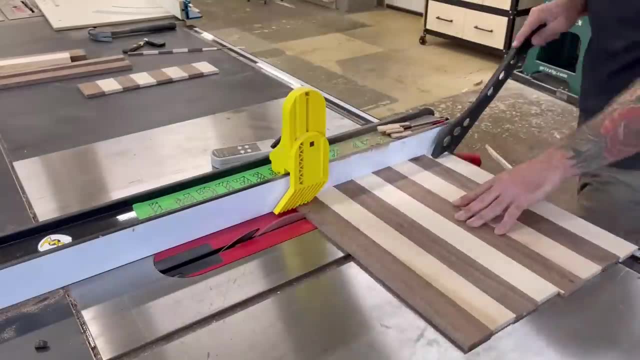 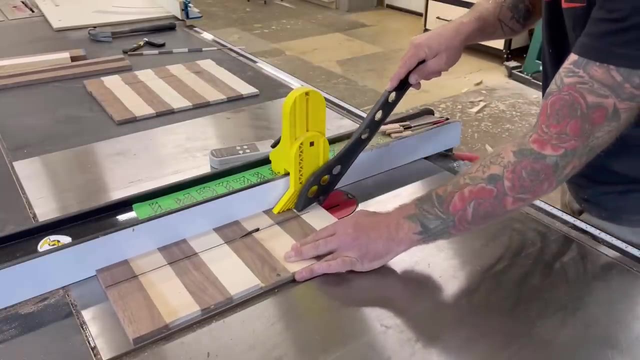 I trimmed down one side so I had a nice square edge. Then, using that square edge, I set my table saw to the exact width as my individual strips, which was two inches, And I sliced my maple and walnut pinstripes into eight individual strips, alternating in color. Now I know, I know chessboards. 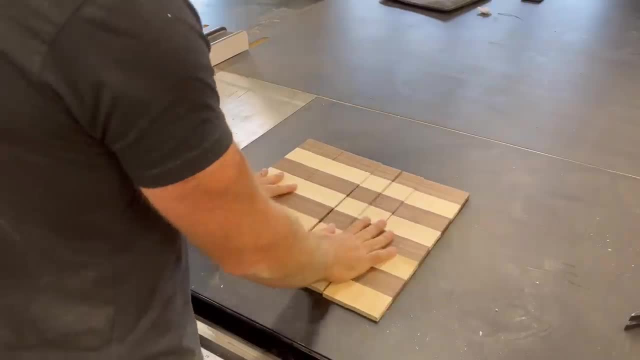 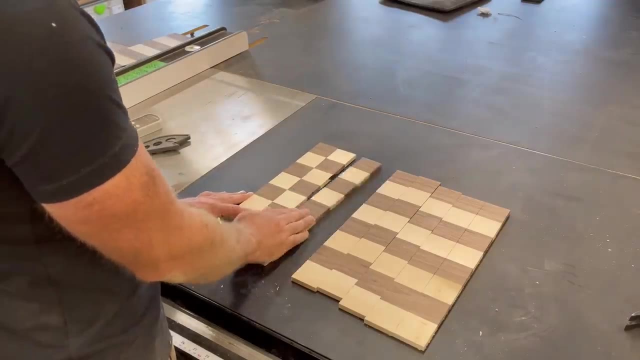 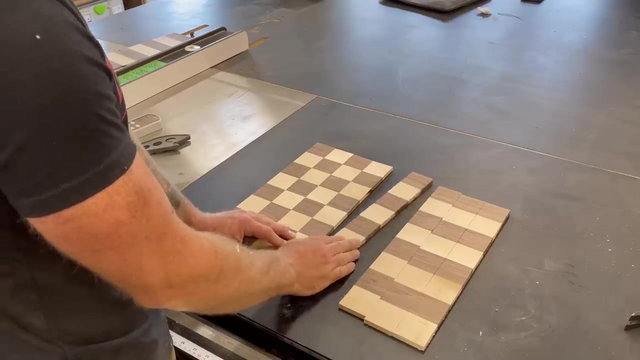 aren't striped, They are more of a checkered pattern. Well, once you get all your strips cut down like this, you turn every other strip around the other way and it turns it into a chessboard pattern slash checkerboard pattern. You could use this board to play either The prerogative, 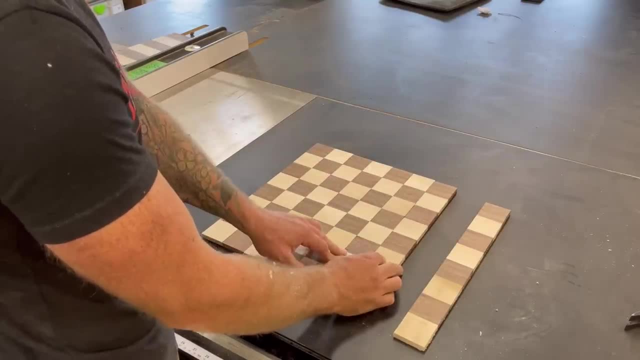 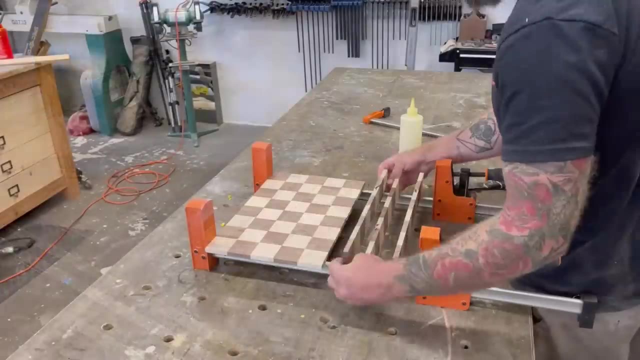 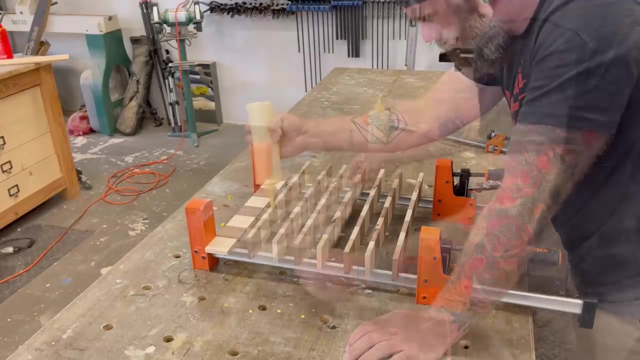 is yours, Anyways. you alternate every single piece and now, instead of stripes, you have a beautiful checkered pattern of which to glue up your chessboard and or checkerboard. So, after gluing this whole thing up and cutting it apart, yeah, we're going to glue it back together, but this time in the right pattern And you want to. 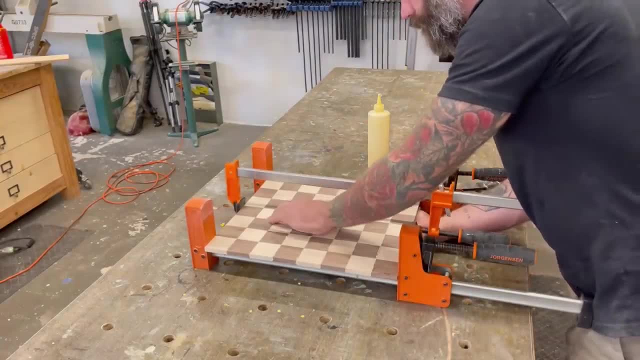 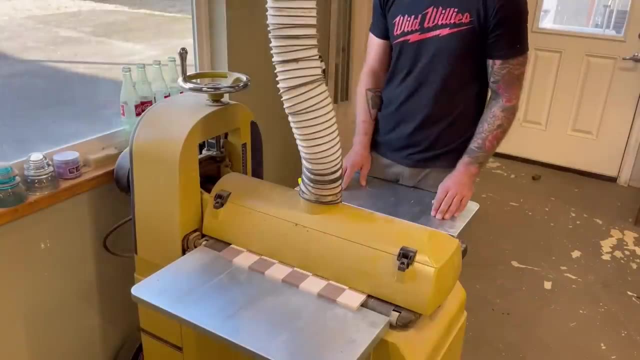 try and get these glued up as even and flush as possible, because this is going to be the finished size of your chessboard. After my glue dried, I pulled this out of clamps and it was back over to the drum sander to send it through on both sides and get the top very smooth. And look at. 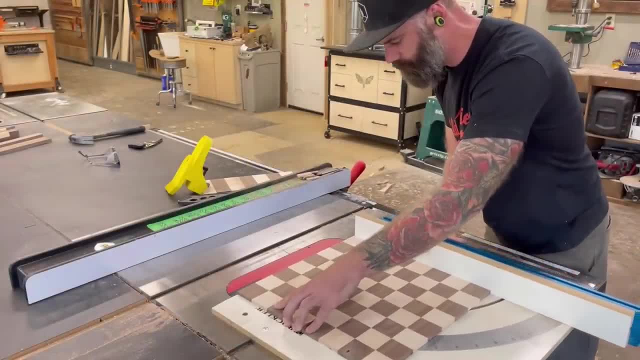 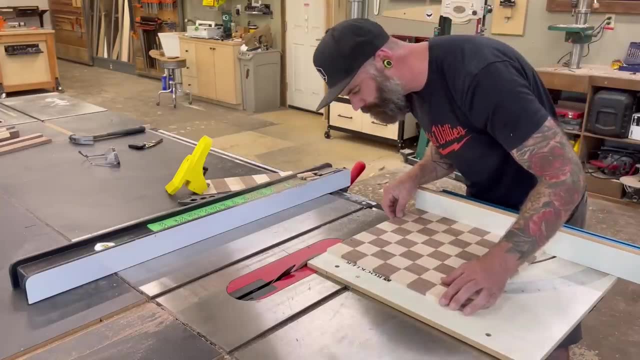 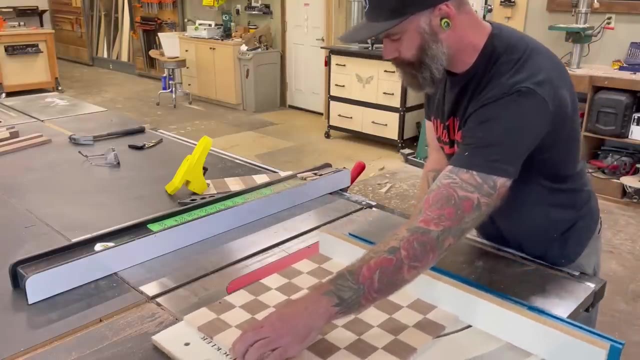 how nice and fresh. Then, just to ensure that I had nice straight edges on all four sides, I went back to the Rockler crosscut sled and I just took a wisp off each side, not really removing any mass amounts of material, just making sure that everything was nice. and even This shouldn't. 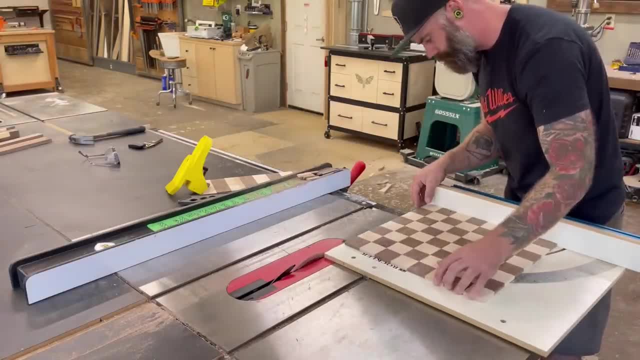 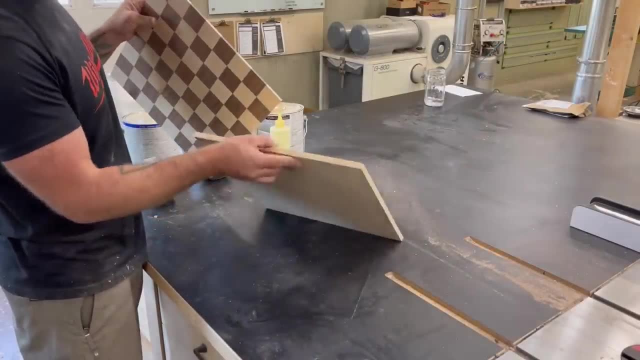 affect the look of the overall checkerboard slash chessboard in any way, shape or form. Now you might have noticed that the chessboard is pretty darn thin: It's just under a quarter of an inch, and that was by design because of wood movement. We're going to lock this entire. 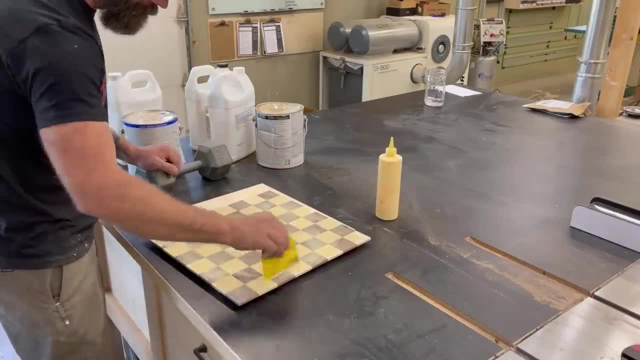 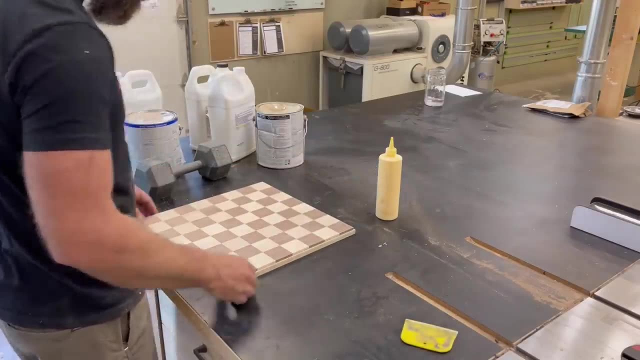 chessboard into a mitered border. And if we did the chessboard in full thickness wood, well, that internal wood would want to move and expand and contract with seasonal wood movement and it could bust the seams on our mitered border. So we purposely made the chessboard really thin. 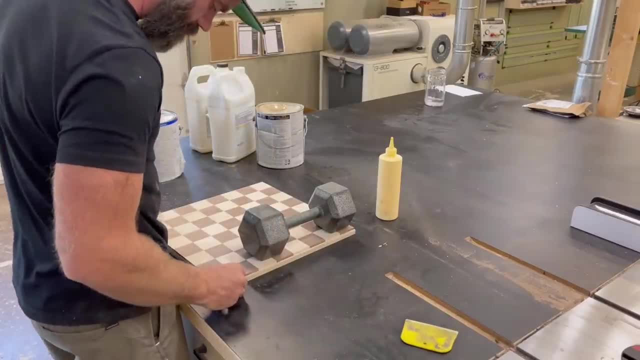 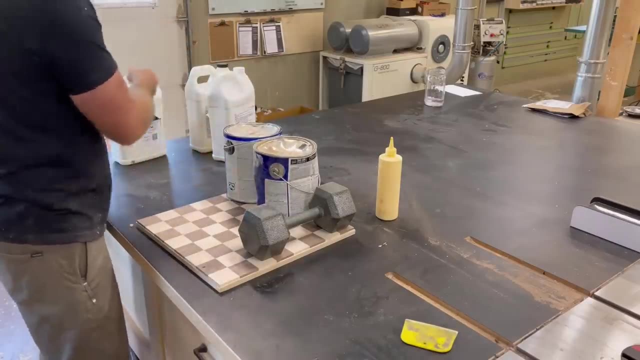 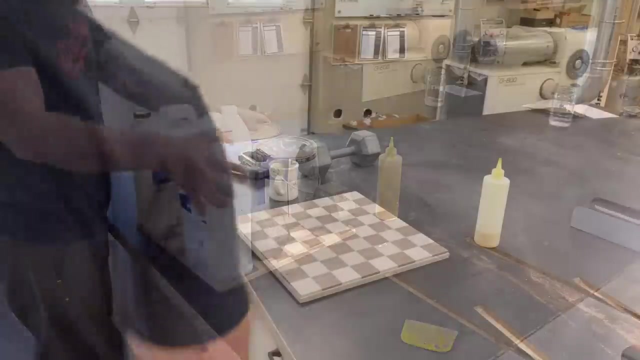 and then we glue it to a substrate of half-inch Baltic birch plywood. We just smeared some glue on the back of the chessboard, stuck it on top of the board and then glued it back together. Here's one thing: that epoxy is really good at holding things down. 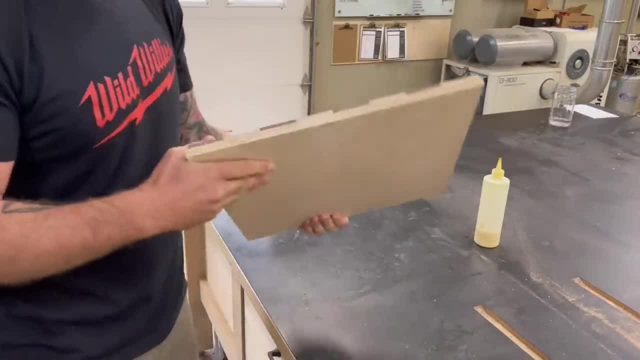 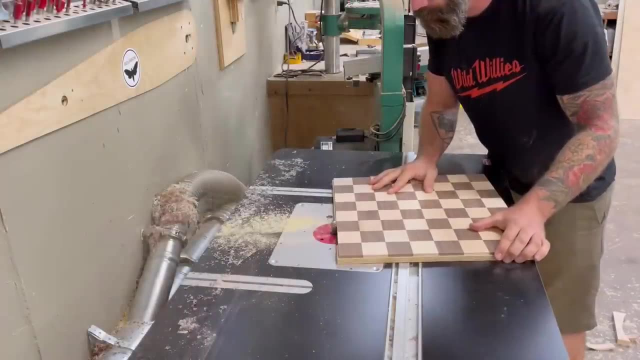 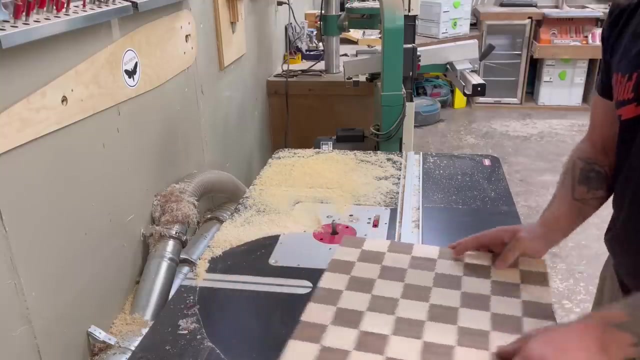 In a half an hour or so. my glue was dry and, as you can see, the plywood is just oversized beyond the edge of our actual chessboard. This was so we didn't have to get it perfect, But then we did get it perfect by taking it over to the router table and using a bits and bits compression. 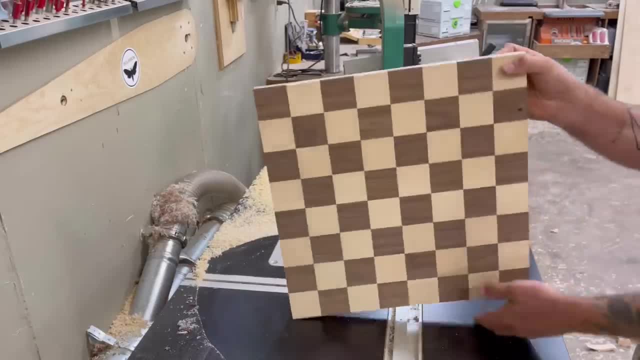 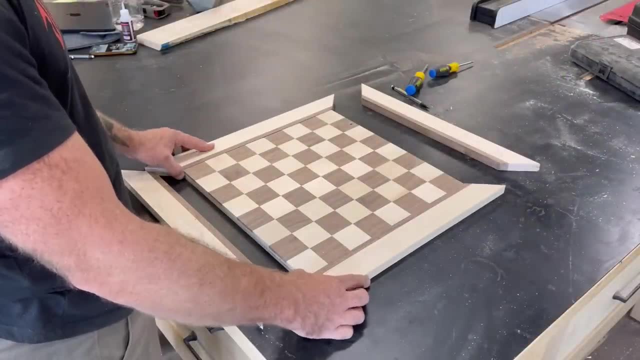 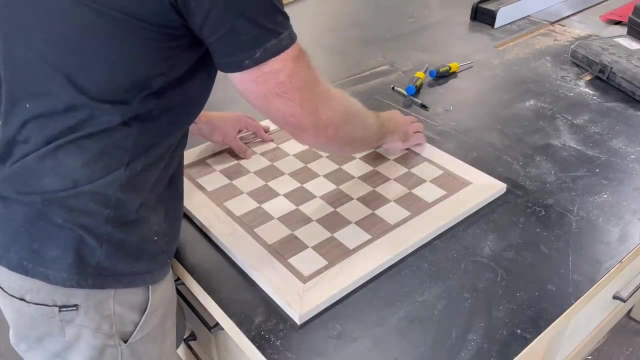 to make it look like a real chessboard. Now it was time to put our border on Now. I didn't show you this part, but I glued up some bits of walnut and maple together and I cut all the pieces for a nice mitered border, Just to give the whole thing a little more class and flair. All I really 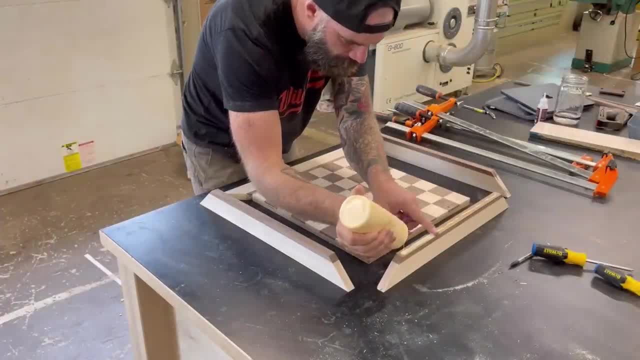 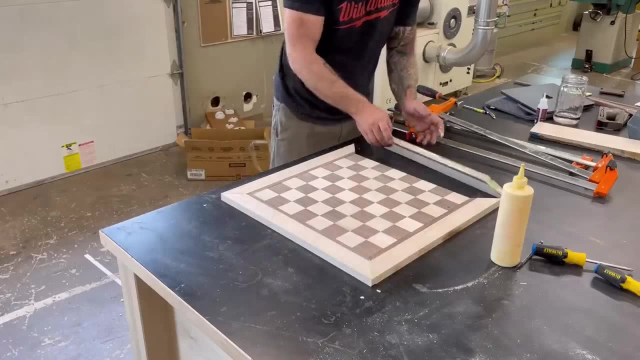 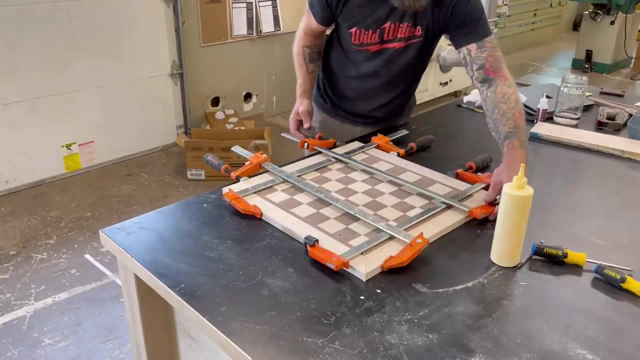 do is make sure all my pieces fit properly, smear glue on all my parts and pieces and then throw the board out of clamps. As long as all your pieces are cut the right size, you shouldn't need any fancy clamps here. I just used four little bar clamps and you don't need a lot of pressure. 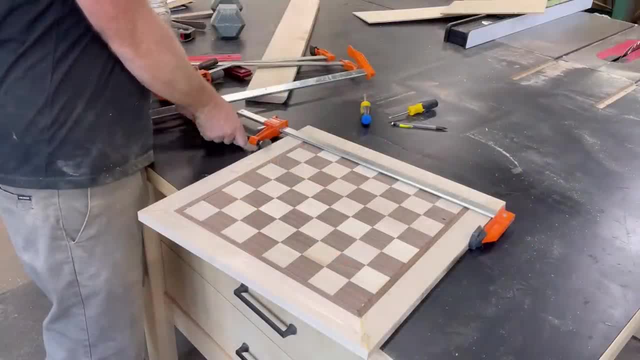 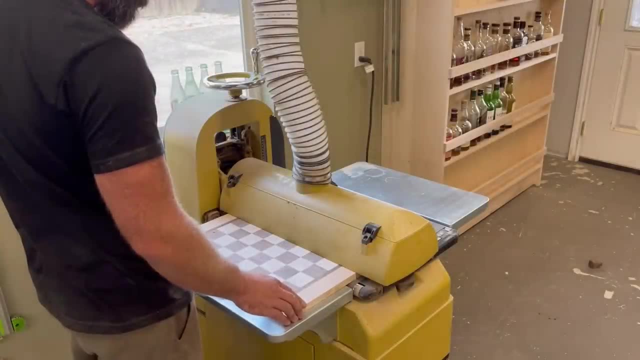 Just enough to get a little squeeze out. Don't over tighten those clamps. Pretty soon my glue was all dry so I could pull the board out of clamps, and then it was one more time over to the drum, sander on both sides to get everything nice and flush across the top, and then I finished it. 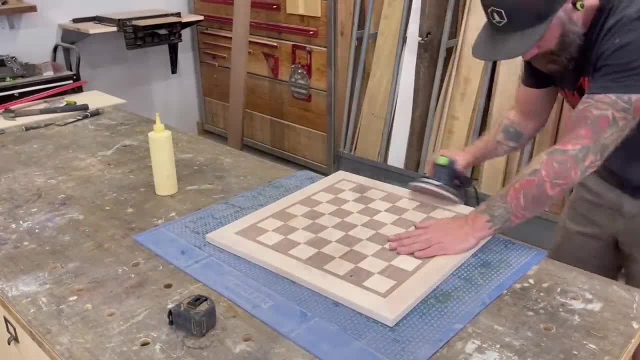 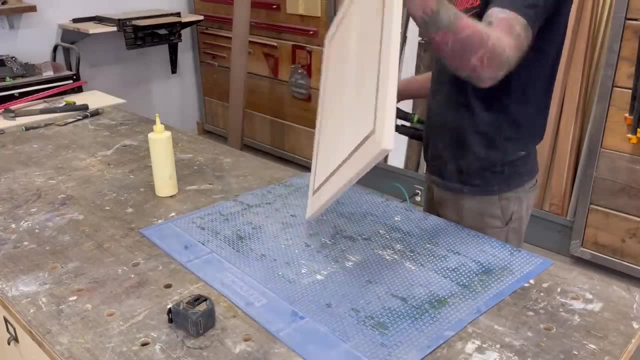 up with a little hand sanding And on the back it's just a nice clean, uniform surface. You could do some other board game on the bottom if you really wanted to take the time, but this is supposed to be a quick gift, So one. 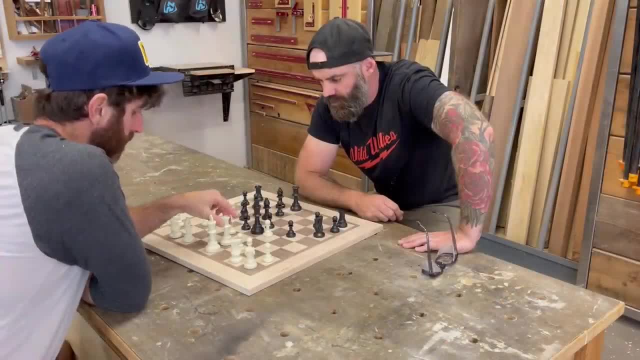 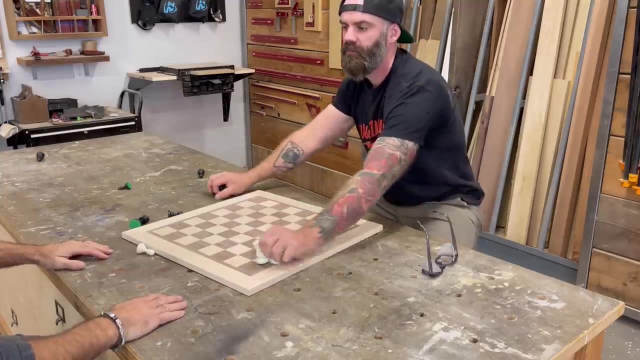 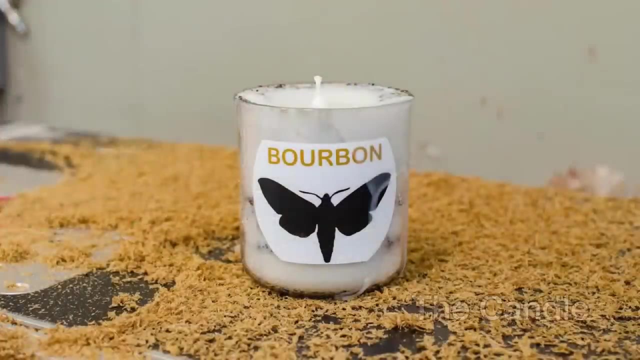 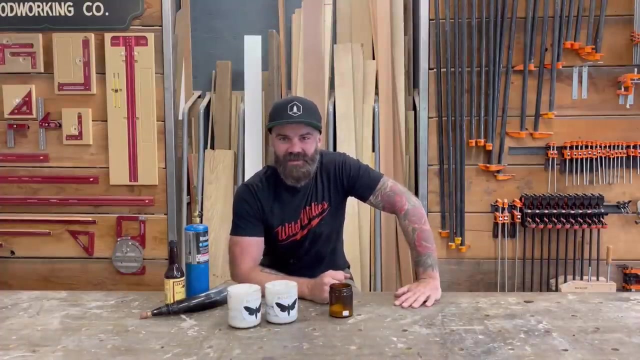 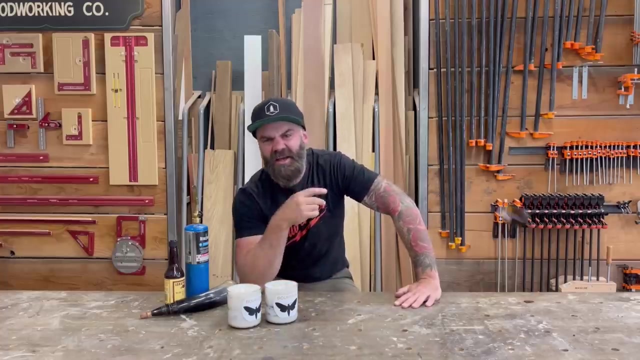 and done, Boom, Chessboard Checkmate. I just need to put finish on it. You know what I think is a giant scam? The candle industry. Every store you go into there's a candle and every candle smells like garbage, Like this one, Chai tea, Disgusting, All right. so I thought 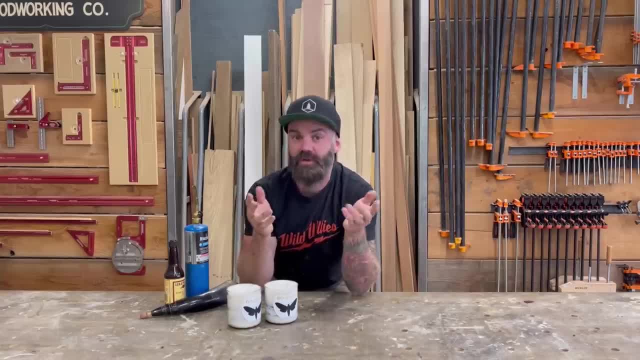 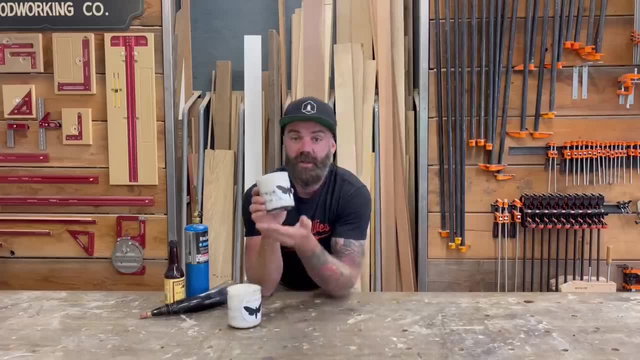 why don't we make our own candles Something a little more unique, Something that men or women working in a wood shop would appreciate? Let me introduce you to the Bourbon Ma Candle. It's got a little something special in there to excite your senses and entice the aroma which is life. 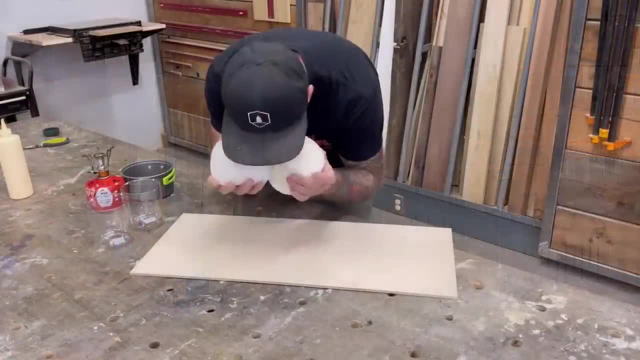 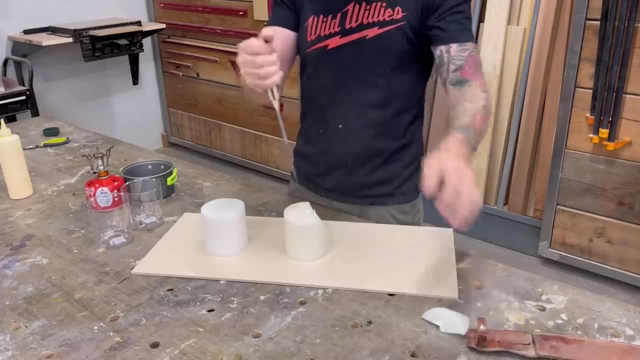 I'm putting that on my ad campaign. Anyways, here's how we made it. Now, I'd never made a candle before, so this entire thing was a little experimental. So I went to the store and I just bought some fragrance-free candles because I didn't want the nasty smells, but I needed the wax. 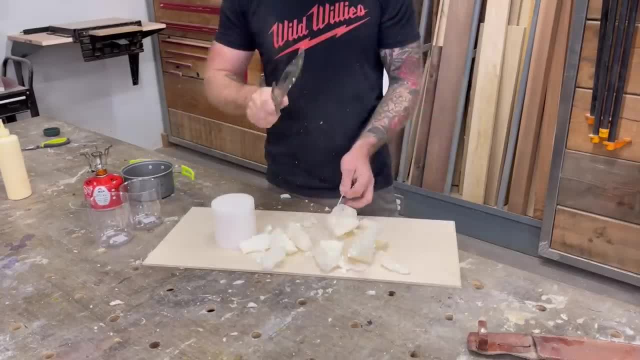 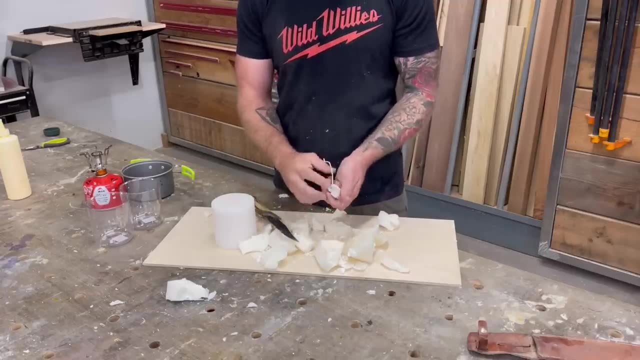 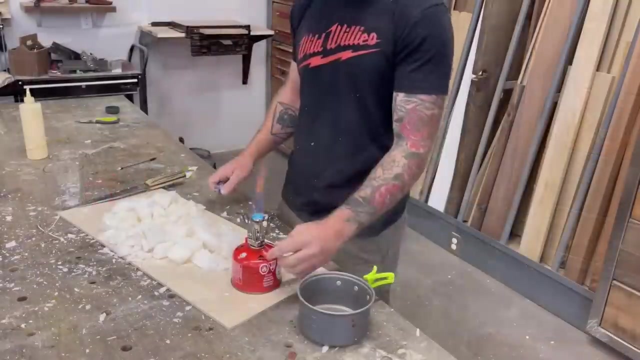 And then, using a big old hunting knife, I started breaking the candles apart until I had a lot of bits and chunks away And chunks of wax that I could melt down into my own special candle. I did make sure to save the wicks, because I'm probably gonna need those a little later on, After we got all of our chunks of wax broken. 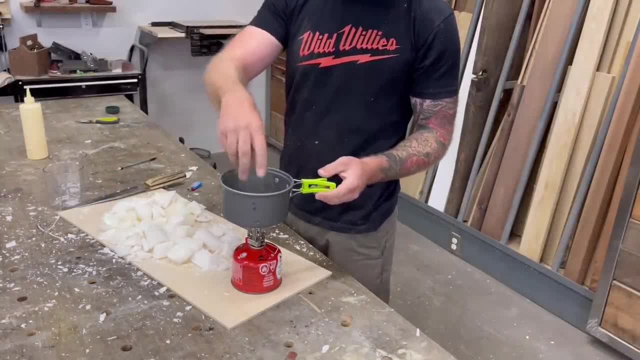 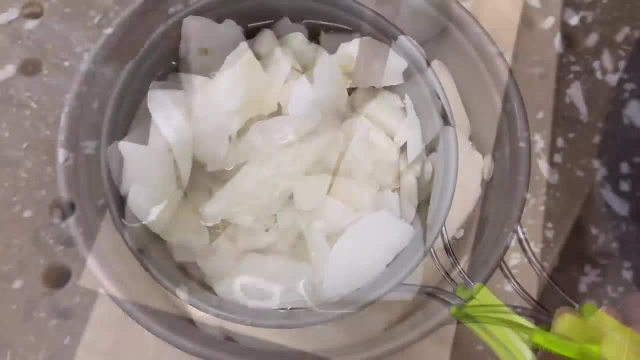 down from our fragrance-free candles. I pulled out a little butane camping stove and a pot and I started melting down the wax. Wax is crazy. I mean it's hard, but as soon as you heat it up it turns all liquidy Weird. 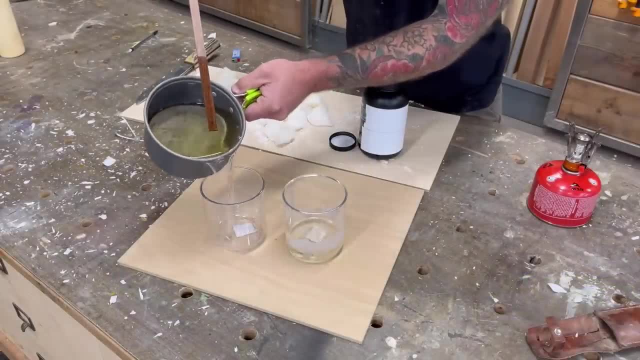 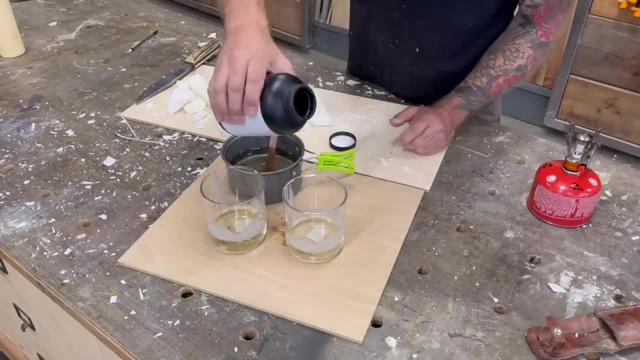 Science. After we had it all melted down, we added a little bit into some glass containers- These are going to be our candle molds- and then we could start adding in our own fragrances. I started with a little gunpowder because you know, I like the smell of gunpowder. 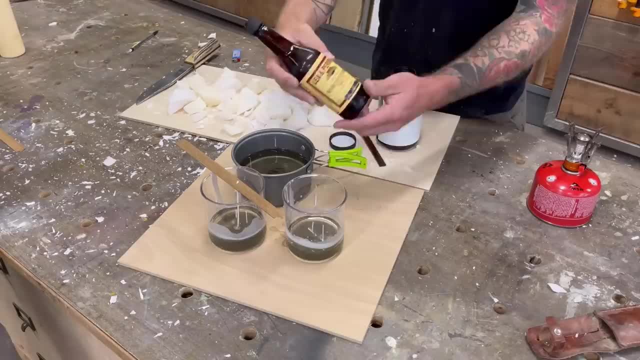 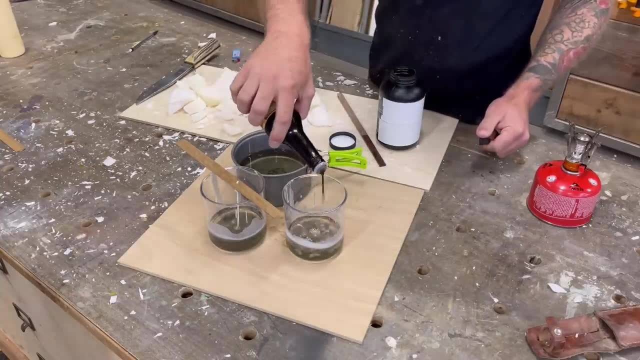 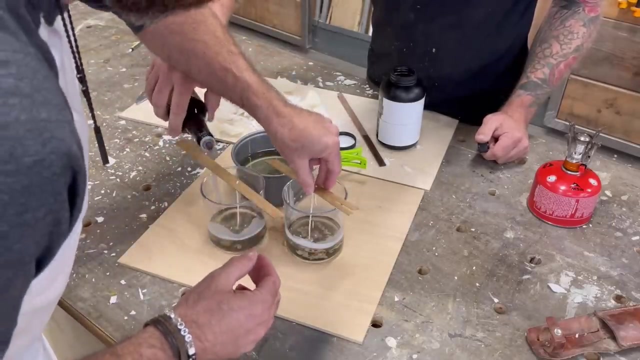 I remember going shooting with my dad when I was a little kid and it always smelled so good. Another thing I love the smell of is Worcestershire sauce, Wichester sauce, Worcestershire, Anyways, that brown sauce that you put on steaks and hamburgers. 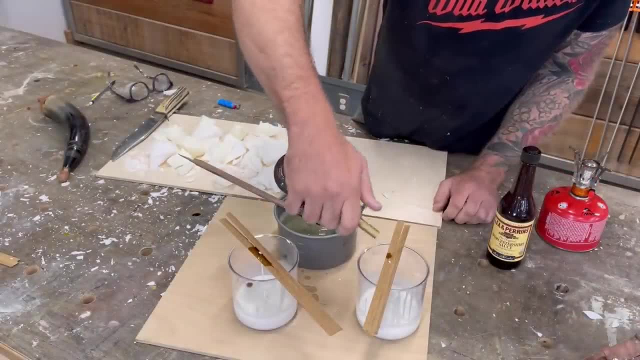 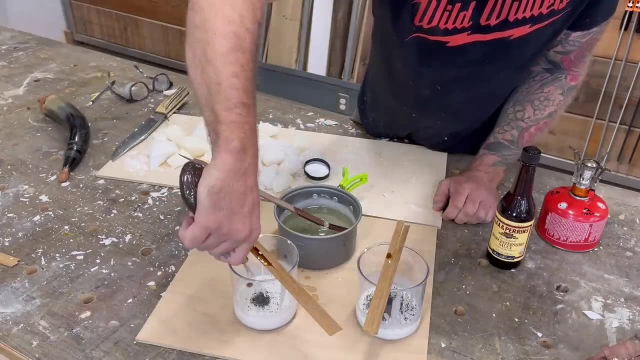 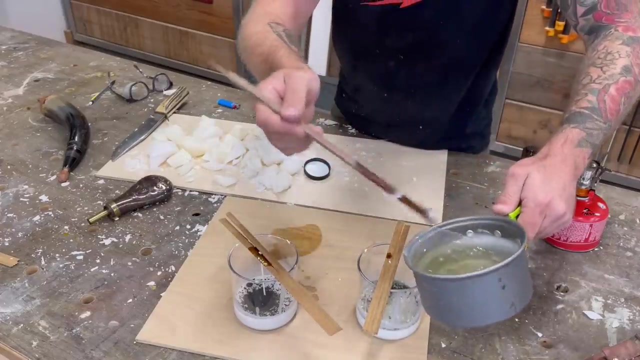 It just makes me think of backyard barbecues. so I thought it'd be a good smell. We just started doing the candles in various layers. We'd let a little wax harden, then add some more gunpowder. Once we got enough gunpowder in there, we'd add a little bit more wax and kind of mix it up until. 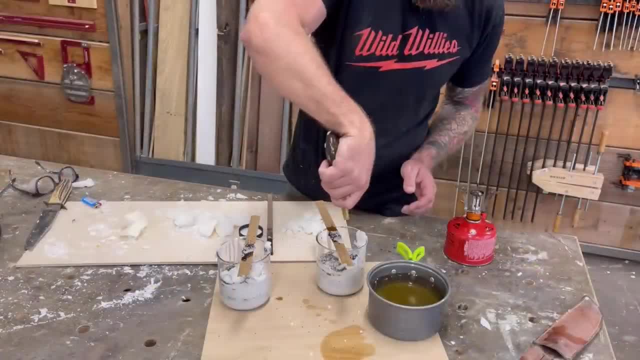 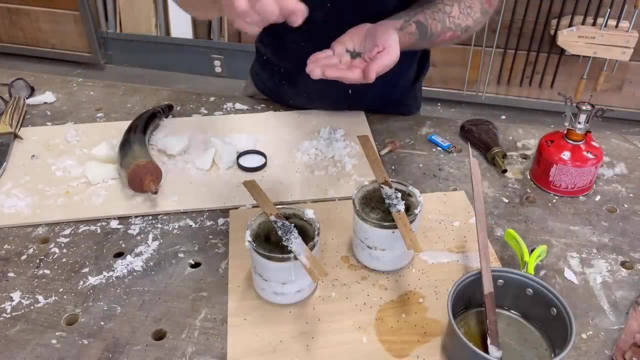 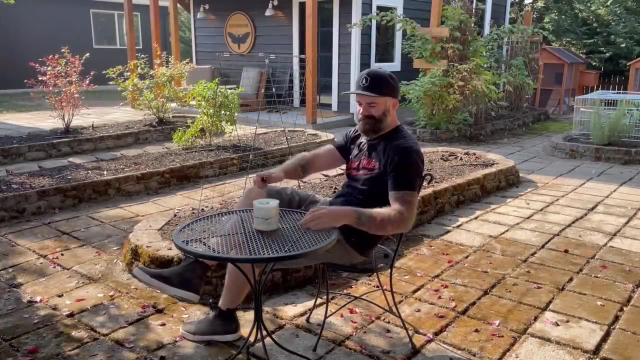 we got a nice mixture of gunpowder and wax all in one unified candle. Pretty soon our candles were constructed layer upon layer of wax and black powder, and I sprinkled a little more black powder on the top just for a added seasoning. Then it was time to go outside and enjoy my candle. 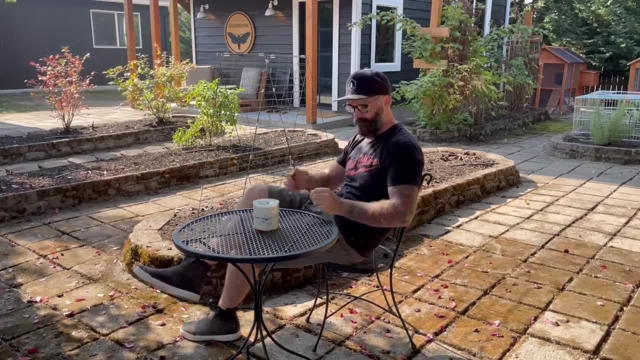 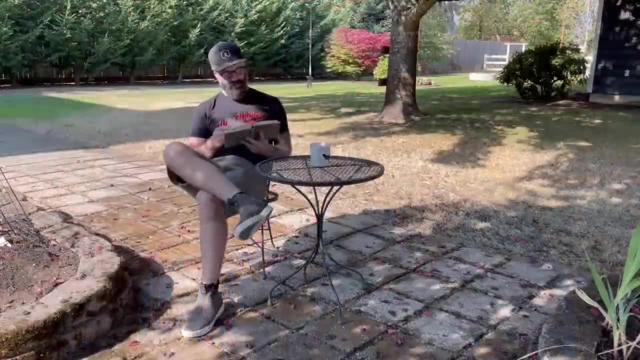 So I sat down in the garden, thought maybe safety glasses would be a good idea, and I lit my candle. You know, at first it was really nice and peaceful. It gave off a light aroma of Worcestershire, Worcestershire, The brown sauce smell. 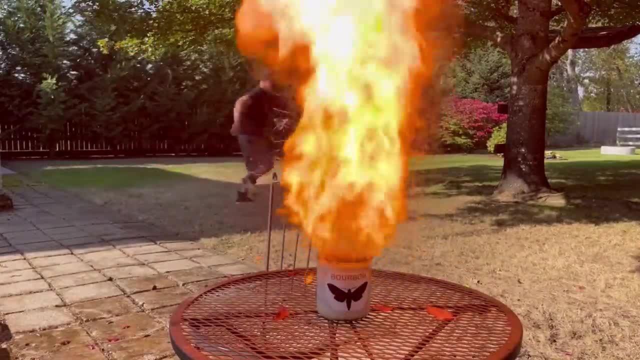 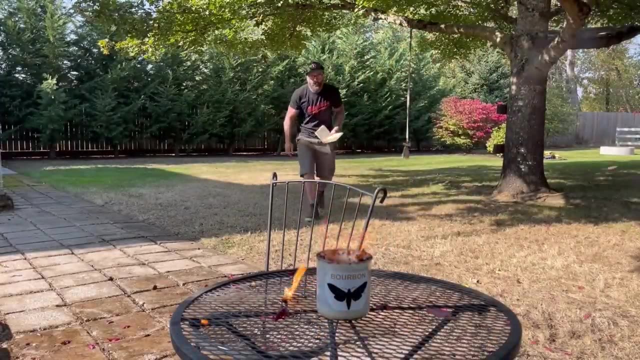 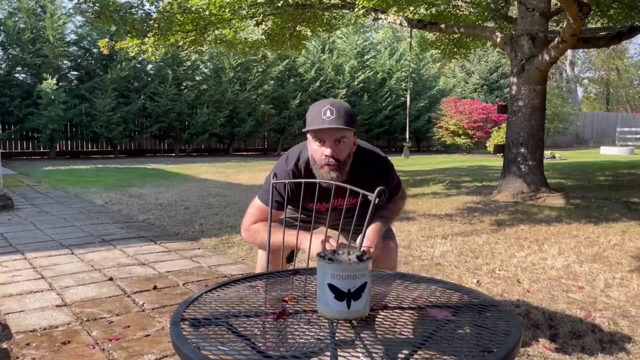 All of a sudden things got a little crazy. I'm not going to say that gunpowder in a candle is a bad idea. It just might not be something for your average candle consumer. But to each his own. I flippin' love it. 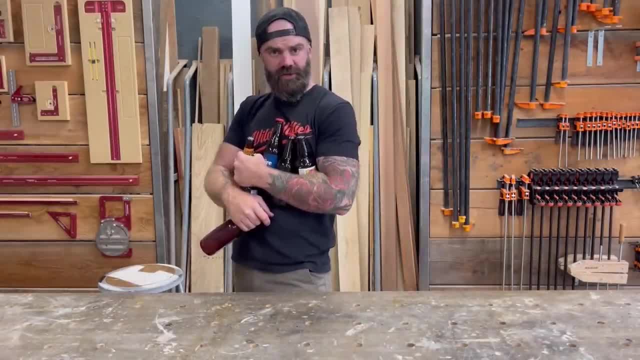 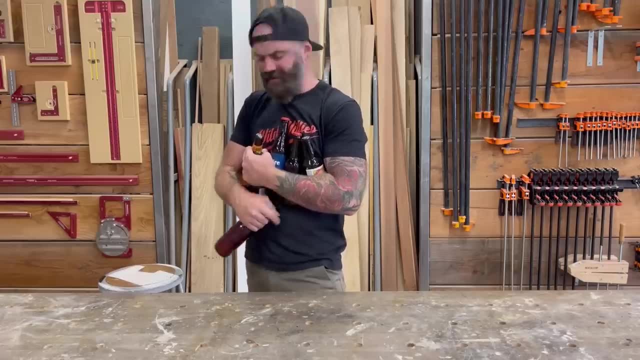 You ever find yourself in this situation. You're walking around the grocery store, you got a bunch of single, random bottles of beer and you got no place to put them And you look ridiculous. Well, that's why you make one of these, This nice custom six pack. 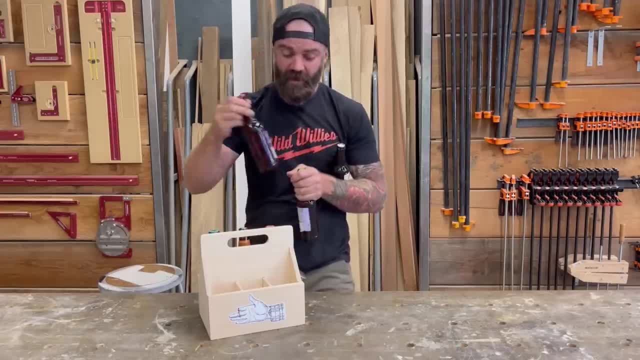 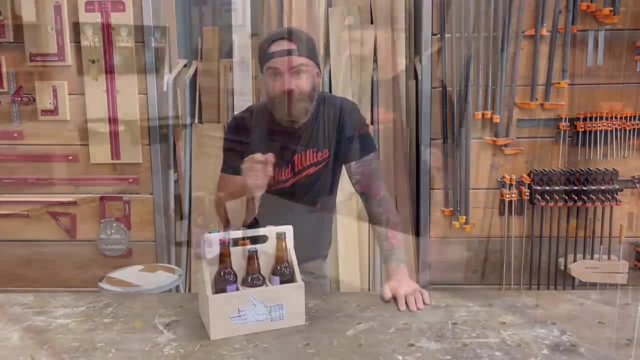 beer holder, And the cool thing about this is you can make it fill it up with all your favorite beers and then give it away as a gift, And I'm going to show you how to make it right now. Now, this is a pretty easy one. You need to have a little bit of time to get used to this. You need 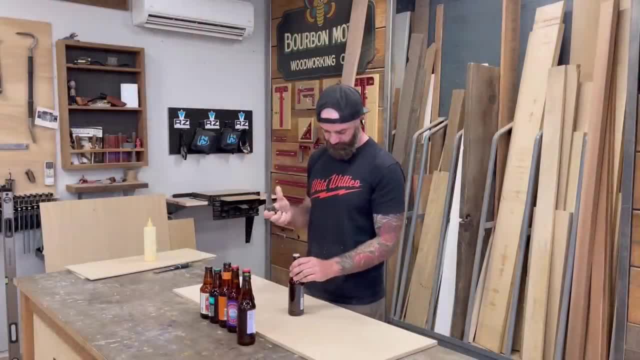 to have a little bit of time to get used to this. You need to have a little bit of time to get used to this. You need to start with a scrap piece of plywood. I'm using half inch Baltic birch. Then you take a beer, pop the top and take a good long sip. 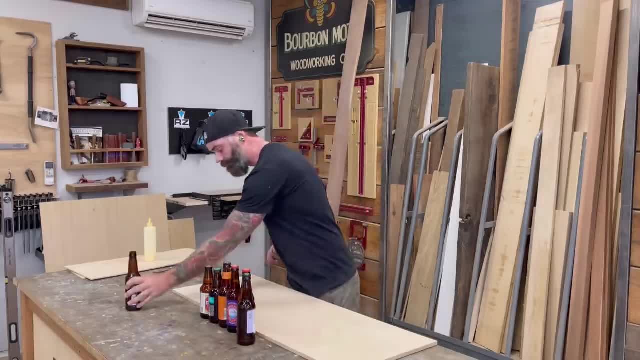 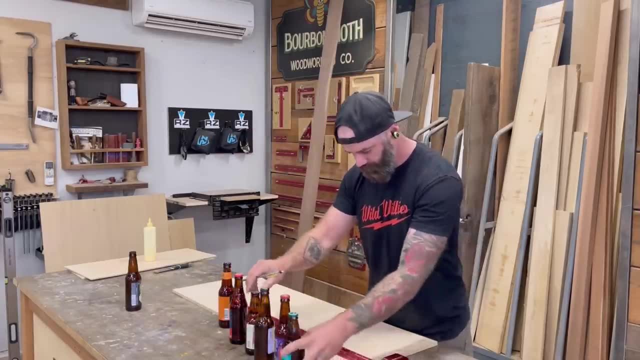 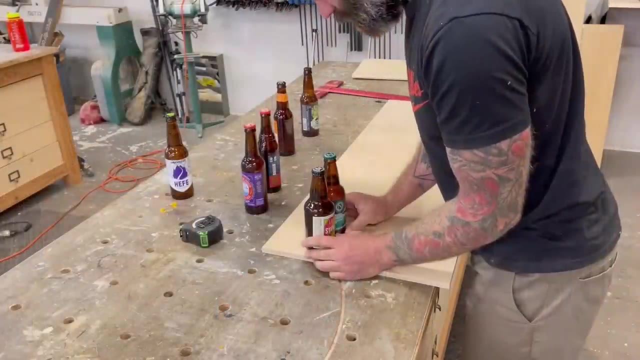 Because it's nice to have a refreshment while you work. After doing that, you're going to use your bottles to figure out the measurements to get an actual size of your beer caddy. I like to get an assortment of different sized bottles so that I know big or small. whatever I get, they're going to fit in my caddy. 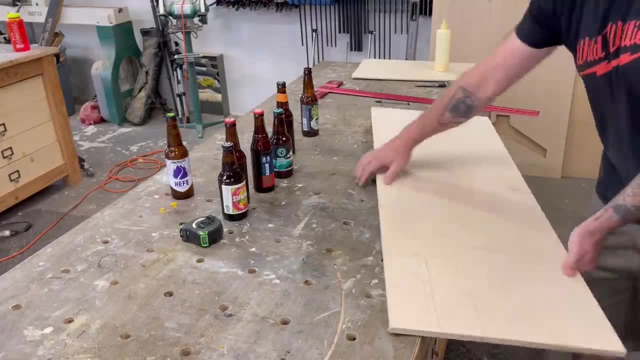 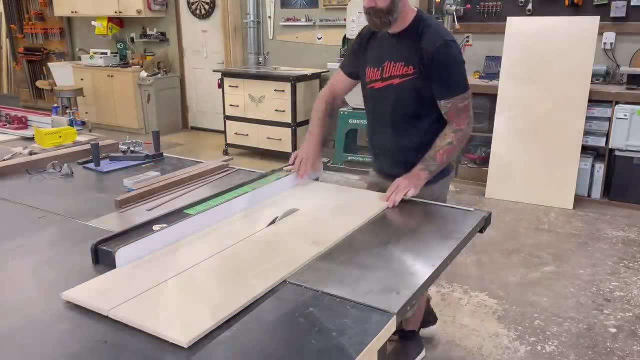 You also need to account for a half inch middle divider. That'll be the handle in the center of the caddy. Once you have that measurement all figured out, you go over to the table saw and you cut down a strip of plywood to that width and you cut it to length. 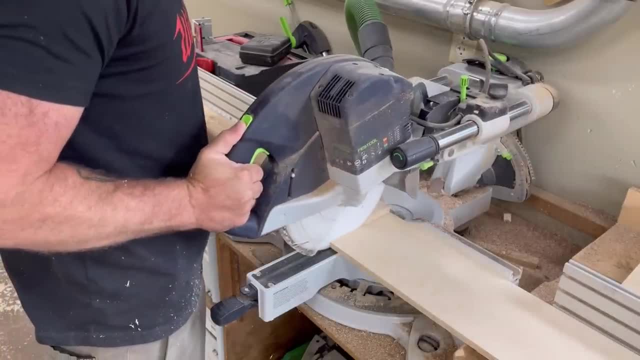 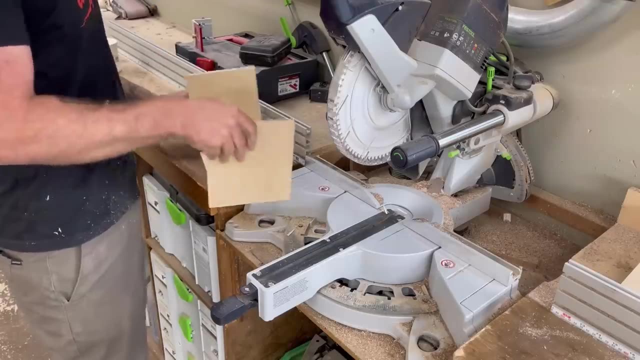 Now you got the base plate for our caddy. Then, using that same strip, because you want these pieces to be the same width, you cut down two side pieces. Those will hook on either end of the base plate for our caddy. Now the side pieces need. 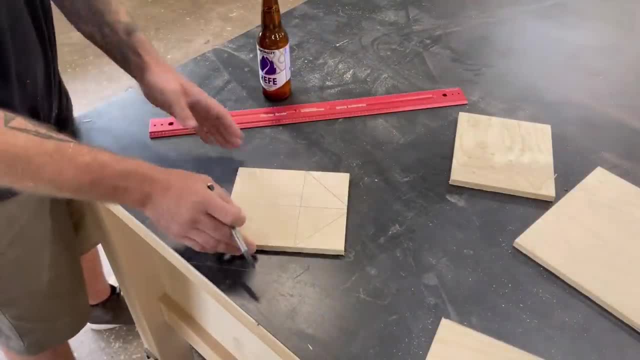 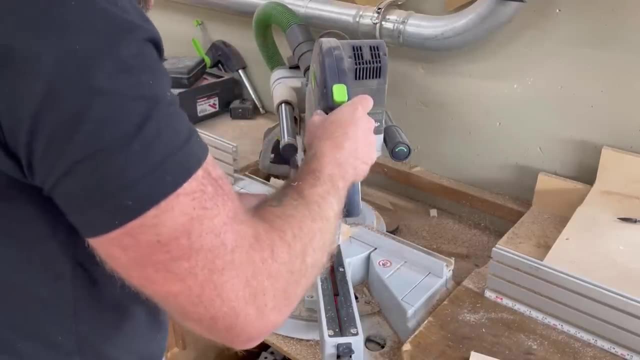 To look like an actual six pack carton thingamawatsit. So we're going to cut them at a taper on the top And because both sides are going to be identical, you can cut both of these at the same time. Just be careful once you get those cut down. 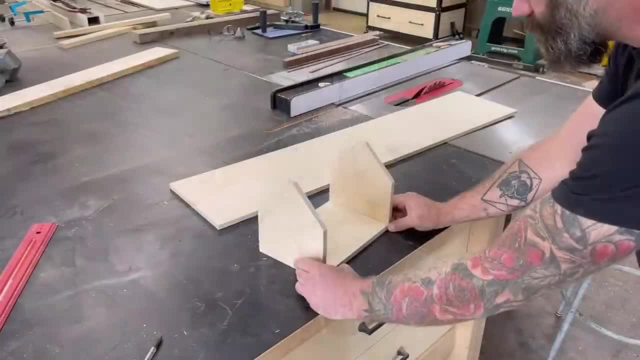 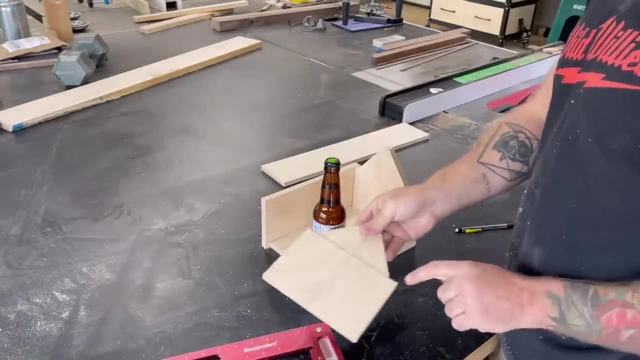 So they're starting to look like the sides of a six pack beer holder. Next, we need to figure out the front and back of our little caddies. So we cut those pieces And I also added these little tabs on my ends because I thought it looked better. 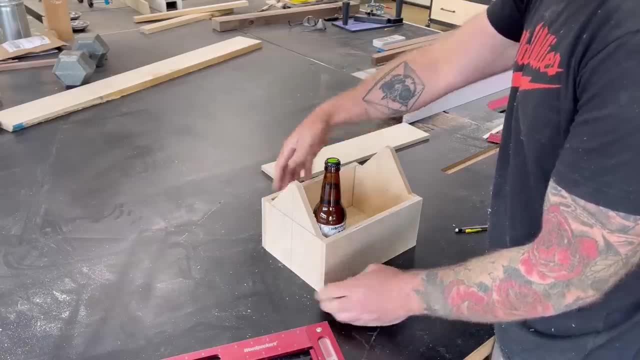 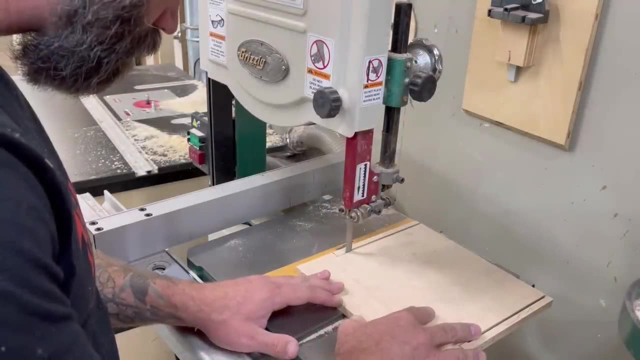 To have the tabs on there. don't ask me why it was a split second decision. Next, we need to figure out our internal divider handle. So I cut a piece that was the right size and shape And I add these little tabs on the top. 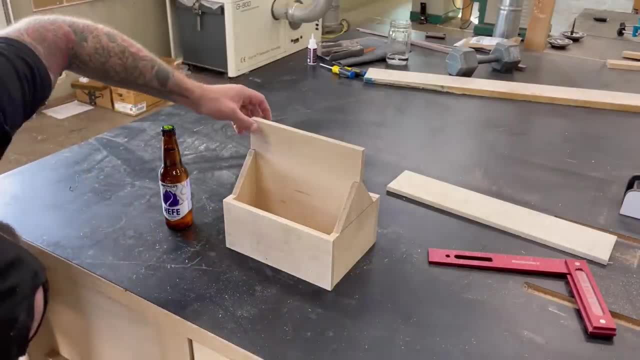 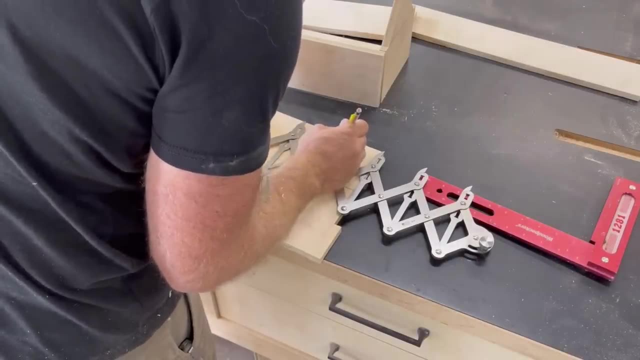 These tabs are going to sit over the edge of our little side pieces and it should fit in the center of your caddy Nice and snug. Then on the base of that piece. we need to divide it into three separate sections, Just like a real six pack beer holder. 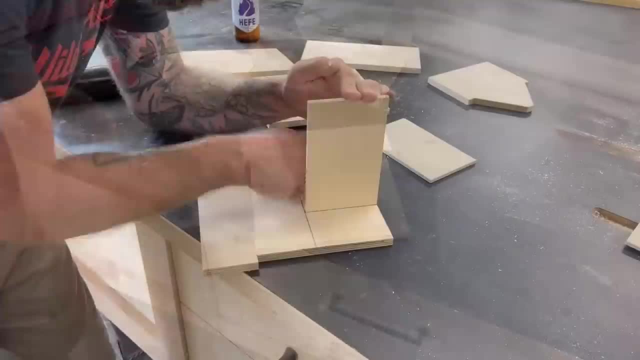 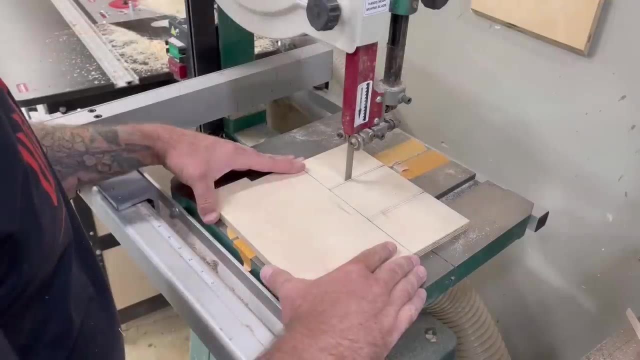 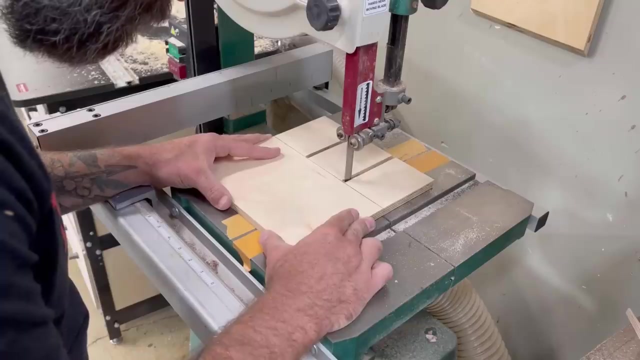 So I marked out exactly where three separate sections would be, and then we're going to do quarter inch Baltic birch for our dividers. So using my quarter inch Baltic birch, I traced out how much material I needed to remove so that I could slot those dividers in the base of my internal handle thing. 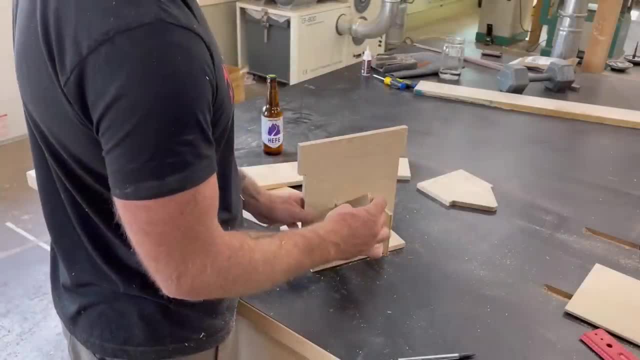 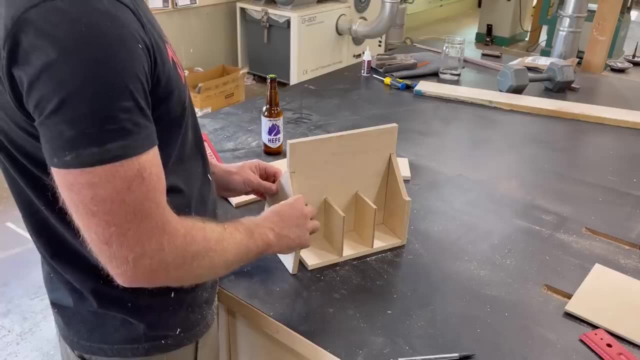 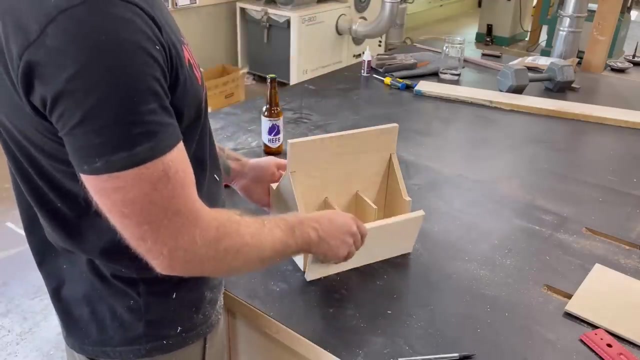 And I cut out those slots over on the bandsaw. Now you should be able to insert your little quarter inch divider things right in the bottom of this center handle piece and put everything back together and it almost is starting to look like a six pack beer holder. 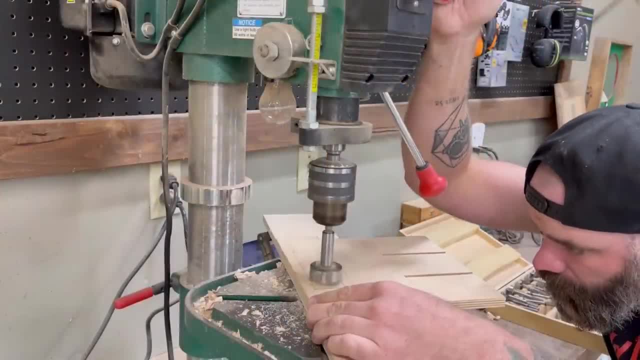 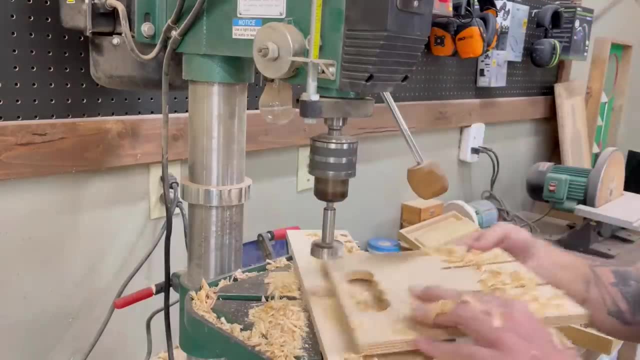 The only thing missing is the handle in the top. For this I just traced out where I wanted my handle to go and I used a Forzner bit to remove the mass majority of all the material for a little oval shaped handle. Then I cleaned up the whole thing. 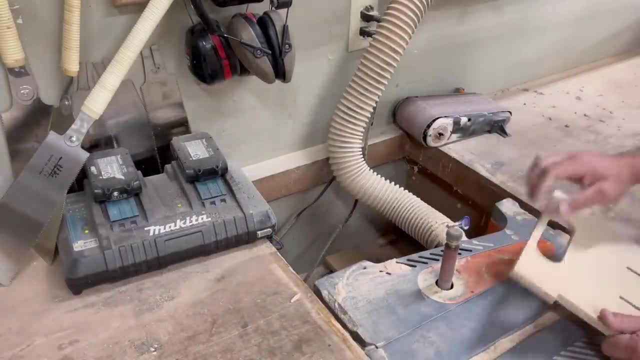 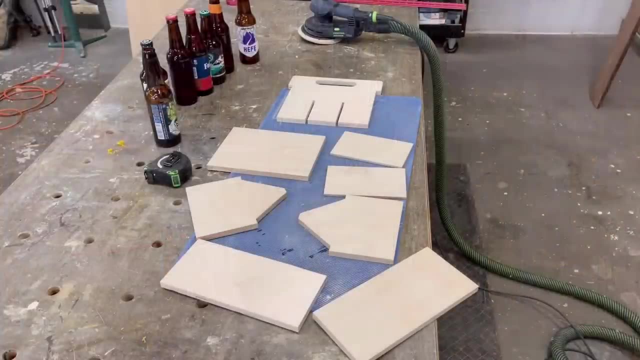 over on my oscillating spindle sander until it was looking nice and smooth. Then I took the time to pre-sand all of my pieces before assembly, because it's hard to sand once it's all together. You should have two front pieces, two side pieces. 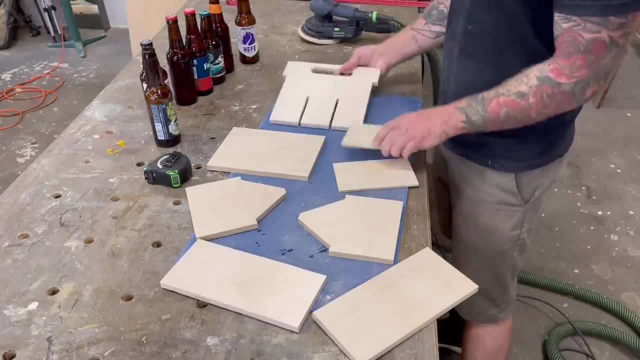 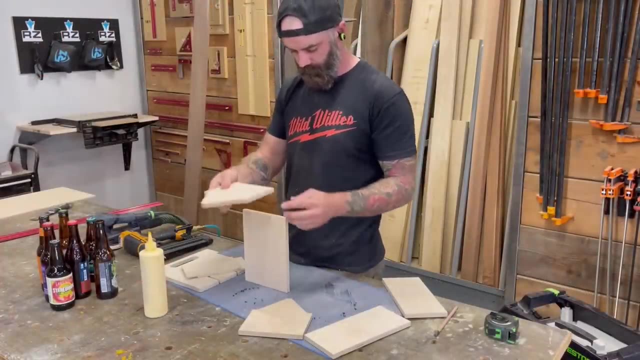 a base plate, two divider pieces and your internal handle piece that's slotted with an oval handle in the top. Then all you really gotta do is add a little glue to all your seams and I just tack it together with an 18 gauge brad nailer. 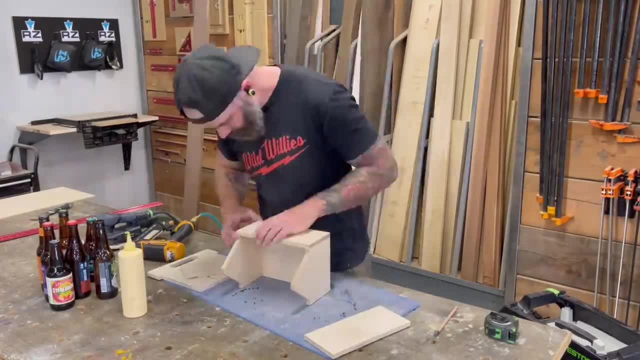 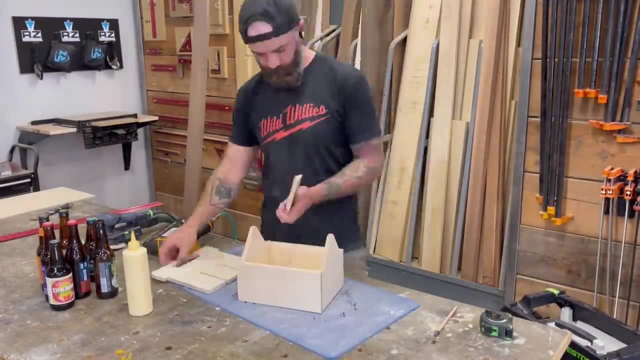 So a little glue, glue, glue, tack, tack, tack, zip, zap, zoop Jason's back. That's what I would say if that was a wrap, which it wasn't. I was just trying to give instructions on how to put this beer caddy together. 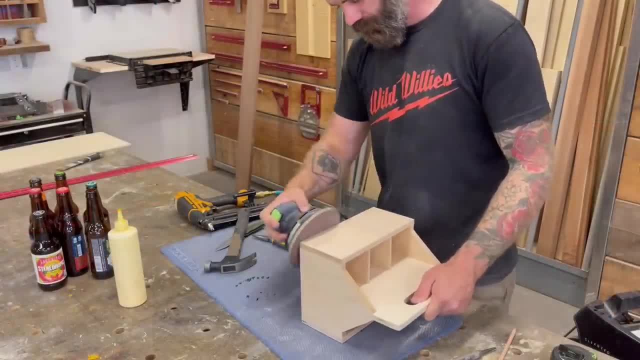 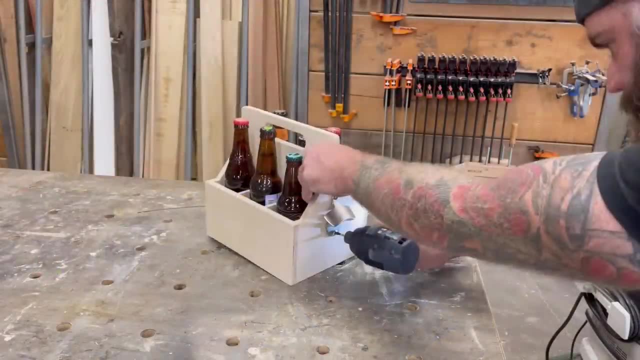 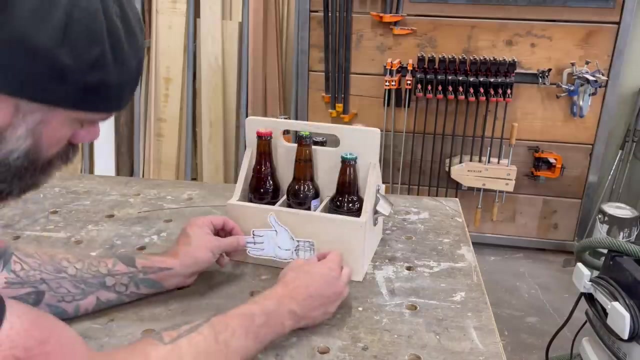 And boom, nice custom wood beer caddy. After it's all assembled, I just do a little finish sanding on the outside, making sure all my seams are even and smooth. I add a little bottle opener because you know you gotta be able to open the beer. 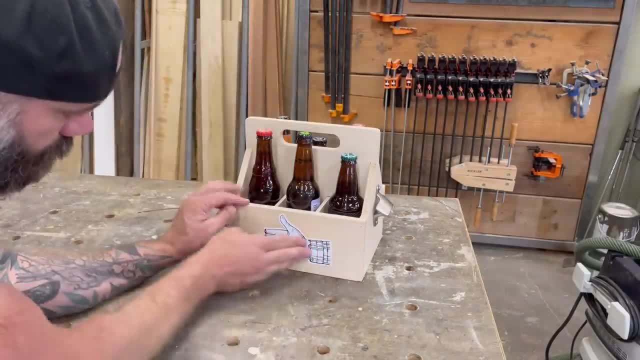 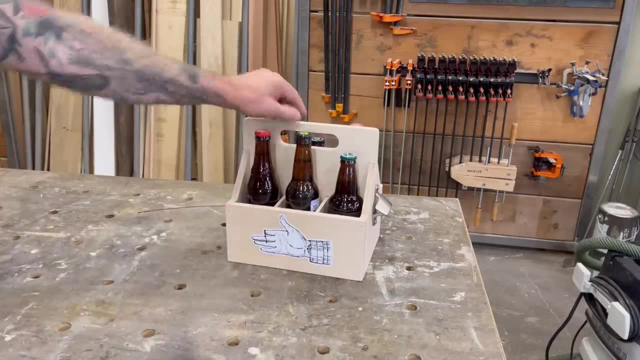 And of course, I added a nice little sticker for branding but also to remind people what happens if you drink and operate heavy equipment: You could lose a finger. Stickers available on my website. See, this is nice because you can get your whole variety. 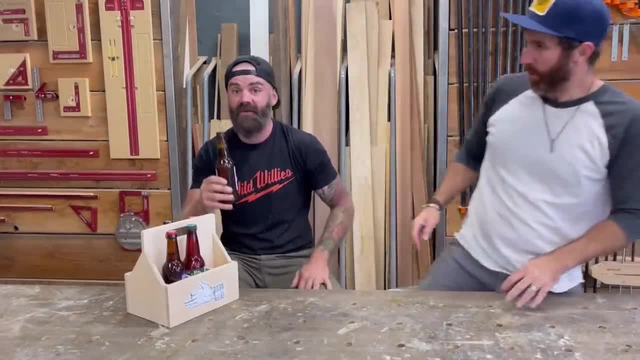 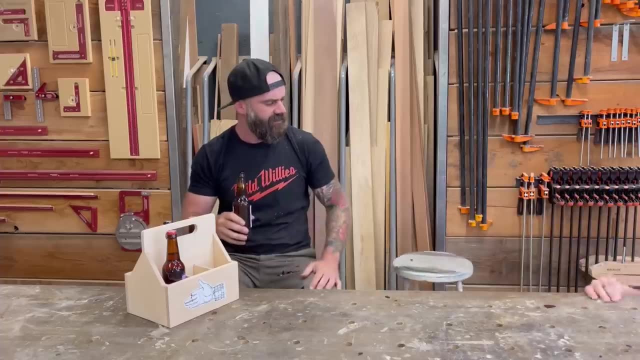 of favorite beers, take it over to a friend's house and then just have a cold one and enjoy it with your. Hey, thanks, man, Dude, you're on the clock, Get back to work. Anyways, you can just enjoy it with your friends. 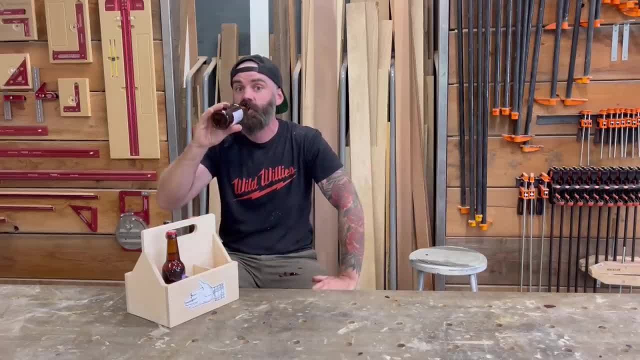 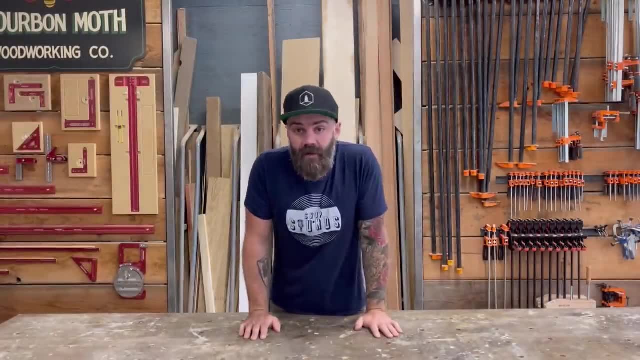 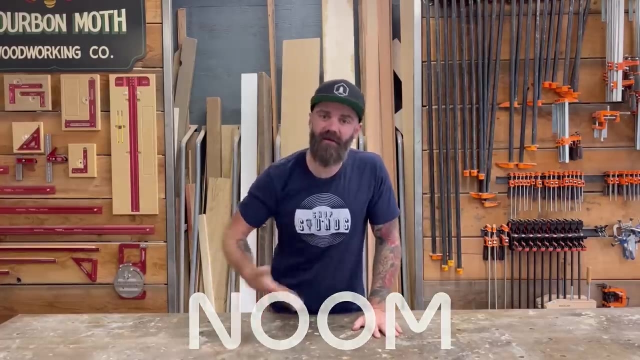 and leave it there as a cool gift. Hey, this video is sponsored by Noom. You're probably wondering what the heck's a Noom? Well, don't worry, that's what I'm here for: to tell you Now. you may have noticed in the last few months, 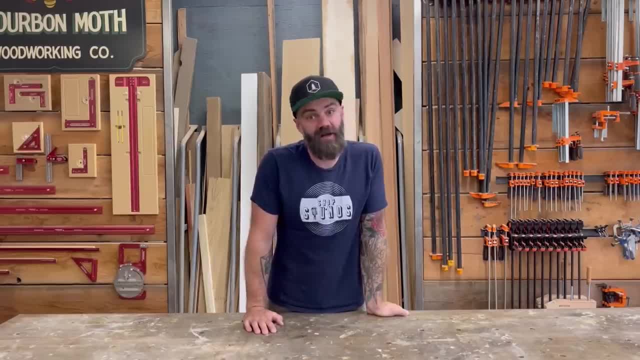 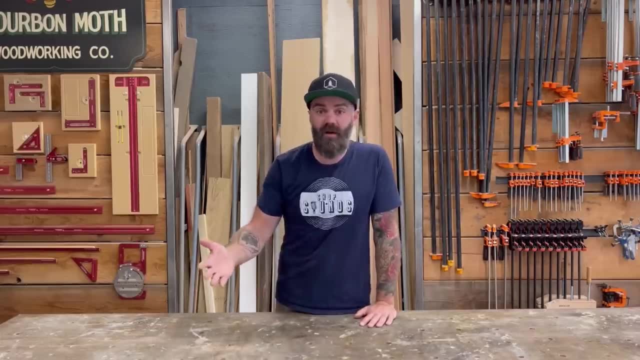 I've started looking a little slimmer, That's because I've lost some weight. I've been trying. I got a little hefty and I wanted to do something about it And like you, you know, maybe you've tried diets before. 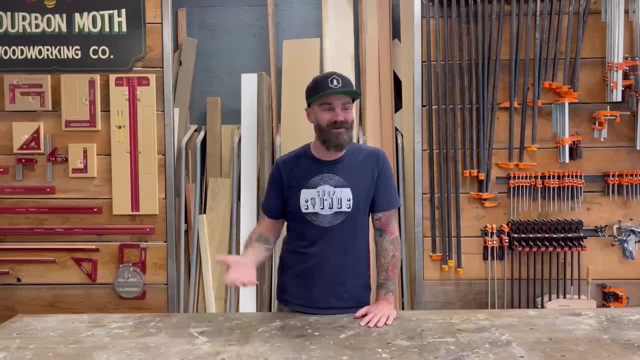 or exercise programs and they always work for a little bit, but then you get burnt out and you get tired of it and you end up falling off and going right back to your old habits. The cool thing about Noom is they approach weight loss. 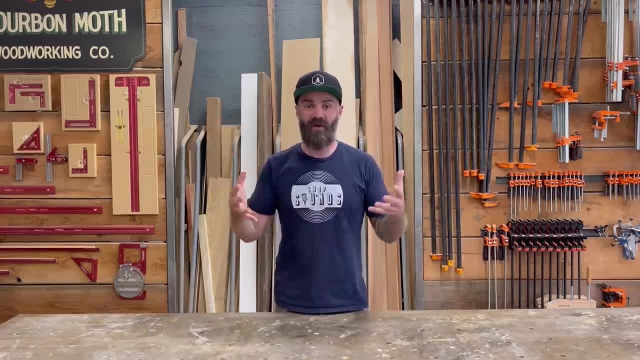 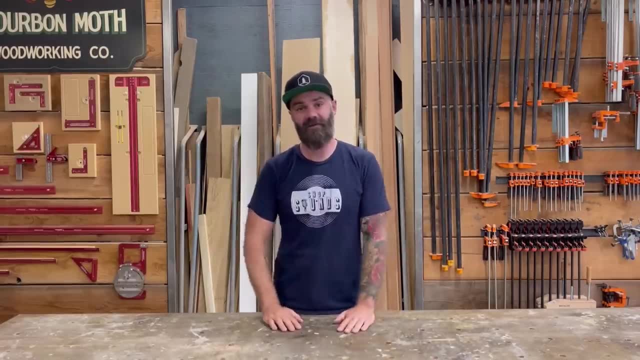 in a completely different way: psychologically, helping you figure out your habits- your good habits, your bad habits- and the best way for you to lose weight and get into a healthy routine. So the cool thing about Noom is that you download it and 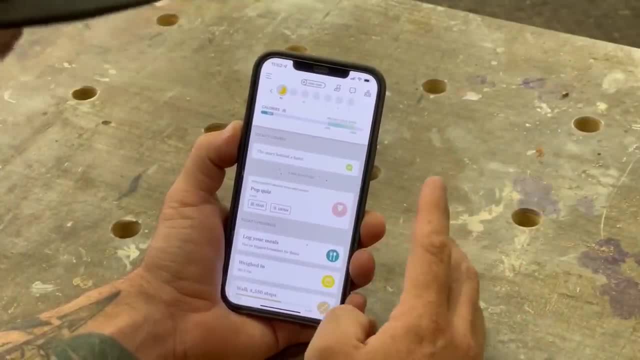 you download the app and then it's got everything organized to help you stay on track and reach your goals. Every day they're gonna give you a Noom course that you can go through, and they're all like a minute to three minutes. 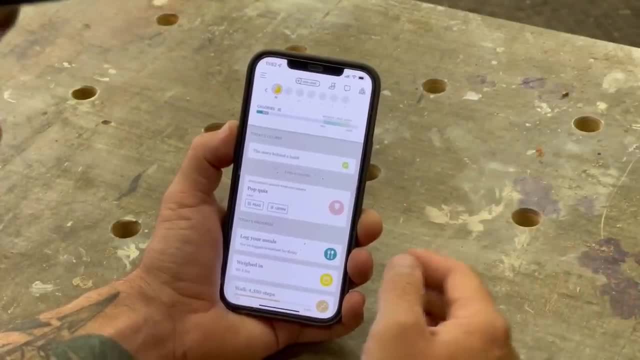 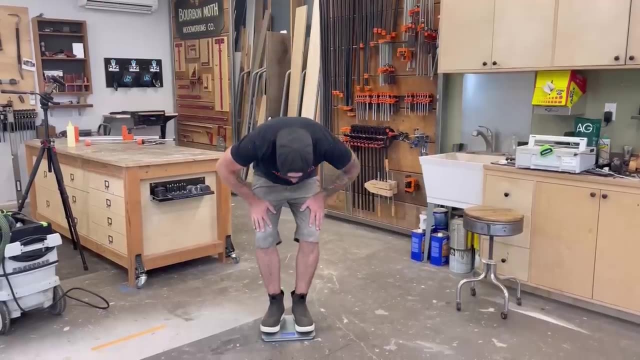 so it doesn't take very much time And they teach you cool things that I did not know before, Like, did you know that people that weigh in every day are statistically more likely to lose weight than people that don't track their weight- Which is nice, because you can track your weight? 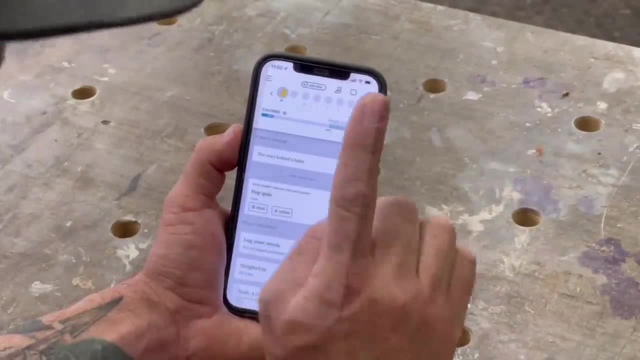 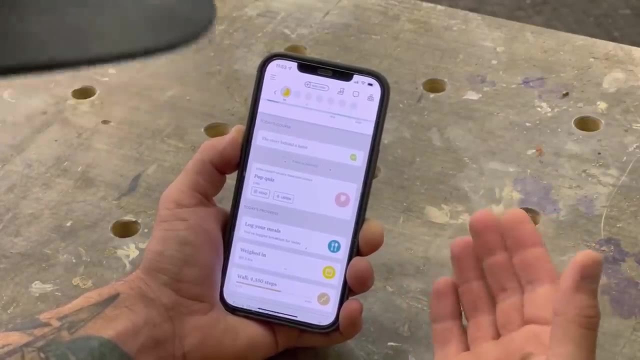 right down here You can log your meals and it counts your calories for you at the top. It tells you what range you should be in if you're trying to lose weight and if you're trying to lose weight healthily. They also teach you cool things about eating healthier. 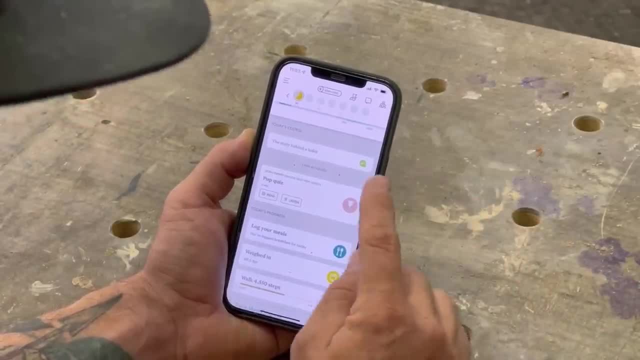 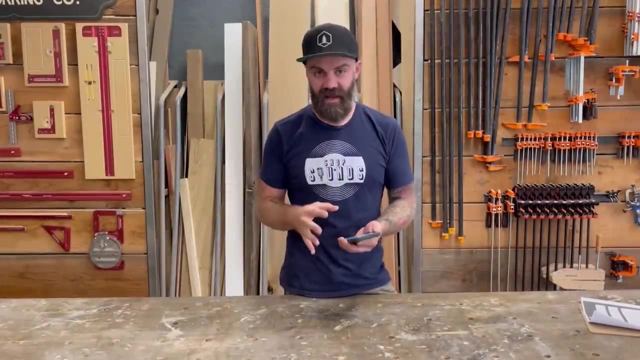 like caloric density. I didn't know that kind of thing, but now I'm thinking about that because of the teachings from Noom. The other thing I love about Noom is that it's not just an app. You really become part of a Noom community. 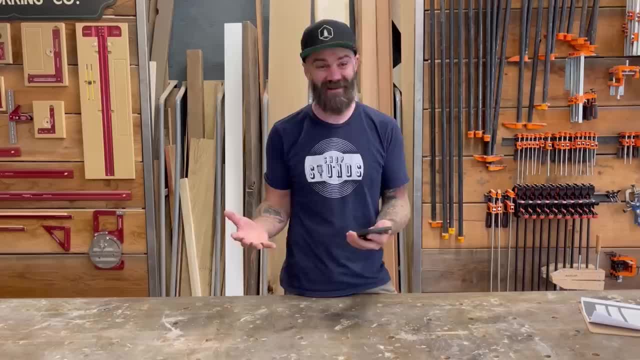 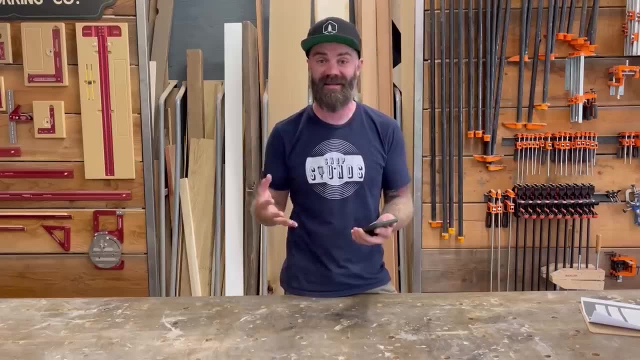 So if I have a question about a certain food or I'm just feeling discouraged that day because I ate too much, there's a live chat where I can chat with real-life experts and they'll give me the encouragement and information I need to stay on track with my goals. 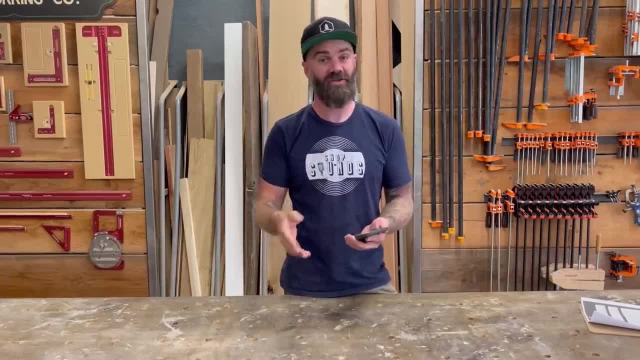 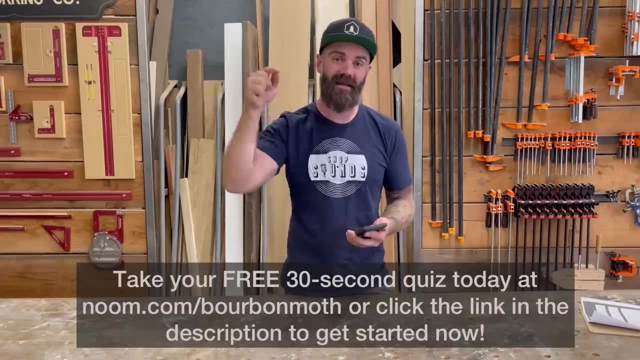 So if you want to try Noom, which I highly recommend, just go to Noomcom. slash Bourbon Moth, take a quick 30-second quiz and get started today, Or you can click the link in the video description. Just check it out. 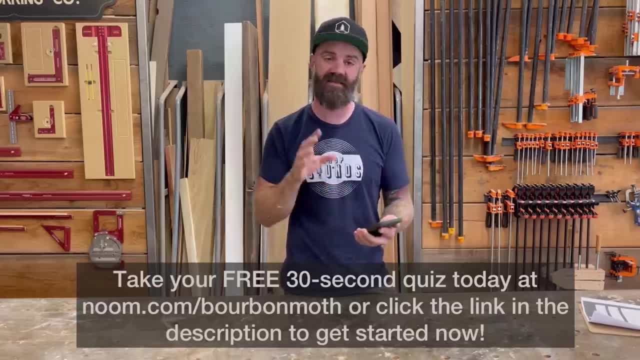 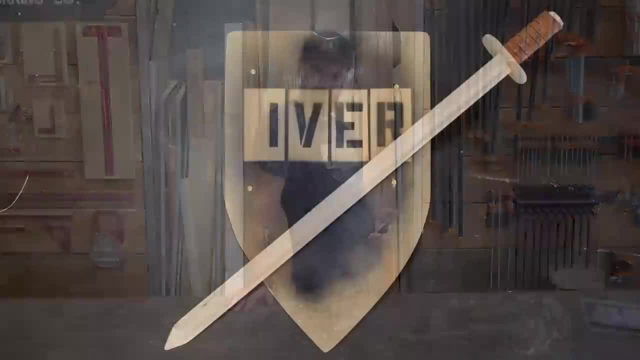 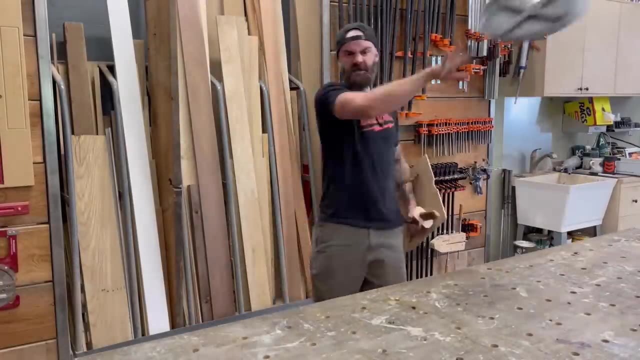 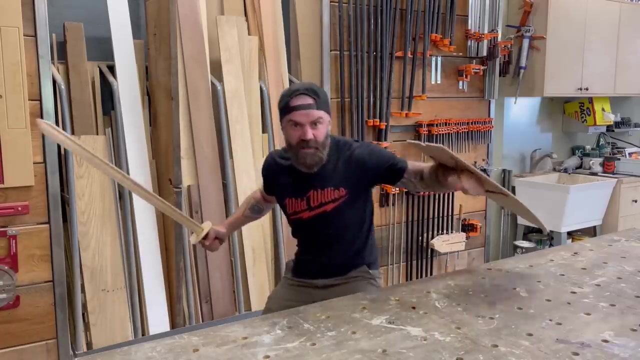 Give it a try. I know for me it has helped a ton. Stay focused, stay on track and accomplish my goals And I will say I am looking much better. Ready your breakfast and eat hearty for tonight. we die in hell. 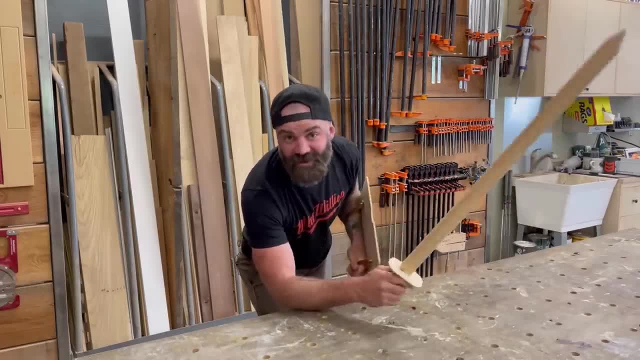 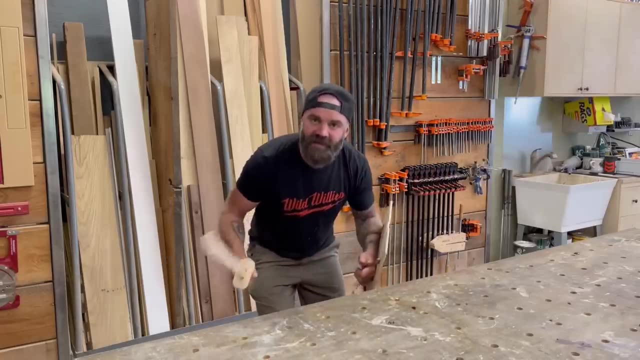 So as a dad I've gotten used to making a lot of swords in my days And at first I just started picking up sticks and saying: here, son, there's a sword. But the more my son grows and knows what's fake and what's, 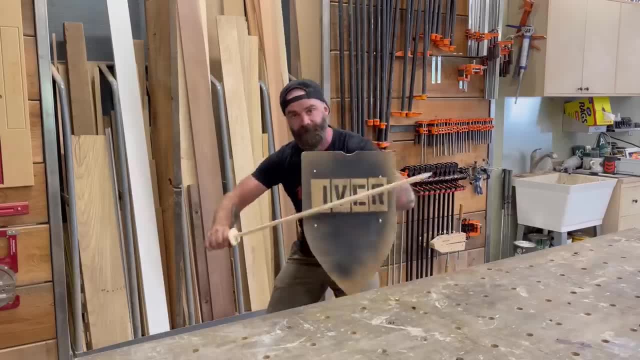 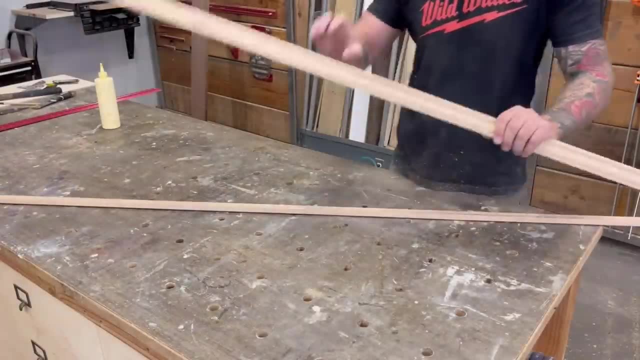 not, the more he wants realistic weaponry. So that's why I'm going to show you how to make this sweet sword And shield. Let's do this thing Now. after a lot of sword making and trial and error, I found that the best material to make sword blades. 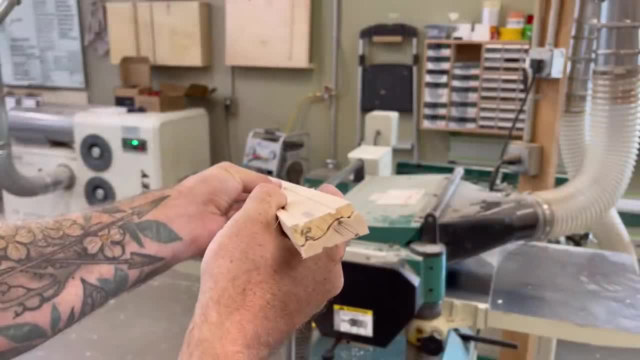 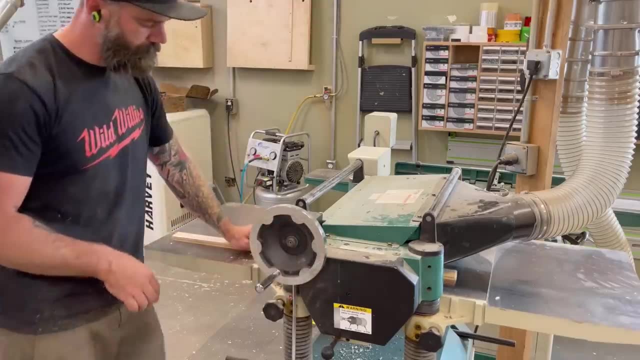 is trim molding, Because it's got all this nice profile- look to it- which you can form to look like an exact replica of an actual sword. All you got to do is thin it down a little bit, So putting two pieces together, so you. 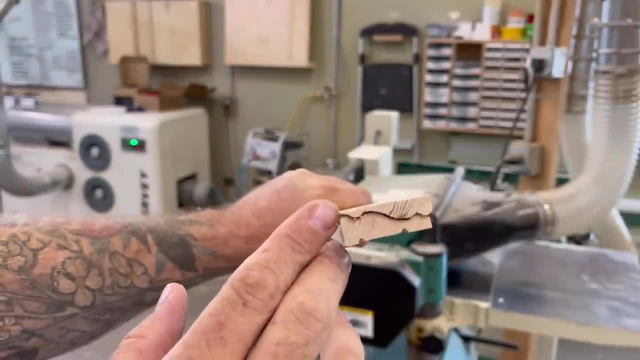 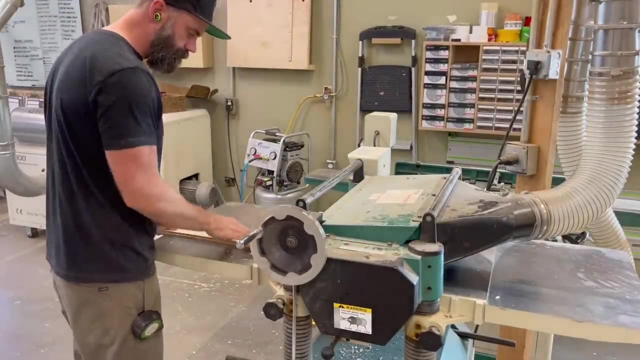 can run it through the planer. you run it through the planer until you see it starts to get nice and thin towards the tip. Once you do that to one side, you flip it over and you do the exact same thing to the other side. 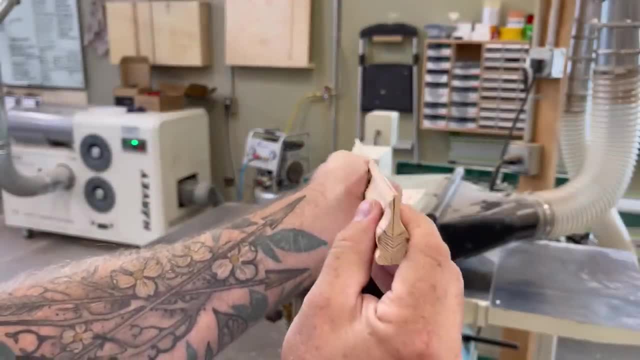 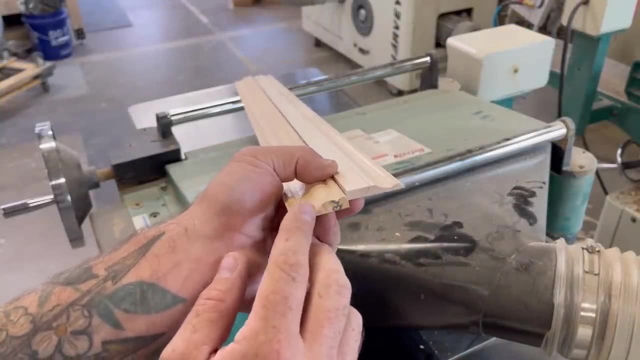 Then you can sandwich these two pieces together and you can see it starting to look like a sword on either side. Next I like to run it through the planer on the rounded side, just to flatten the one end a little bit. So I do that to one side. then I take my other piece. 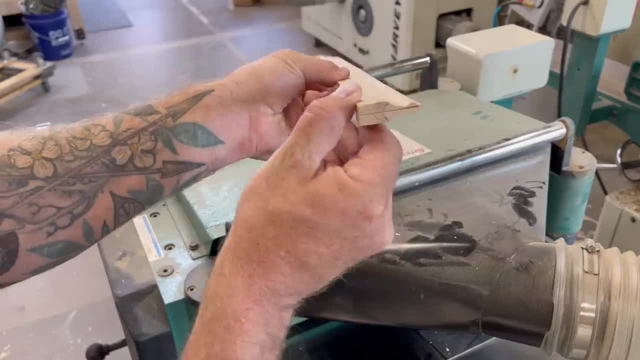 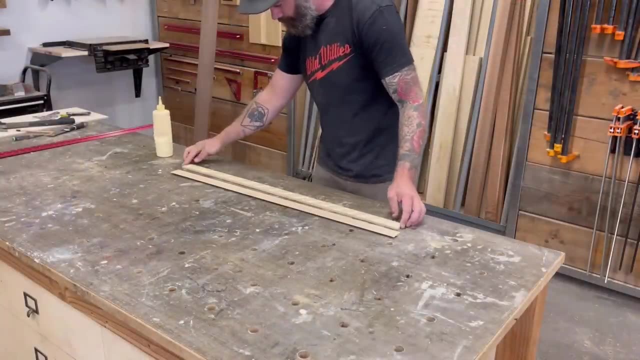 I run that through the planer until you have two identical pieces Now sandwiched together. it's really starting to look like a sword blade. All you got to do at that point is glue your two pieces together so that you have one piece that's the exact same on both sides. 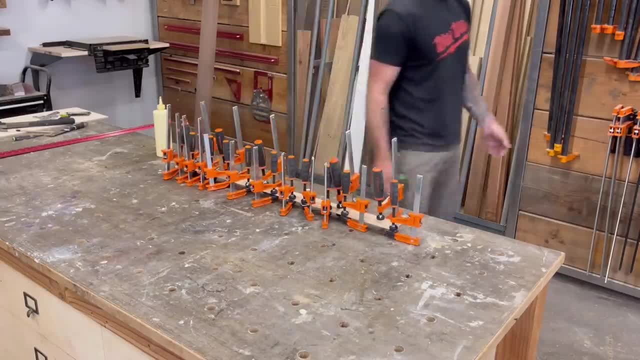 This does require a lot of clamps, but it's worth it. It's for your kid. While we wait for the glue on our sword blade to dry, we'll start working on the shield. Now for the shield. I'm just going. 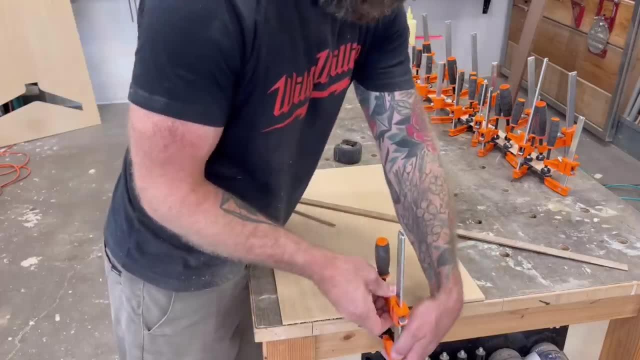 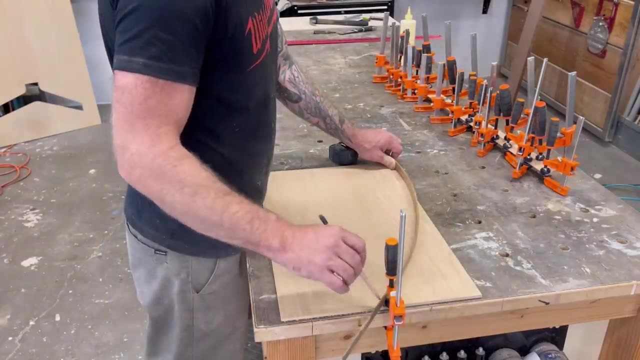 to use a scrap piece of quarter inch oak veneered plywood. I find the center and I hook a clamp on. that's kind of going to be a pivot point. Then I'm going to take a scrap piece of wood and bend it at an arc to try and trace out a shield. 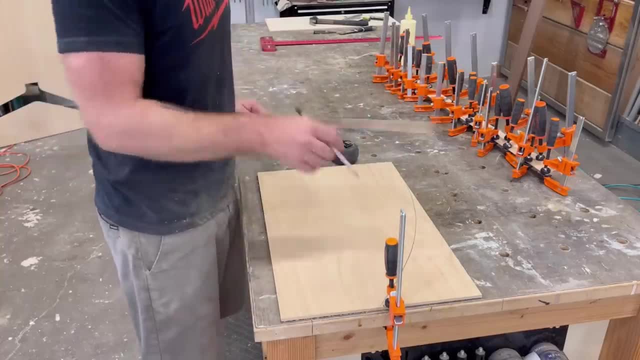 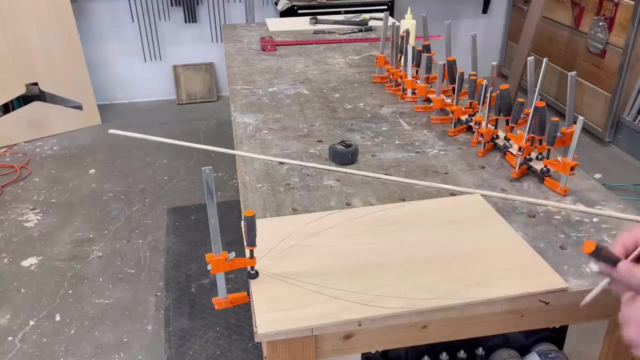 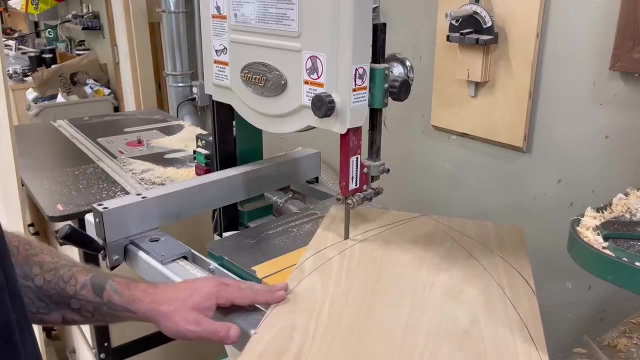 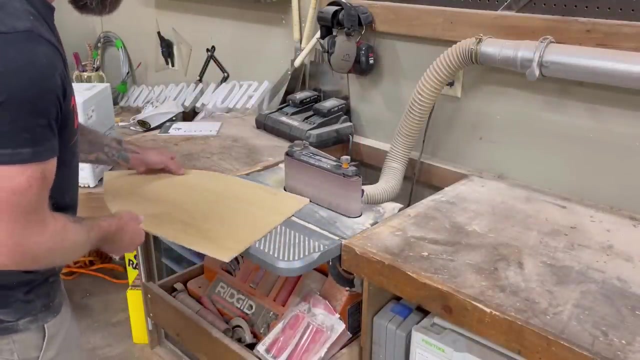 Now for this shield. I'm going to use my wiper to take a little bit of a shape. This might take a little trial and error, using different pieces of scrap wood until you get the right arc and the right shape. I mean, there's no wrong way to do this. 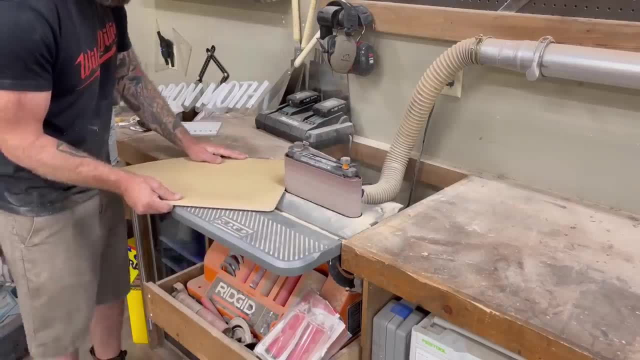 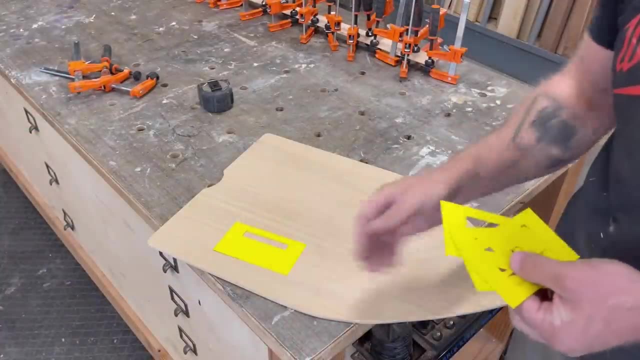 Just keep bending pieces until it looks like a shield, sanded out a little divot until, boom, we got a shield. Next, I wanted to customize this shield for my son by putting his name on it, so I just got some of these cheap paper stencils that you 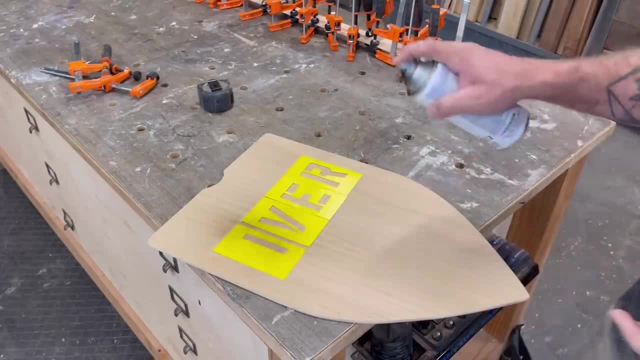 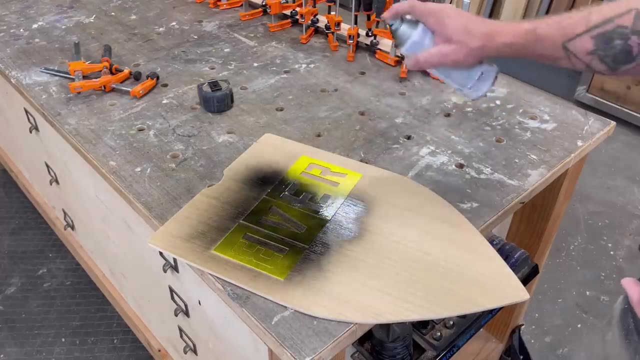 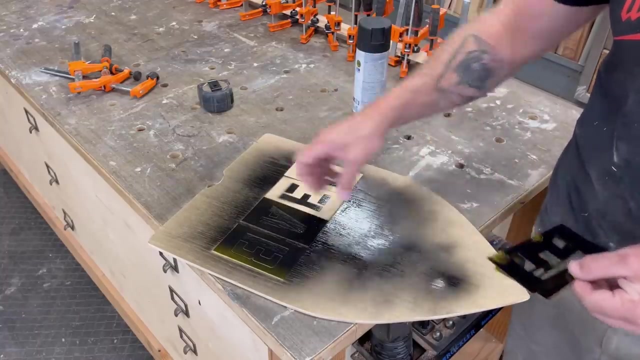 can pretty much get at any big box store, lay them out on top of the shield, and I sprayed the whole shield with a little black spray paint, kind of in an un-uniformed way, you know to give it that aged look like he just came back from some great conquest over the sea in a distant land. 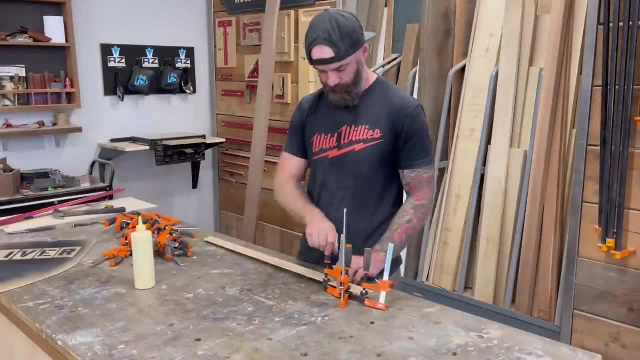 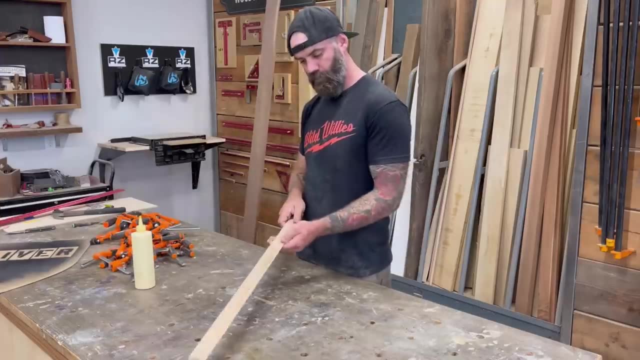 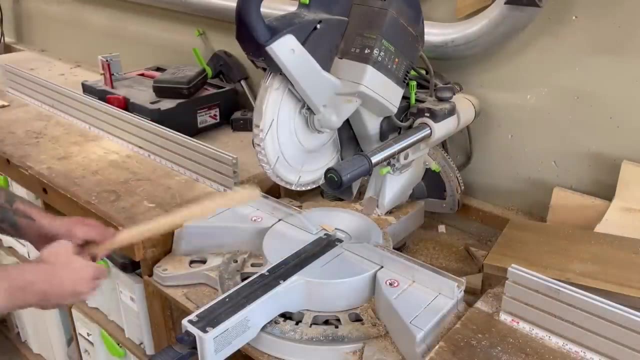 Anyways, now it says Ivor on the front of his shield. While I wait for the paint on the shield to dry, my sword blade was dry and ready to be taken out of clamps. Now we've got a sword blade, but it doesn't have any shape to it, so I took it over to my miter saw, and very carefully, so that 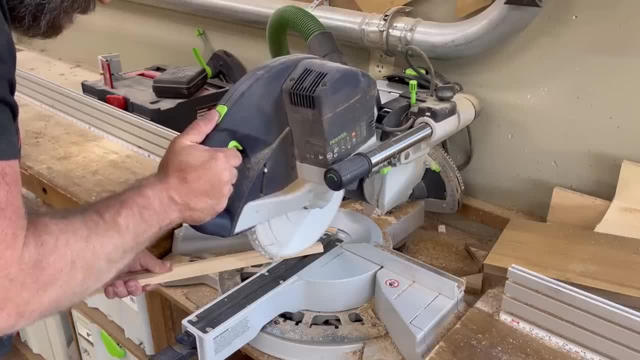 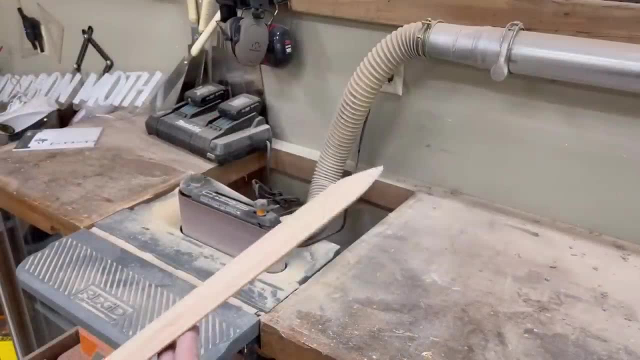 we don't do anything crazy. I added a point To one end. you could do this on the bandsaw too, and it would probably be a little safer, but this got the job done. Then, using the oscillating belt sander, I tapered the end so that it looked like. 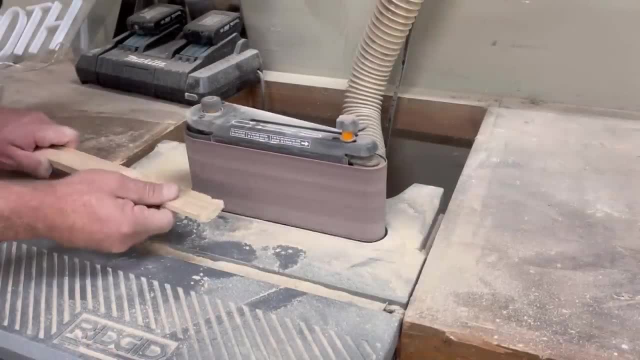 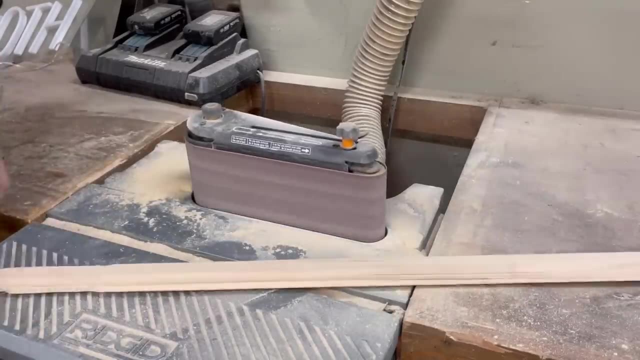 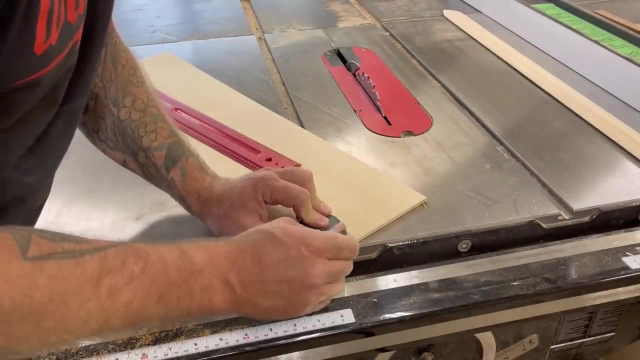 the point of a sword. Next, you have to slim down the hilt of the sword just a little bit, Not a lot. it just has to be thinner than the actual blade. so the blade becomes a stop for the guard. And speaking of the guard, that's what we're going to do next. I just get something round that. I. 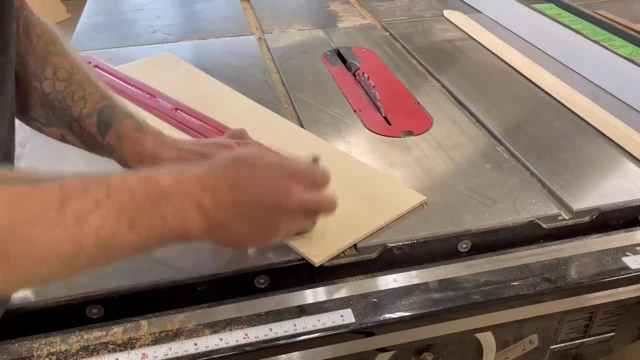 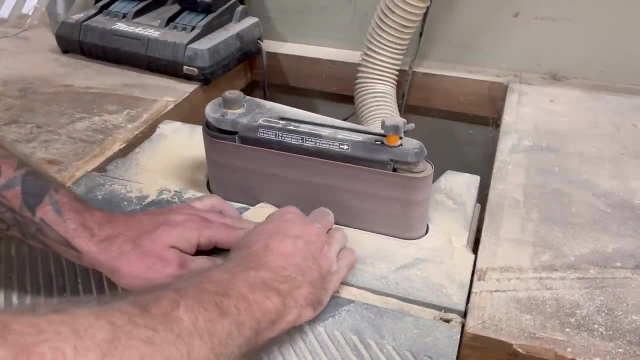 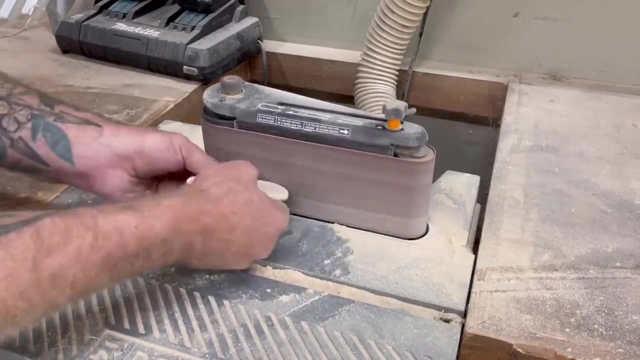 can use to trace out. and well, just kind of get a round guard like shape traced onto a piece of scrap quarter inch ply. Then, after cutting most of that shape out, I go over to the oscillating belt sander and I refine the shape, just sanding down to my pre-traced line, until we have a oval like 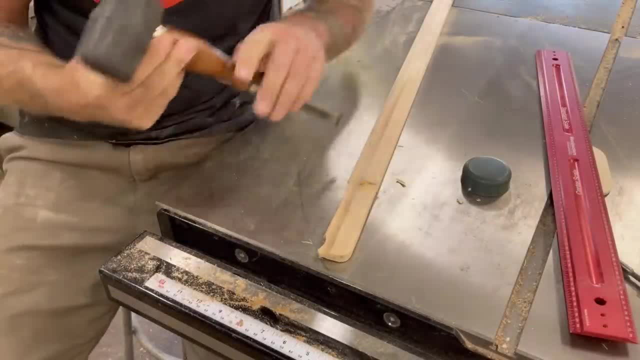 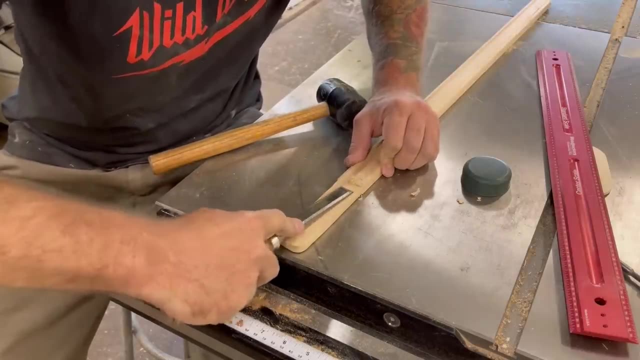 guard shape. Then I use the chisel to clean up where I stopped thinning the hilt over on the belt sander so that we have a nice hard stop and this will allow us to slide our guard on and it should stop when it hits the. 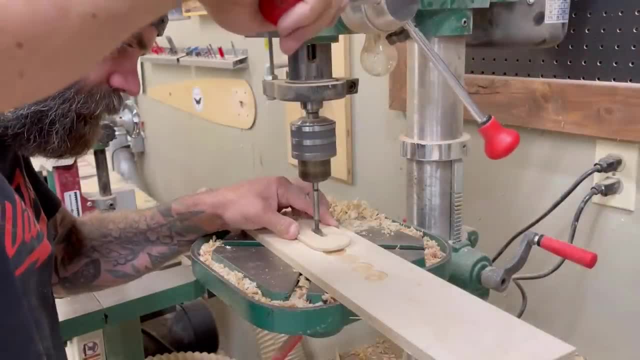 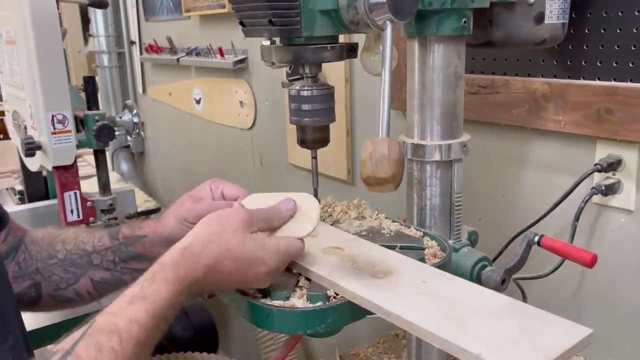 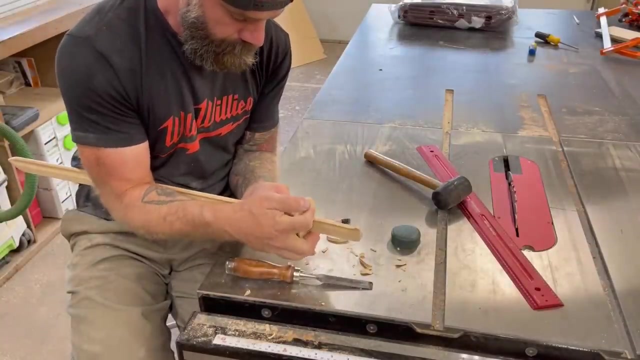 blade. Next, we need to cut a slot in our guard so that it can slide over the handle of our sword. For this I just used a little Forzner bit that was about the same size as the handle of our sword. Next we just start to slide it onto that handle, cleaning it up with the chisel as we need until. 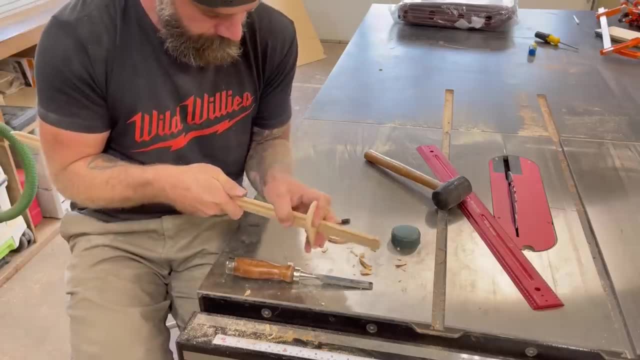 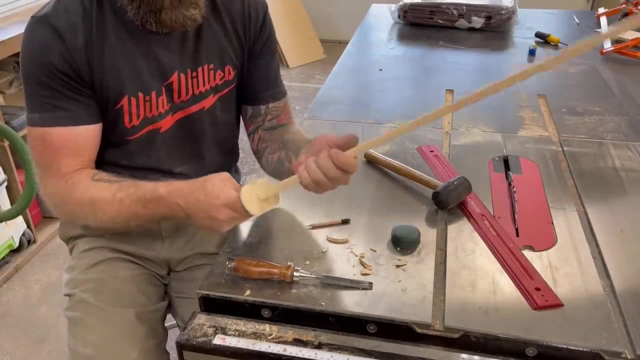 we get a nice friction fit right up to the base of the sword blade. Then we just cut a little bit of leather strapping that I had lying around. I just cut one end at a nice little wedge to get it started. I staple it in place with a half inch 18 gauge staple and then I just keep wrapping that leather all the way around the handle, working my way down to the base. And once I get down to the base I staple that part in place. 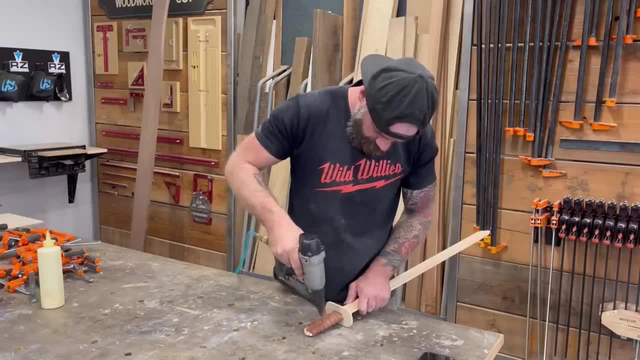 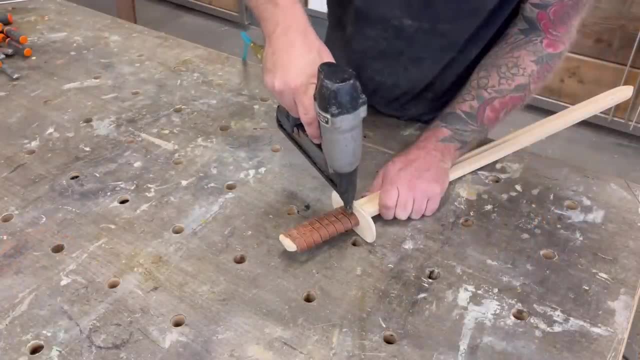 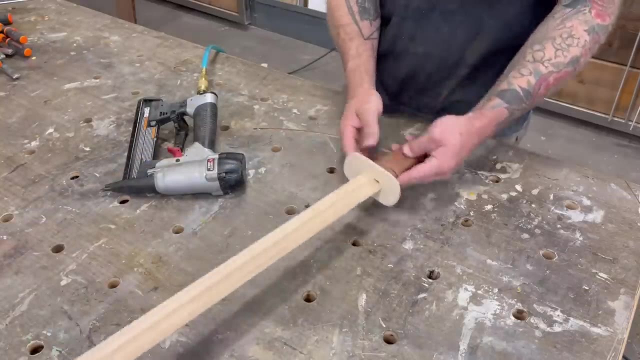 Then I run some staples all the way up the handle. These are half inch and they don't go all the way through the sword. They get stuck in there. so don't worry, you're not going to get poked. After doing one side, I do the same thing to the other side. This gives it a nice kind of riveted look. At least that's what I tell my son. 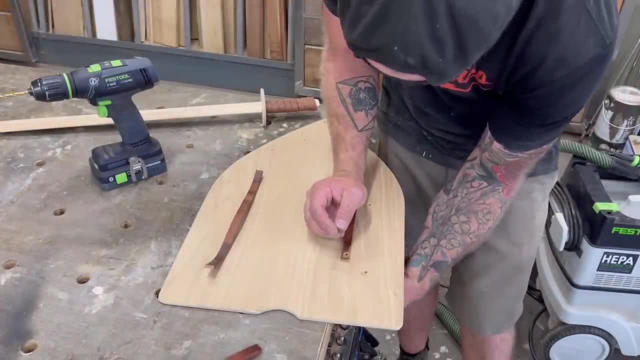 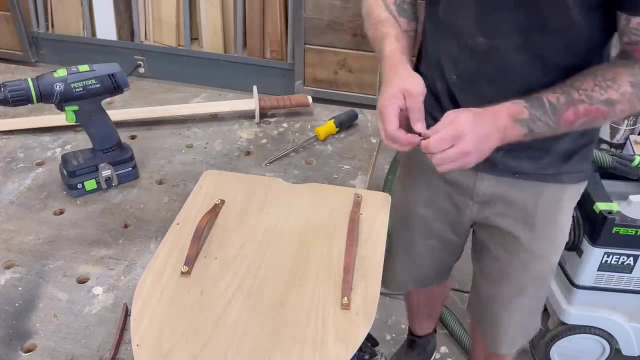 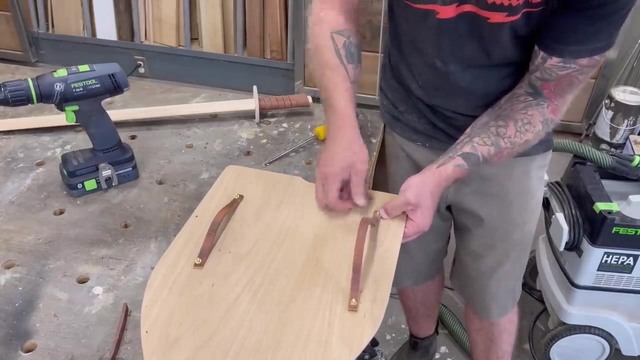 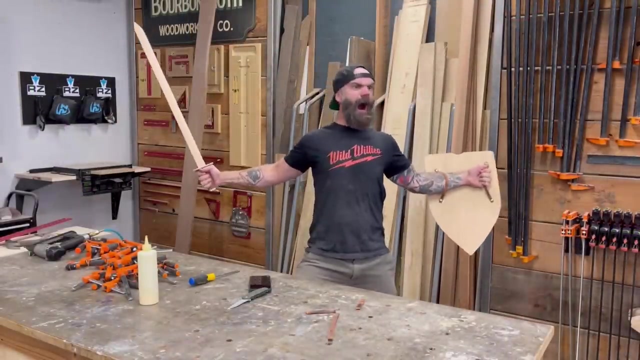 Next, we just have to add some leather straps to the back of the shield so that he can hang it on his arm when he goes into battle with the neighbor kids. I just drill some holes in it. I drill some holes through the shield and then I hook it on with these little brass screws and nuts. You could use acorn nuts, but I didn't have any, so I just used regular nuts, which means he'll probably get poked with those screws at some time and it'll be all my fault, but I just made you a sword and a shield. What more do you want? 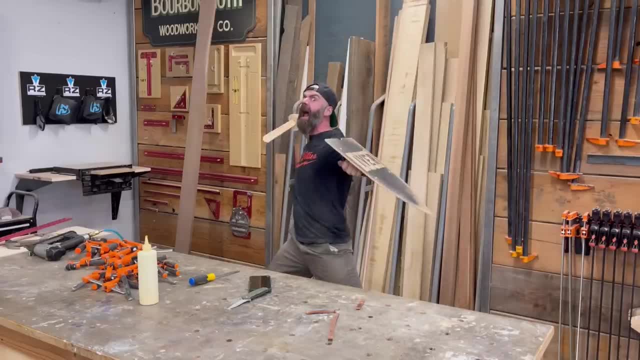 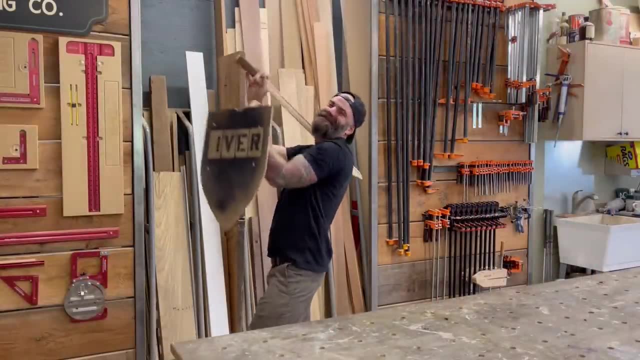 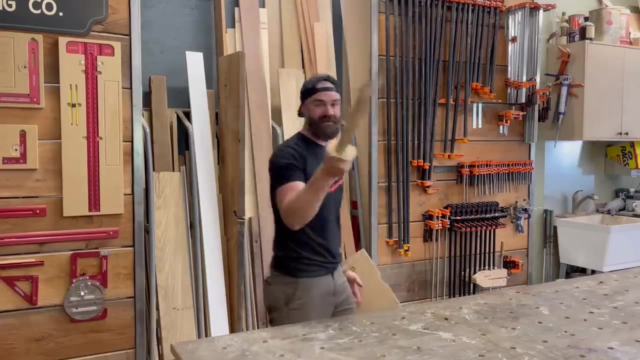 Obviously, I had to test it out and sure enough it works. It was on the back side of my head. Anyways, that's how you make a sword: Don't poke your eye out, don't kill yourself, don't slaughter the neighbors, Alright, next. 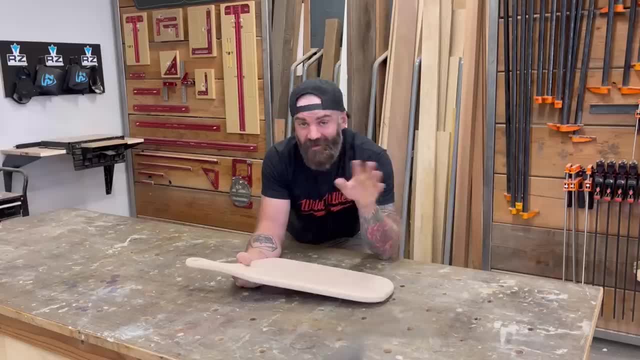 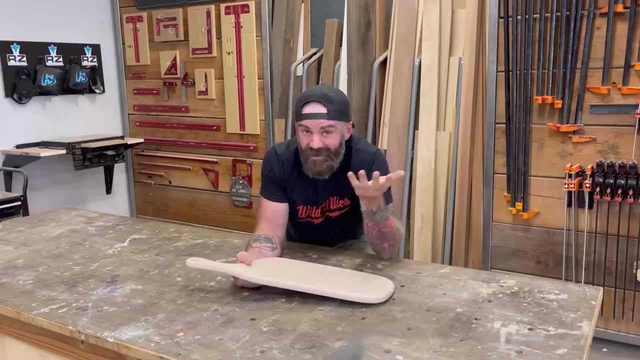 One of the most insincere and unthoughtful gifts you could ever make for somebody is a free form cutting board cut from a single piece of wood. But sometimes we're in a bind and we need a quick gift, So I thought I'd show you how. 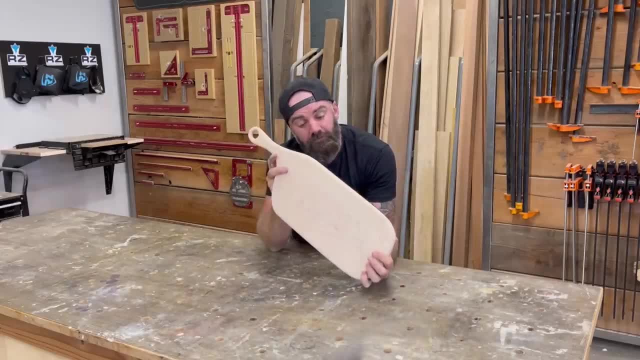 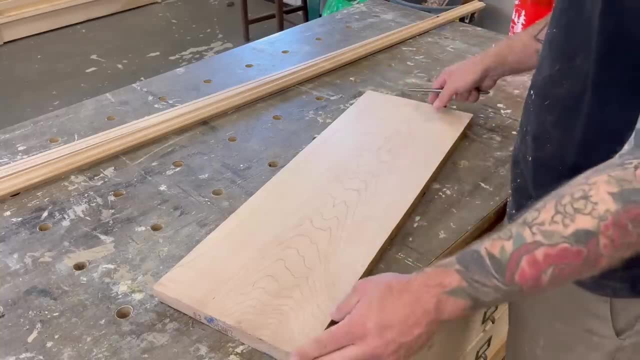 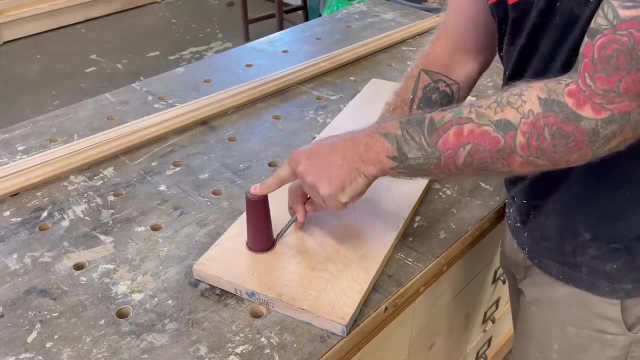 I thought I'd show you how to make one. Huh, Your wife will love it. Alright, this one's insanely easy, so pay attention. You're going to need a board, A single board that works good for a cutting board, Like maple or walnut or cherry, Something of that sort. 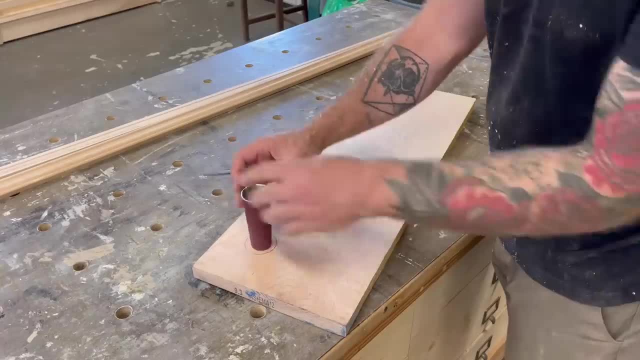 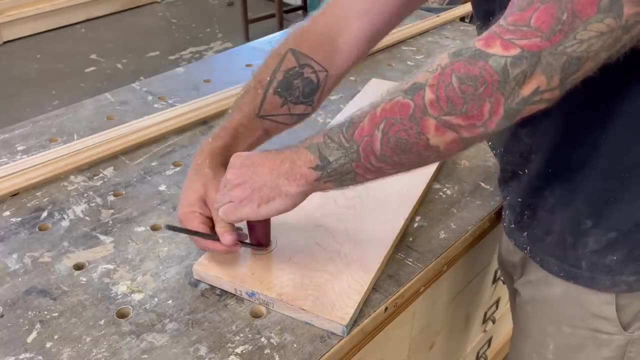 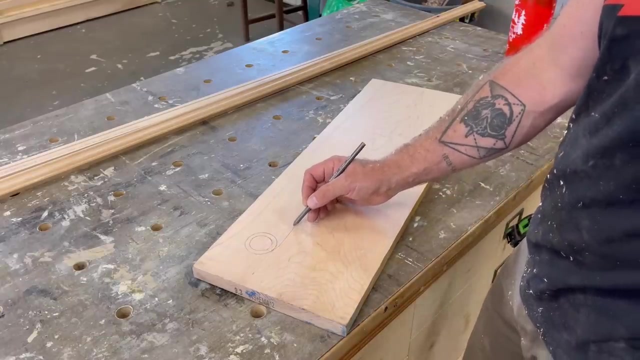 I always like to start with my handle, which is going to be round, and I'm going to drill a hole through the center. So I found this little shot glass from a bottle of bourbon And I traced out roughly where it was Beautiful. Next, you're just going to take a pencil and draw a shape. 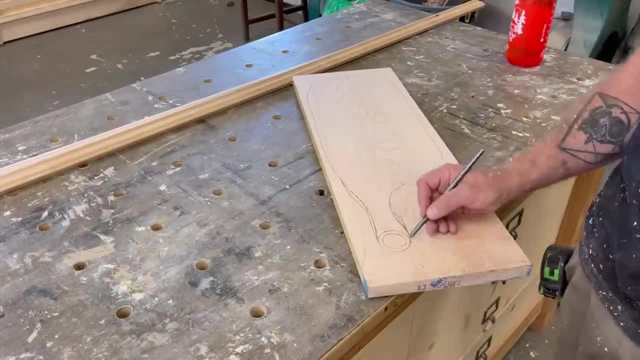 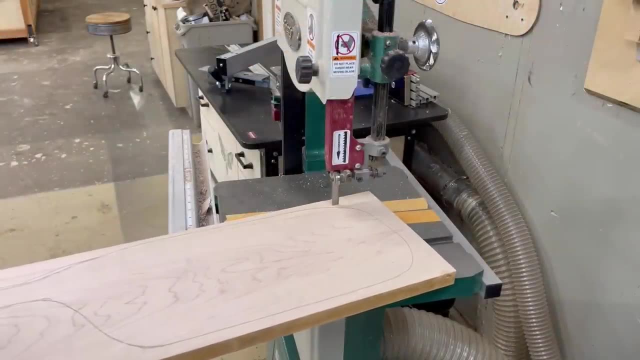 There's no wrong shapes. This is a free form cutting board. It doesn't have to be pretty, It just has to be art. That's what you tell the recipient of the gift. Once you have a shape that looks good to you, you go over to the bandsaw and you cut out that shape. 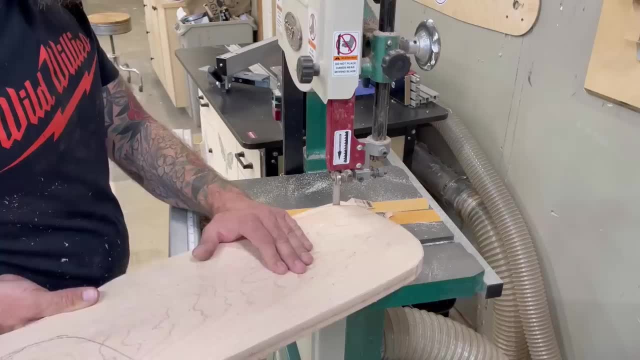 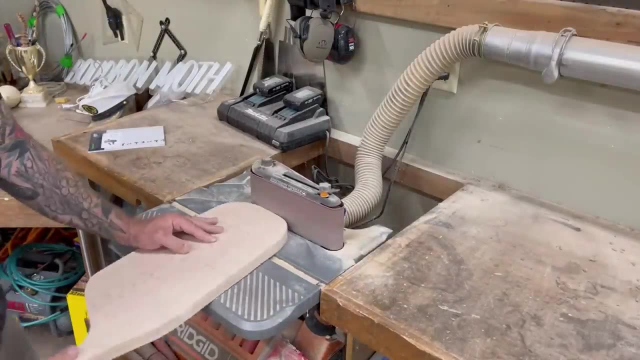 Remembering that staying on your line isn't super important. It's a free form cutting board. The lines are more of a suggestion. After you cut it out on the bandsaw, I like to clean it up over on the oscillating belt, sander. 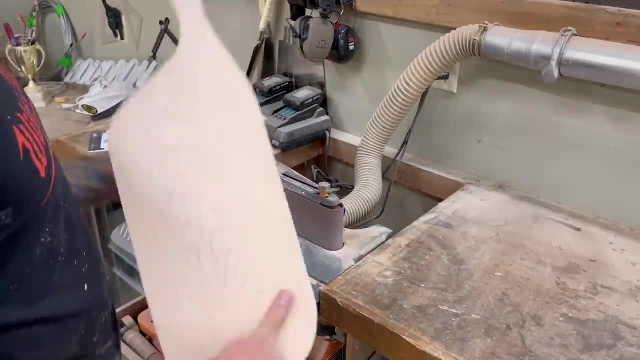 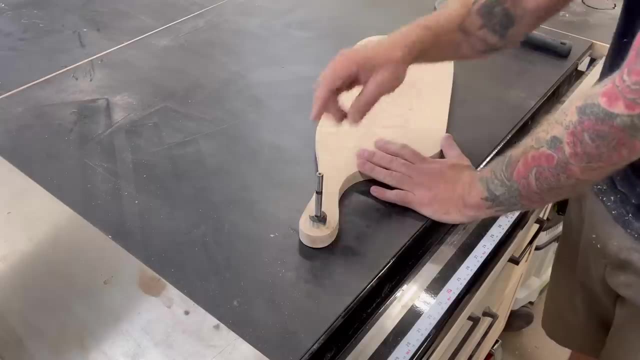 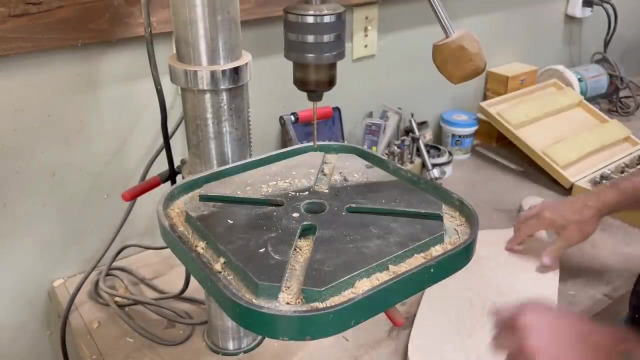 Which is being used a lot in this handmade gift video. After we get all the edges cleaned up, nice and they're looking smooth, I take a Forzner bit that looks like a good size to drill out a hole in my handle. I tap it in with a hammer to get it started and then, using a smaller drill bit, I drill all the way through the cutting board. 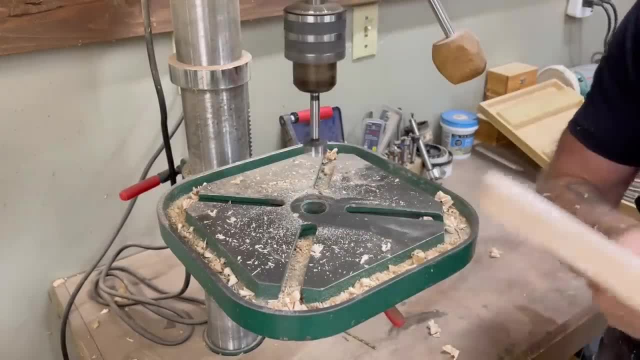 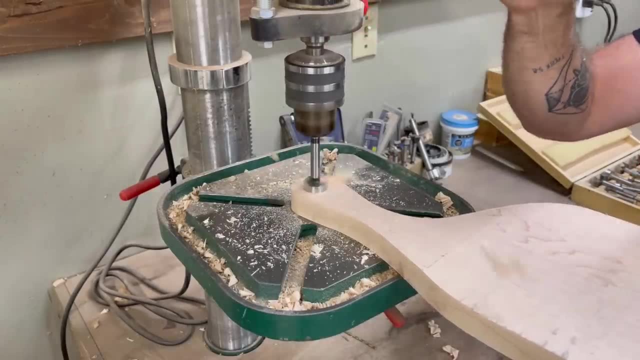 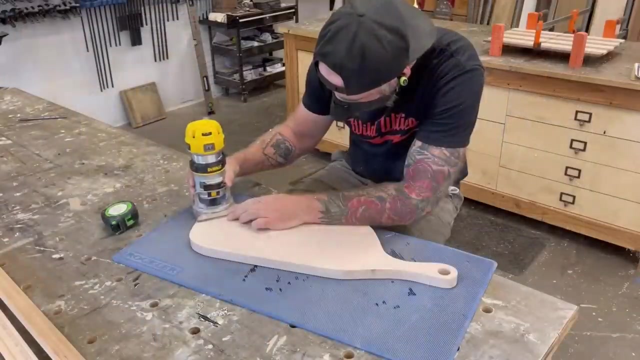 This will allow us to drill in from both sides, with the Forzner bit Making sure it's lined up and we're not going to get any blowout on one side. I mean, we still want the cutting board to look nice. After we drill the hole, I take it over to the drum sander and I send it through on both sides to get it nice and smooth. 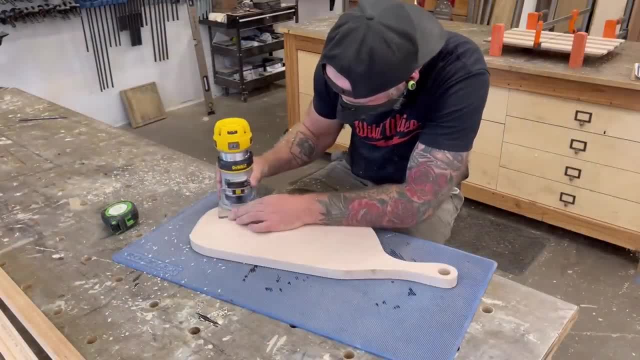 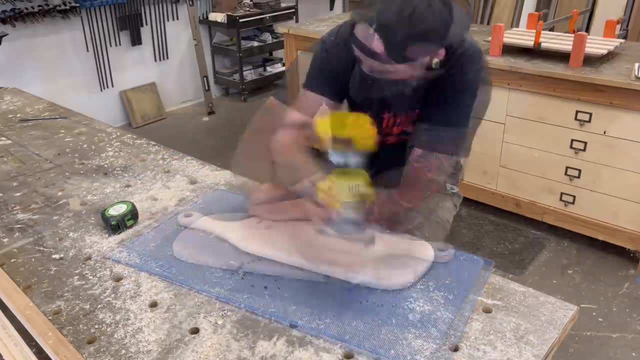 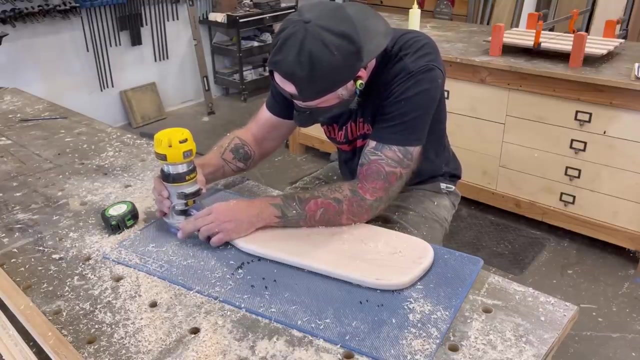 And then I pull out a quarter inch round over bit and I start rounding over all of the edges To make it look like I put more effort into this than I actually did. I also rounded over the inside of the hole I drilled out To make it feel nice on your finger. 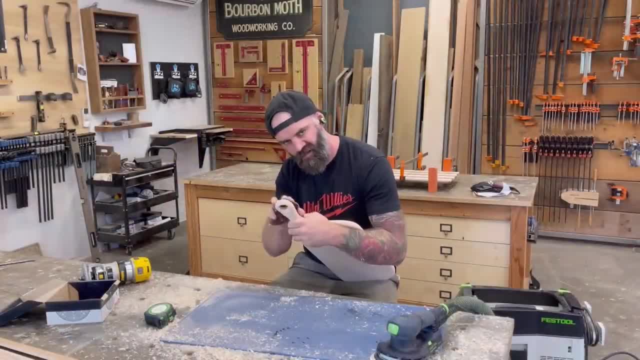 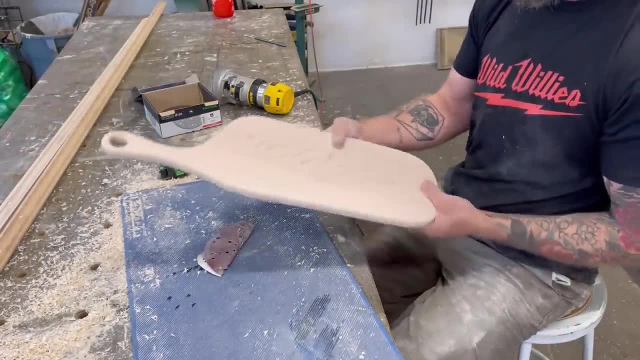 After everything is thoroughly rounded over, you sand, And I hate the sanding part, But in no time. look at that- A free form cutting board made in about 10 minutes. Just tell the person who's getting it. it took all day. 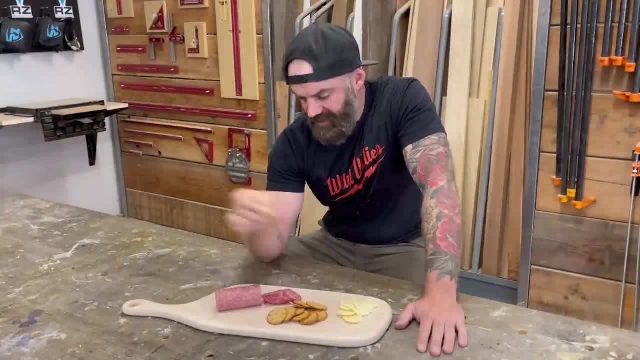 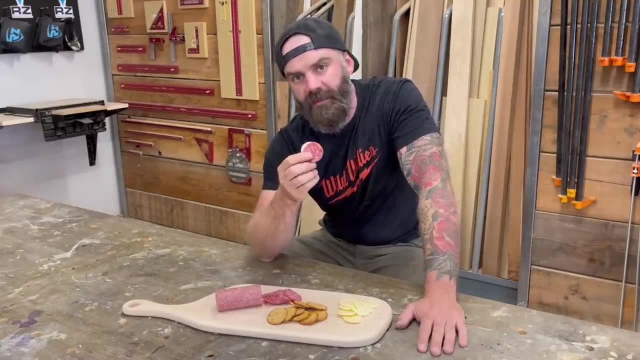 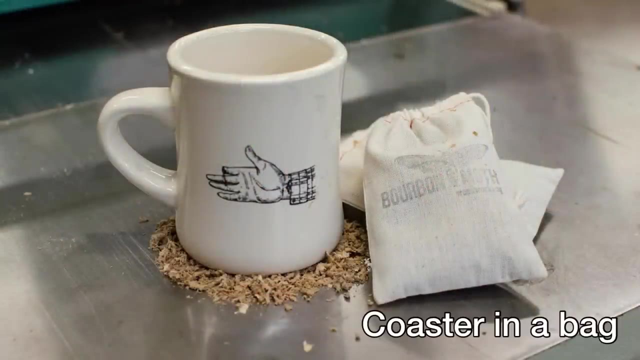 Well, I try and do something nice for my wife. Make her a 10 minute cutting board from the sincerity of my own heart, And what happens? She gives it back to me. and now I'm out here eating all by myself As woodworkers. what's our number one pet peeve? 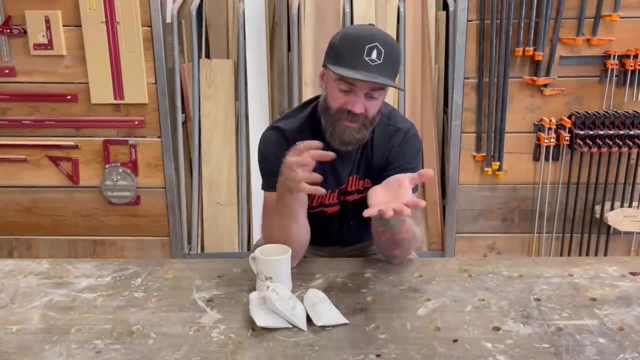 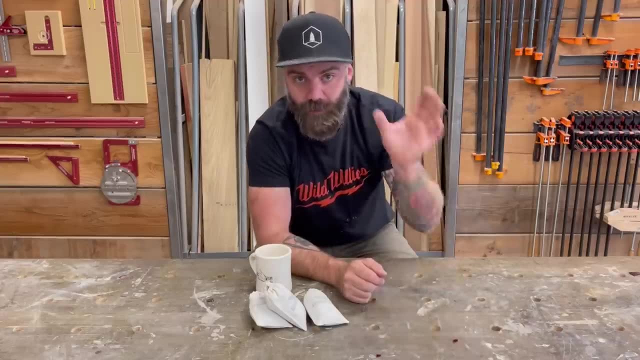 People who only pop the popcorn halfway through and you got a bunch of unpopped kernels in there. It's annoying, But what's our number two pet peeve? Yeah, people putting drinks on top of our brand new, freshly made furniture without a coaster. 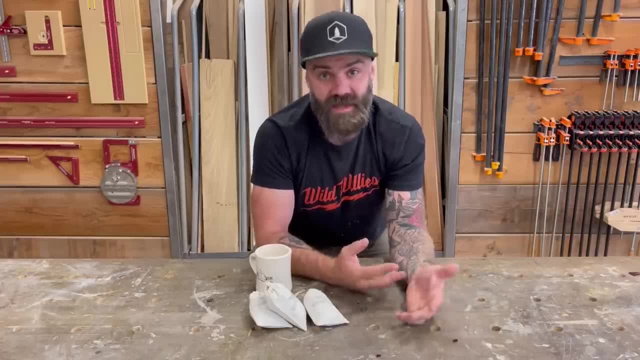 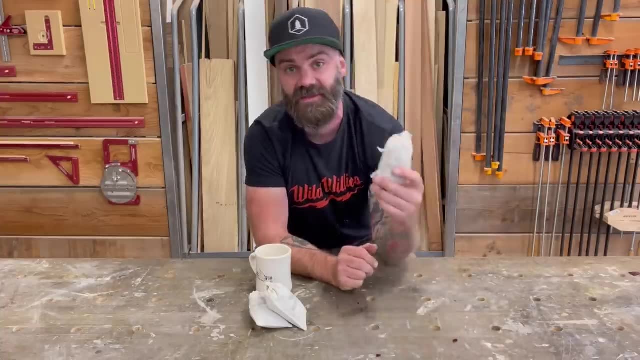 But coasters can be. ugly Coasters can be hard to find. Some houses don't even have coasters. That's why this is a great gift for your friends, family members and clients, And that is coaster in a bag. Regular coasters are inherently flawed. 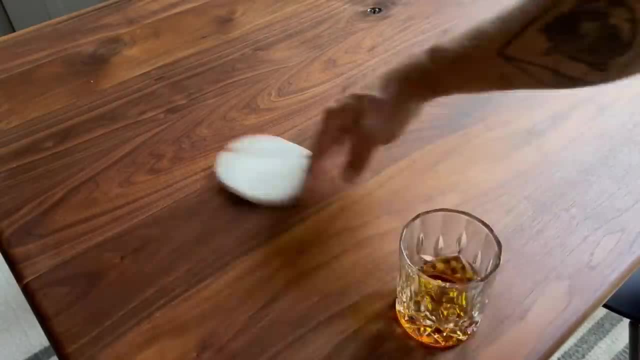 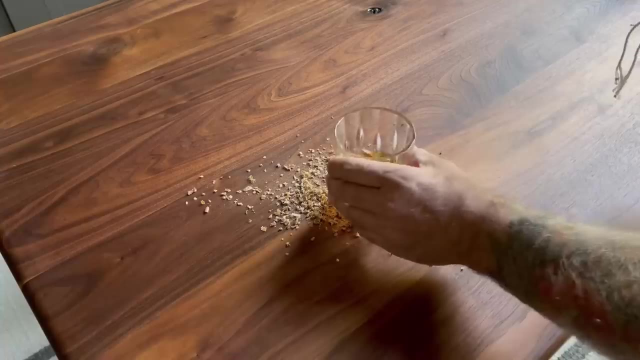 Because once you set the drink down, it can sweat and still roll onto your piece of furniture. Introducing coaster in a bag, You simply pour out the contents of the bag and set your drink on them. Not only does it protect your table, but the contents will soak up any unwanted moisture. 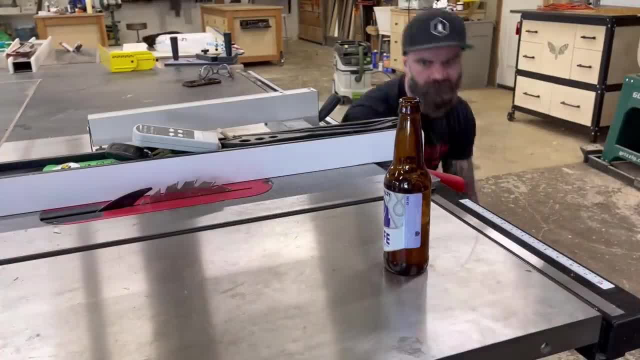 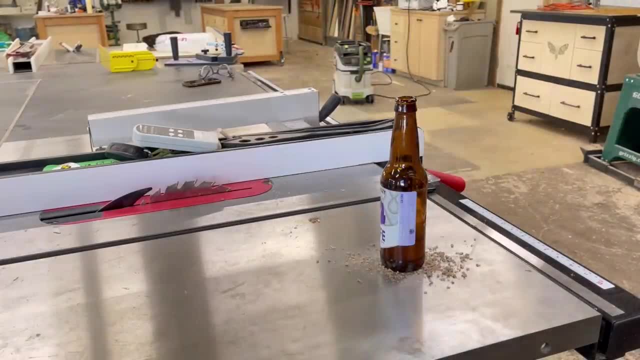 Do you have annoying employees who just set their drinks on your cast iron work surfaces? Well, coaster in a bag is here to help you save the day and your equipment. Yo Jason, I need one of those coasters in a bag, Thanks. 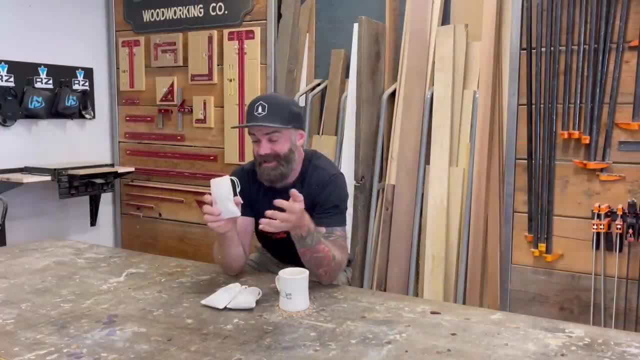 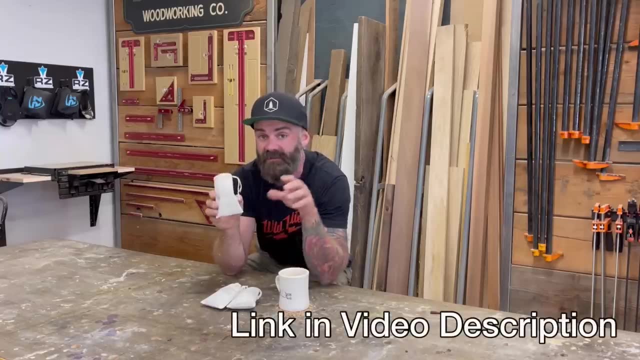 I'm telling you guys, coaster in a bag is a great gift and it's easy to make. But if you don't want to hassle with making it yourself, these are actually going to be available for sale on our website: $12.99 for one coaster in a bag or $26.50 for two. 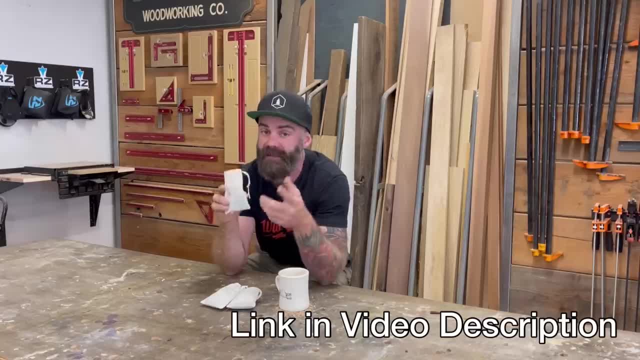 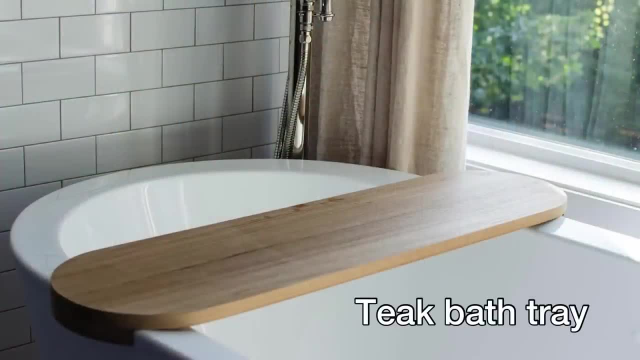 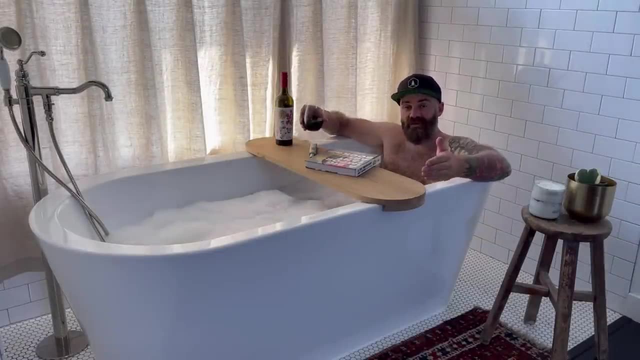 There's a link in the video description. Get yours today. Only available while supplies last. Another great gift for that special someone in your life is a custom wooden bath tray. It's a little tray that sits across your bathtub and holds all your fancy accoutrements. 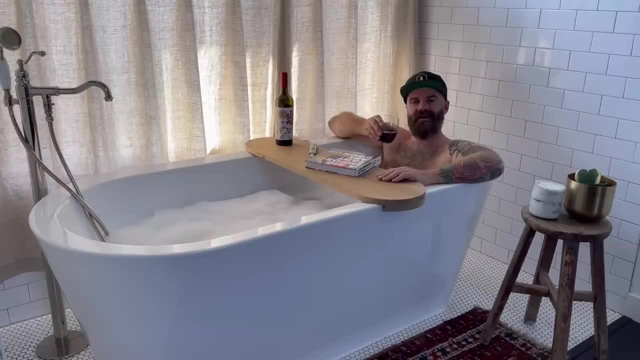 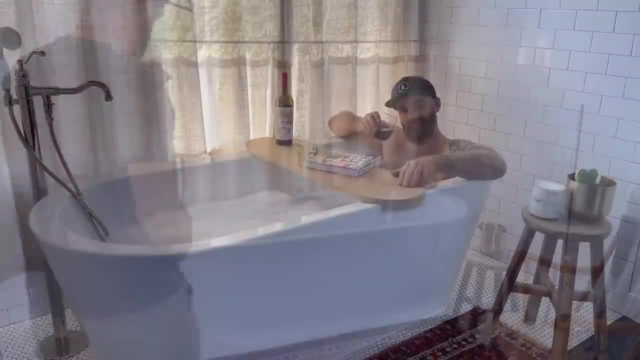 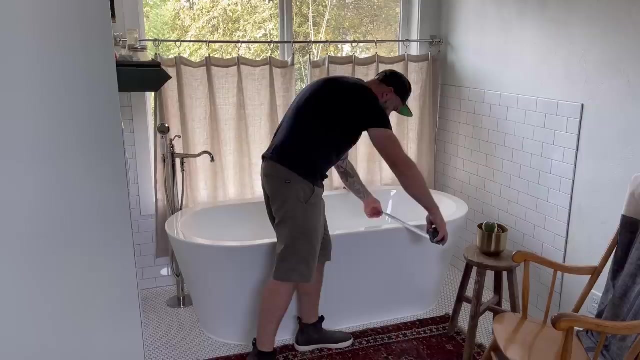 Things that really enhance your business, Make it a bath time ritual, Make it something special, Make it something to remember. I'm going to show you how to make this one right now. Now, everybody's bathtub is different, So the first thing you want to do is measure your bathtub or the bathtub of the person who will be receiving this gift. 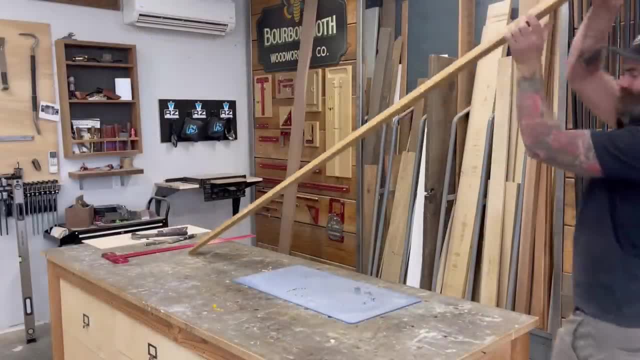 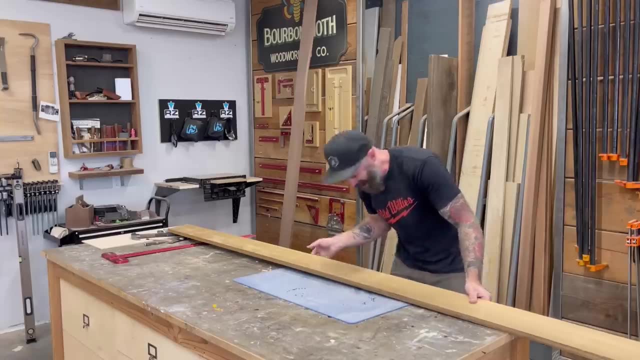 Once you get the measurements right. next you got to select the wood. Now for this tray, I'm using teak, because teak does great with moisture. It's got a very high oil content. People actually use it to build furniture for inside of showers. 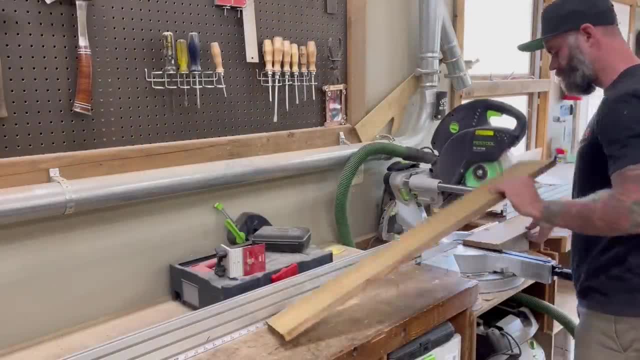 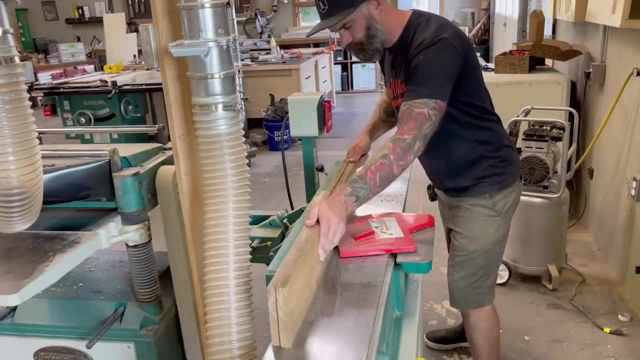 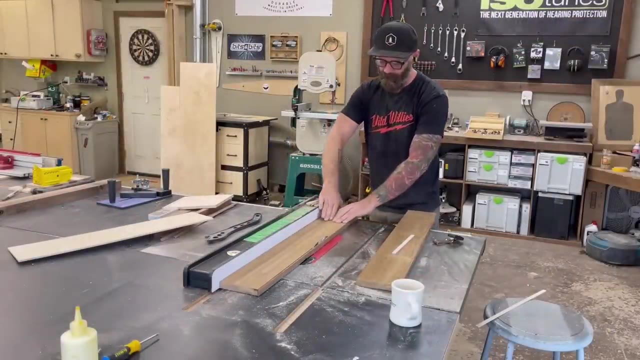 Because apparently that's a thing now: Furniture and showers. Anyways, with your measurements in hand, you need to cut your boards down to the right length. Next, you need to join one side of both boards so you have a straight edge that will allow you to run it through the table saw and cut it down to the correct width. 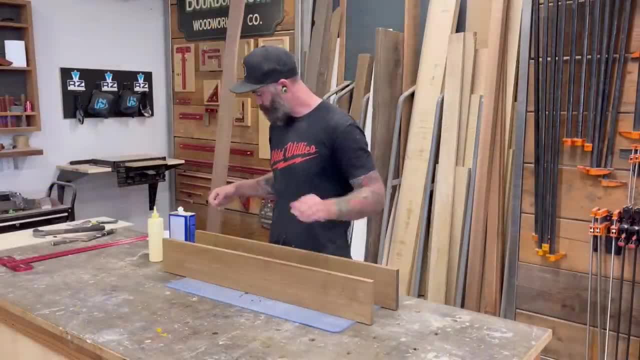 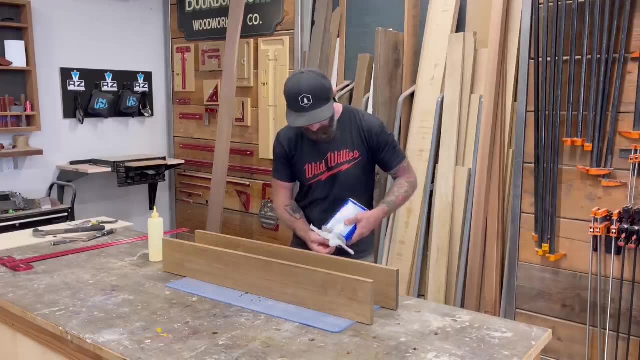 And the correct width is whatever the heck you want it to be. Now, one thing to note about gluing teak to itself Is that the oil content is so high that, before you glue two boards together, you really need to wipe down that glue joint with a little acetone. 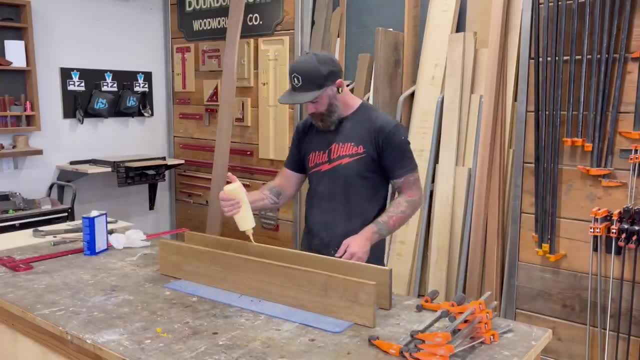 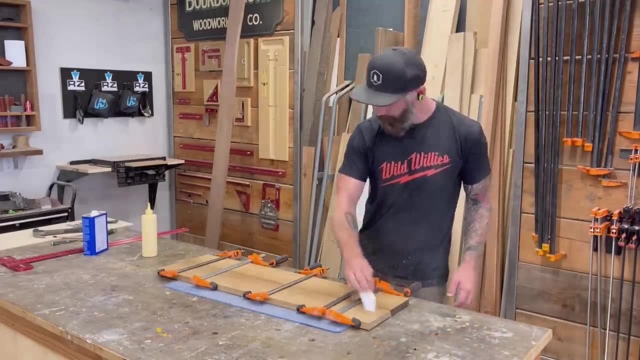 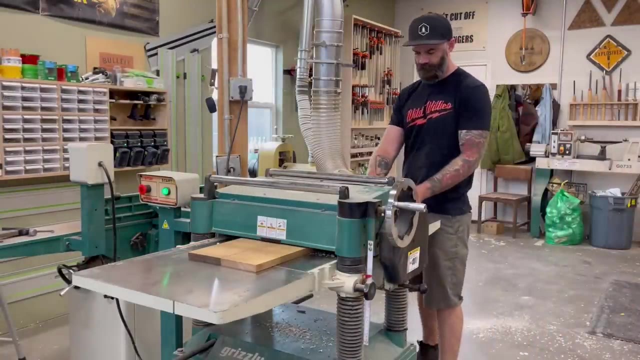 This will remove any surface oil that's sitting on the wood and will allow that glue to penetrate in and actually hold the boards together. So after doing that, I clamped the boards up and waited for the glue to dry. Once the glue was dry, took it out of clamps and I sent it through the planer on both sides to make sure the top and bottom were dry. 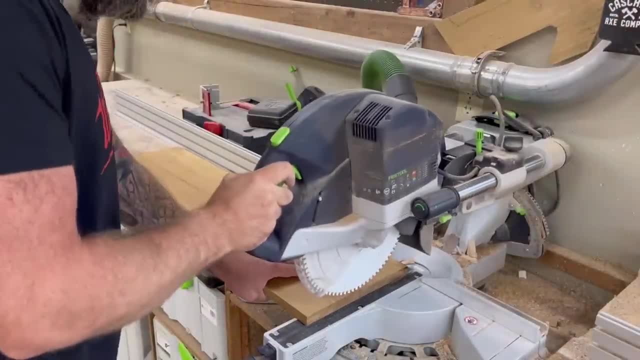 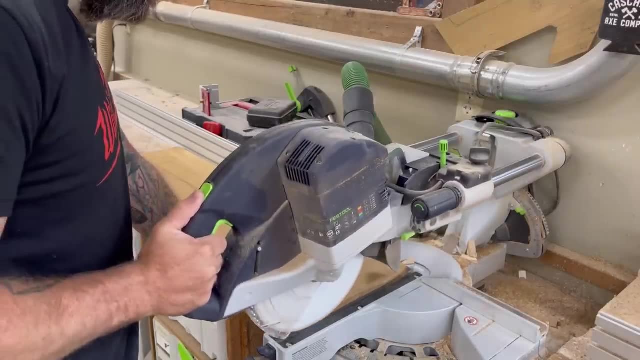 The bottom was nice and smooth. Then I went over to the chop saw and I just cut a tiny little bit off each end to make sure that both sides were perfectly square. Next you want to take your boards, set it on your workbench and grab a big bucket full of junk. 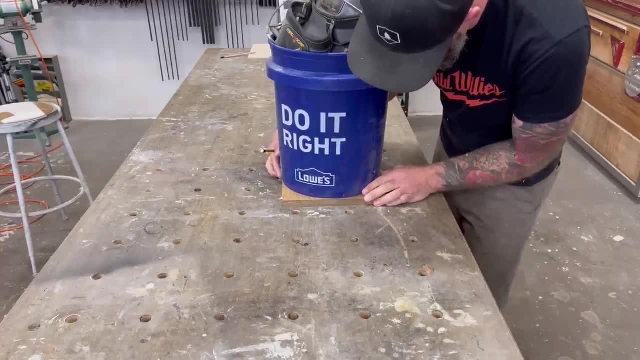 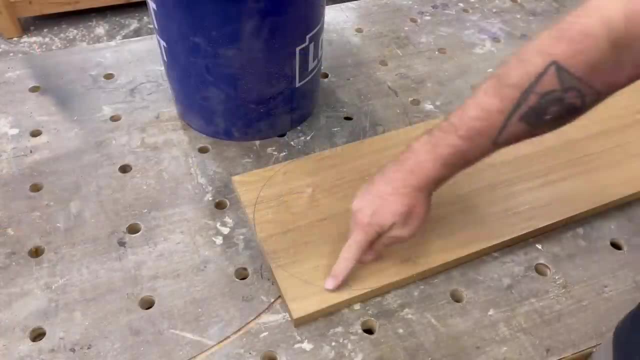 And set it on top. I mean, I guess it doesn't have to be a bucket, just anything big and round. The bucket just happened to be the exact right size to get the profile we wanted, Which was this nice round profile on either side. 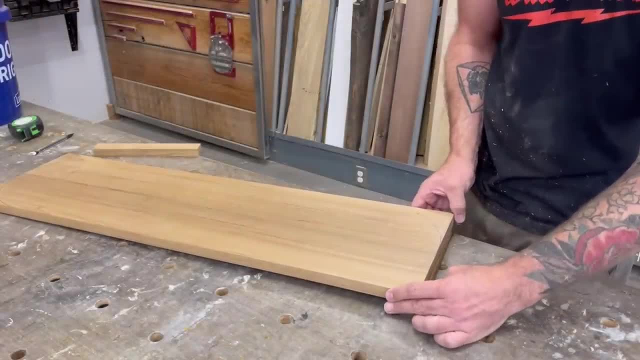 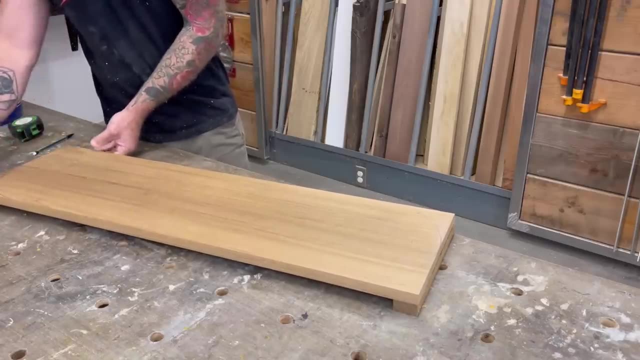 So I used the bucket to trace out that profile on both ends. Next, we need to attach some feet. These are less feet and more guards. These are what's going to keep the tray from sliding to one side or the other and falling into the bathtub. 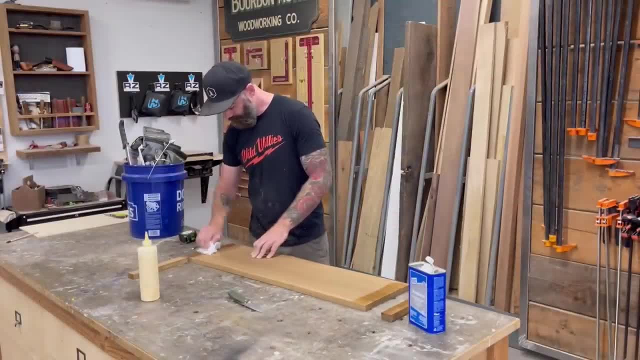 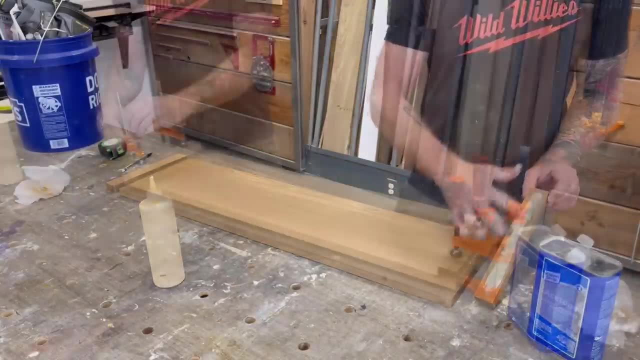 And just like our other glue seam, before we glue these feet onto the bottom, we wiped down each seam with some acetone to get rid of that surface oil. Spread on some Titebond 3 because it's good for moisture And we clamped the entire thing. 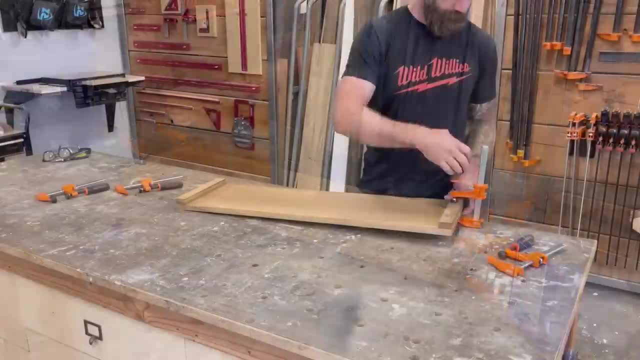 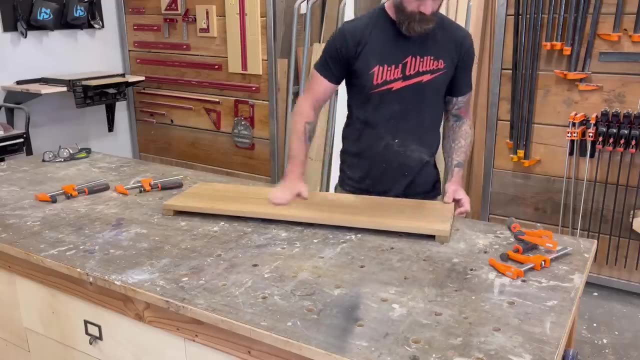 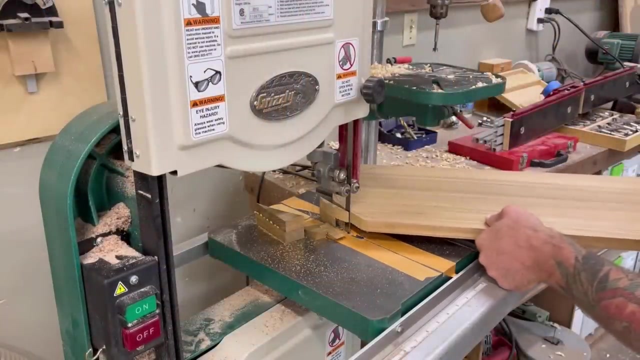 Then we just had to wait for our glue to dry. Ooh, our glue's dry. Look at that With our feet glued on. now it was time to cut that rounded profile shape. So I went over to the bandsaw and I cut off most of the material staying just outside of my pencil line. 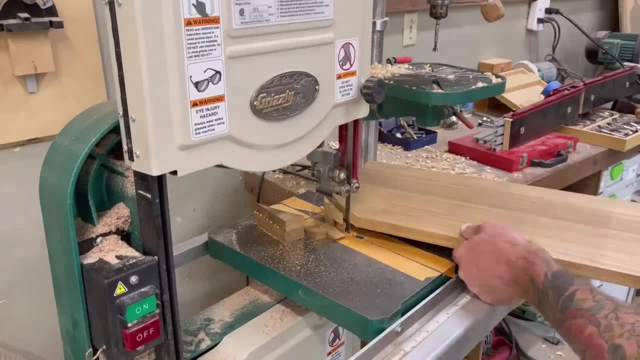 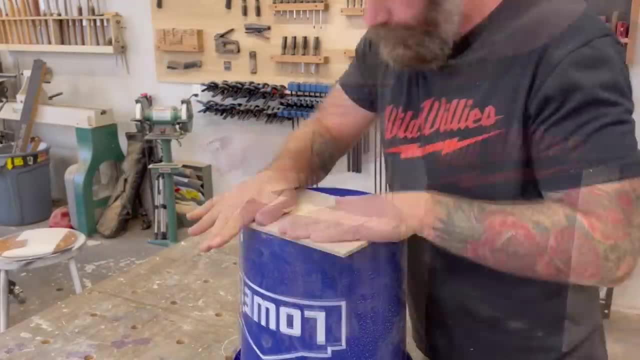 Once I had enough material removed, it was time to use the router. But for this we needed a router template And unfortunately I thought the bucket would be a little awkward to use as a router, So I cut it off. So I'm going to use the bucket to make a template. 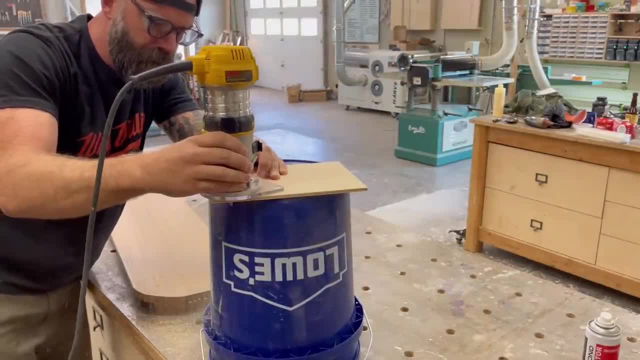 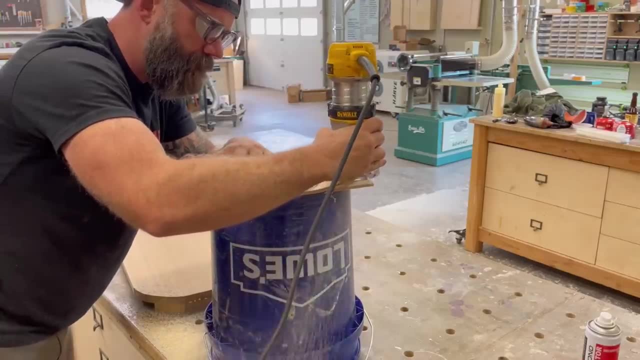 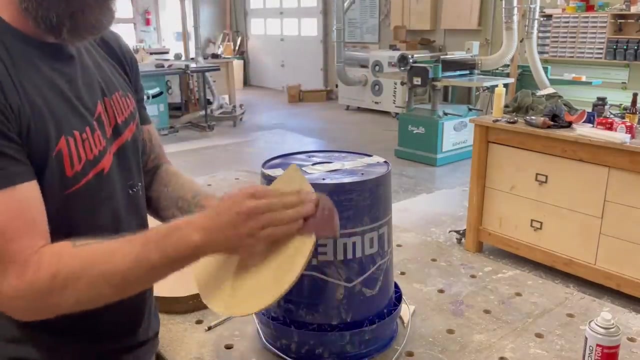 So I CA glued a piece of quarter-inch plywood onto the bottom of the bucket And using a quarter-inch flush trim bit from Bits and Bits I just made a template real quick out of that quarter-inch plywood. After that was cut out I just pried it off the bottom of the bucket. 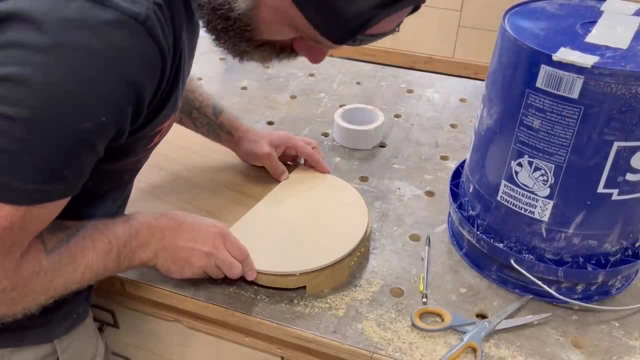 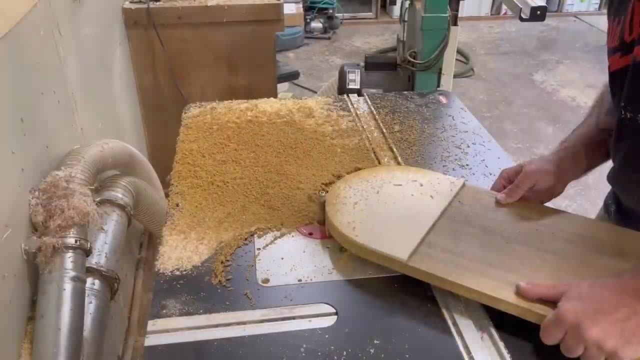 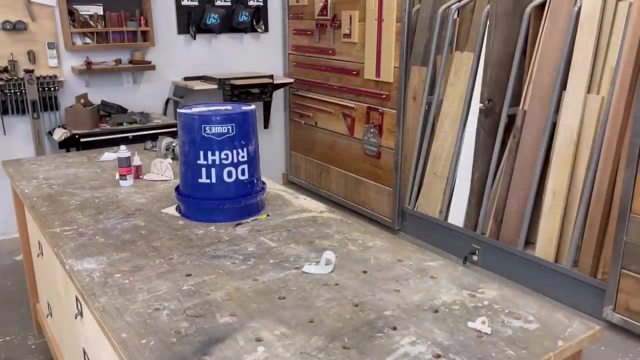 And used some double-sided tape to stick it to the top of my template And stick it to the top of my teak bathtub tray shelf thing. Then I went over to the router table And again using this flush cut compression bit from Bits and Bits. I flush trimmed both the ends to match my template. 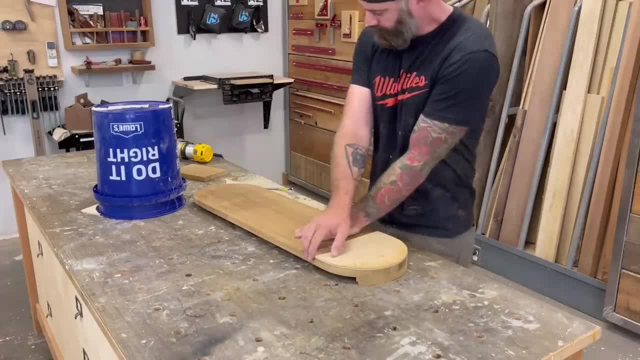 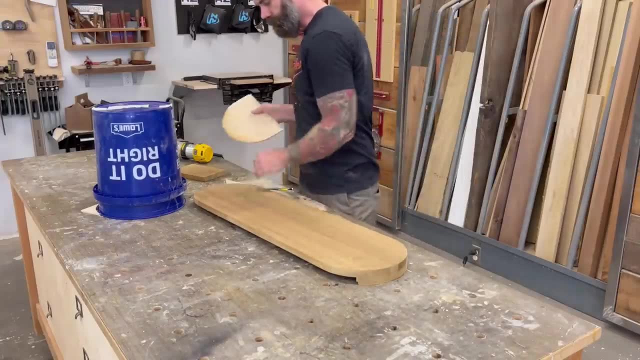 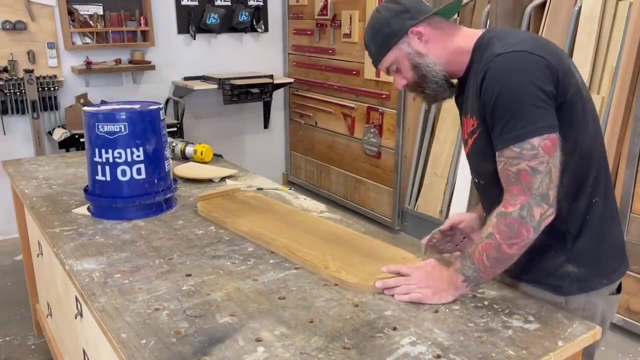 And look at that, We have this nice rounded looking bathroom tray shelf thing. All that was left to do was to clean it up a little bit with some hand sanding And this thing would be ready to install, And by install I mean ready to set on top of the bathtub. 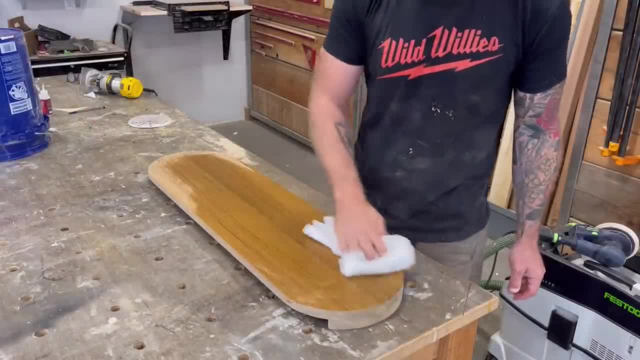 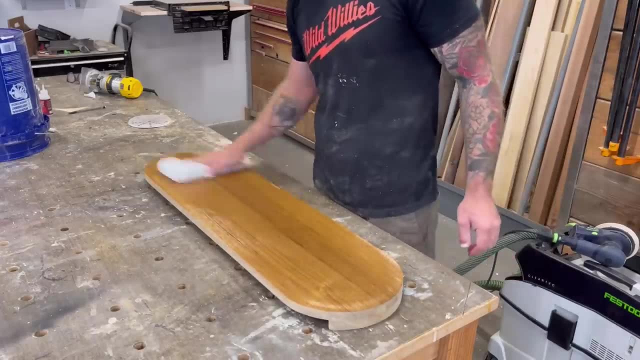 I did wipe the whole thing down with a little more acetone just to get rid of all the dust and get rid of any surface oil that might be sitting on the outside of the teak, And I was ready to take a bath. Man, this is great. 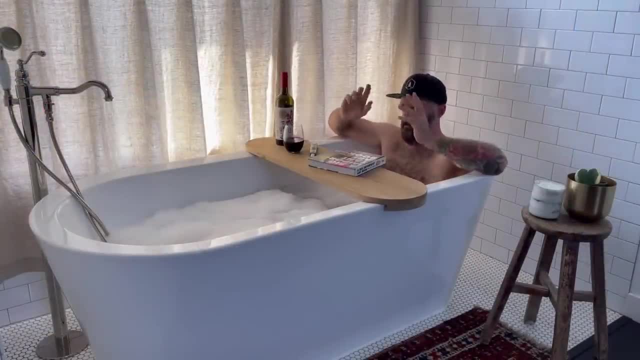 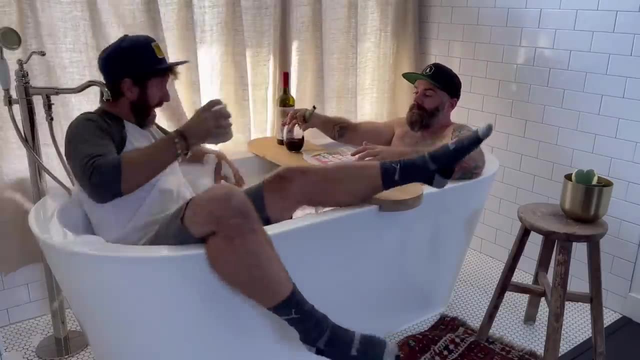 I got my wine here. I got a good book I can dive into. The only thing I need is a nice scented cane little just to make the mood. Jason, no, no, no, no, no. Are you crazy? Hey man. 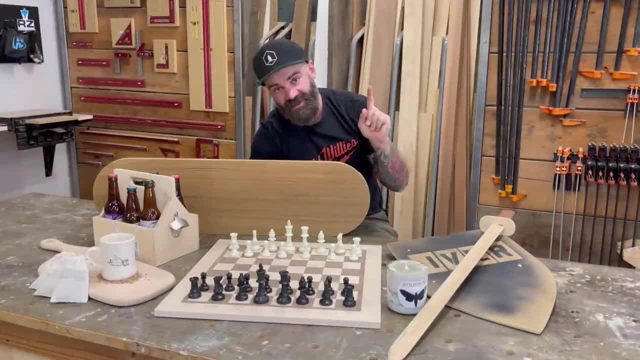 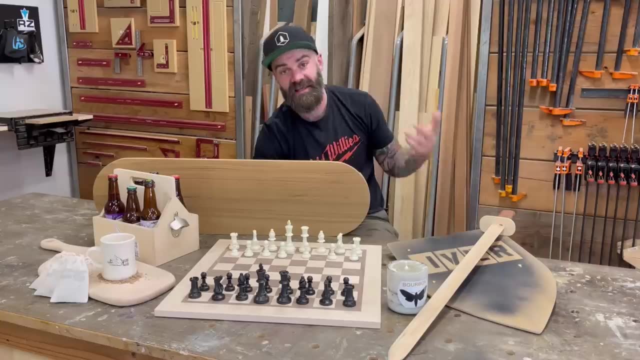 All right, There's still one gift that I haven't mentioned yet, And I saved the best for last. If you're too lazy and can't find the motivation within yourself to get up off the couch and go make something for your significant other, 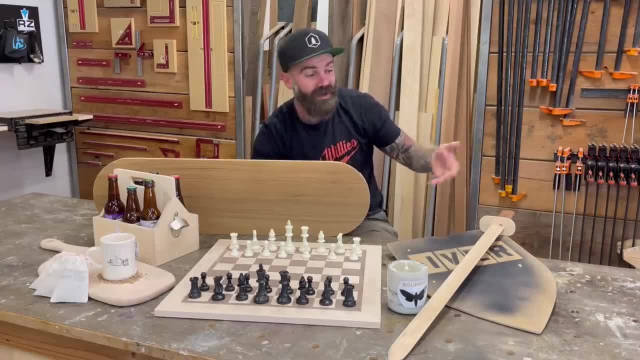 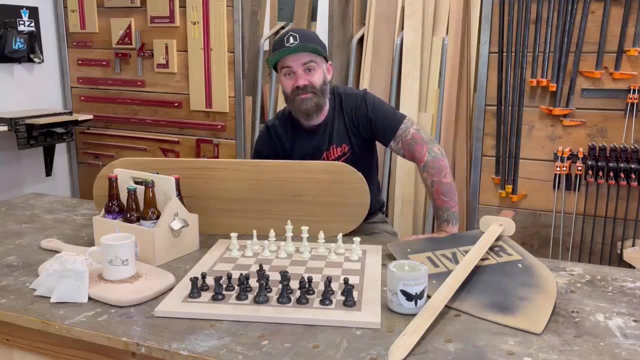 well, that's okay, You can just get on our website. We've got a whole bunch of new merchandise: T-shirts, hats, coffee mugs, that sort of thing. There's a link in the video description. Just do that. 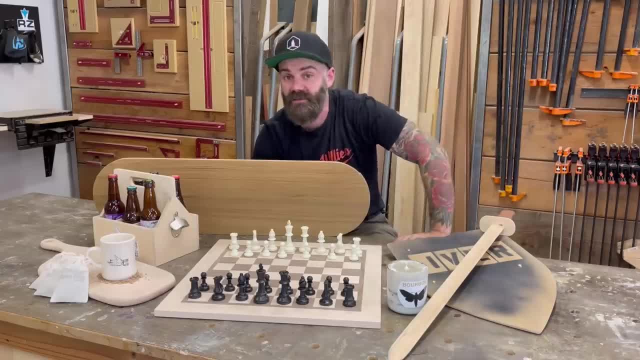 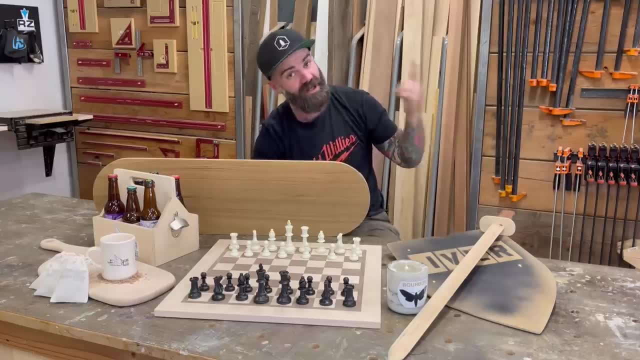 Or go in the woodshop and build something. Hopefully, you got some good ideas from this video. There's also links to all the products and tools. we used a link to our Patreon page down there. If you're not signed up for Patreon, you should be, because you get a whole bunch of behind-the-scenes footage, backstage pass perks, live question and answer every week. 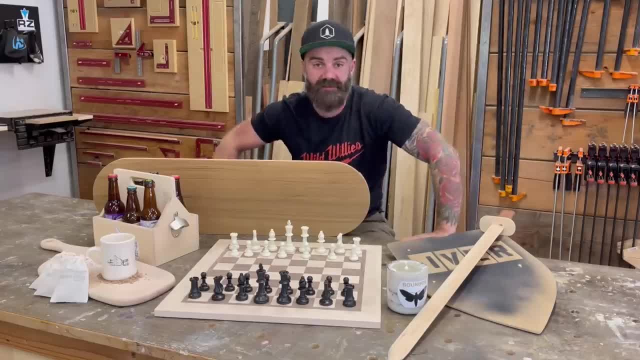 Disclaimer, Discount codes, All sorts of things. So until next time, go make a gift and use a coaster.